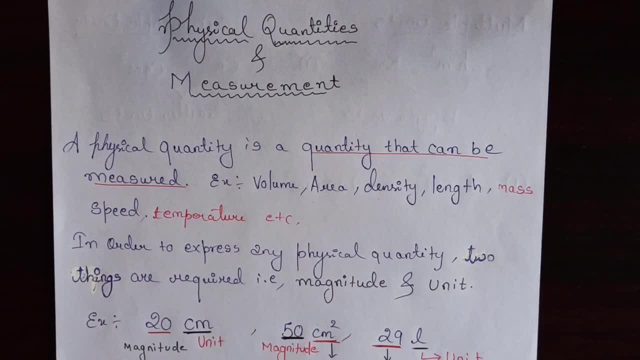 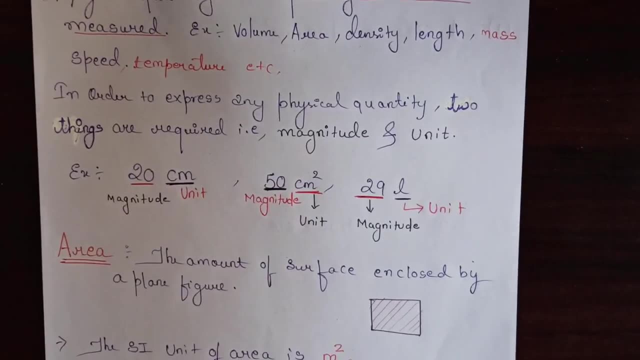 So in this chapter we will sow the number of meters we can measure versus, say, in data itung. So basically, first of all we cannot go into much detail because it is in class 6, so you know a lot well from the beginning. 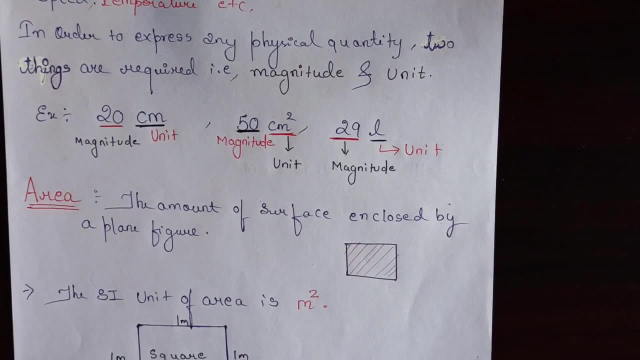 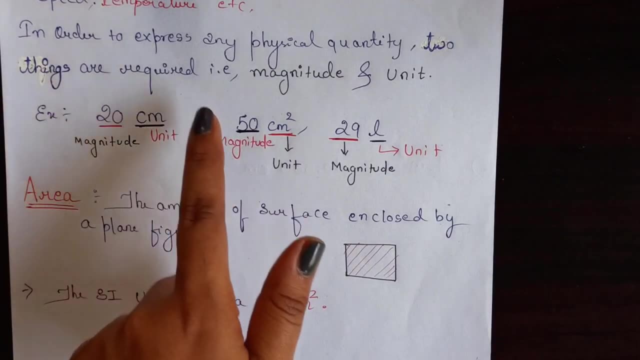 So then lets go to the question whichEveryone may have been regularly with me. We have to. Normally, if we ever express a physical quantity by measuring it, we write it in this way. For example, if I am measuring the length of something, then it is 20 cm. 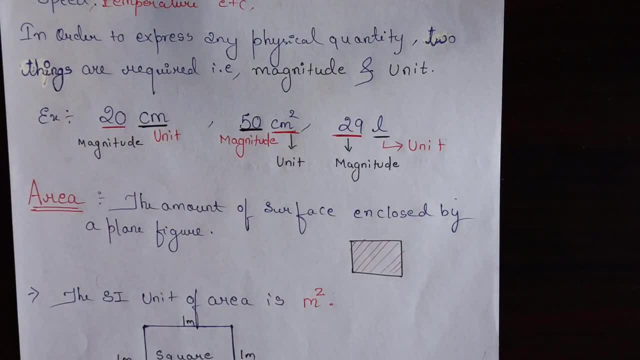 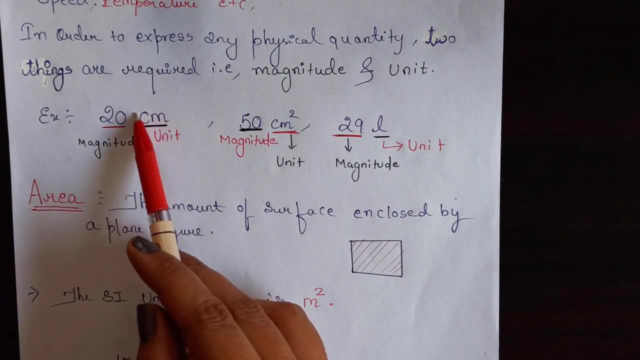 So we write this physical quantity like this. So here you can see 20 cm. In one part there is a number and in the other part it is written as CM. This is called unit. So here you can see 50 cm square, or 29 litre. 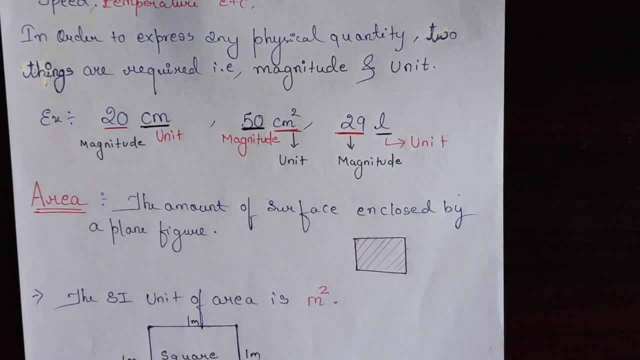 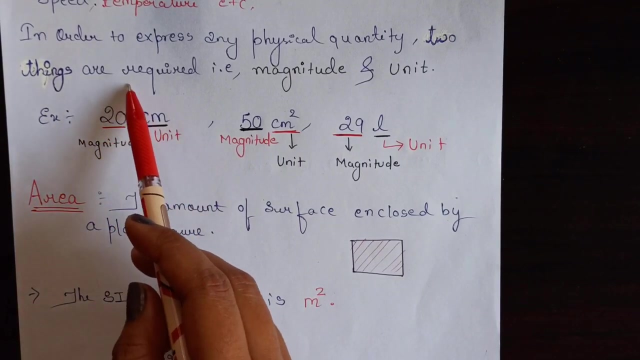 So this is definitely expressed by measuring a physical quantity. So if we ever express a physical quantity, then we write it in this way. Normally two things are written in this. The first part, which we normally write first, is magnitude, But don't think that the first thing written is magnitude. 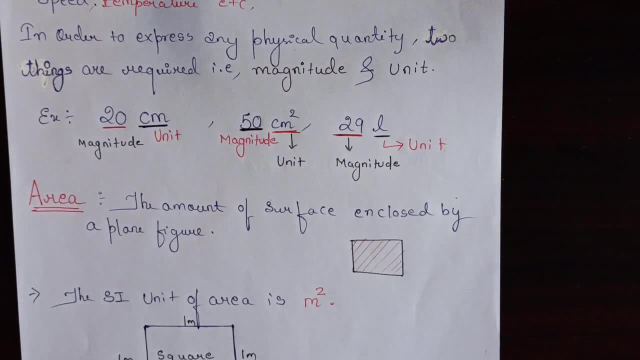 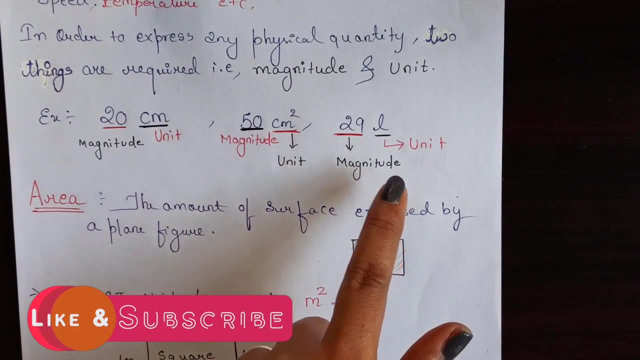 Actually, magnitude means numbers Like here 20 cm, So here 20 is magnitude. Here 50 cm square, So here 50 is magnitude. Here 29 litre, So here 29 is magnitude. Now let's talk about unit. 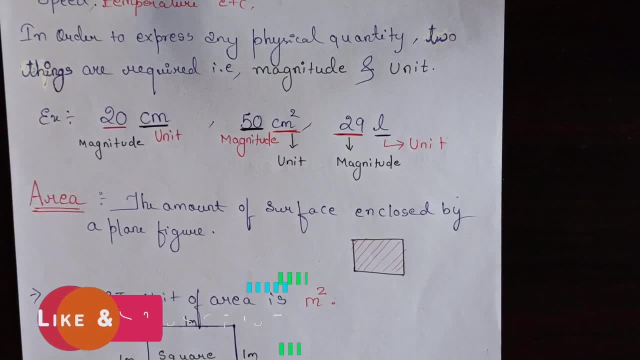 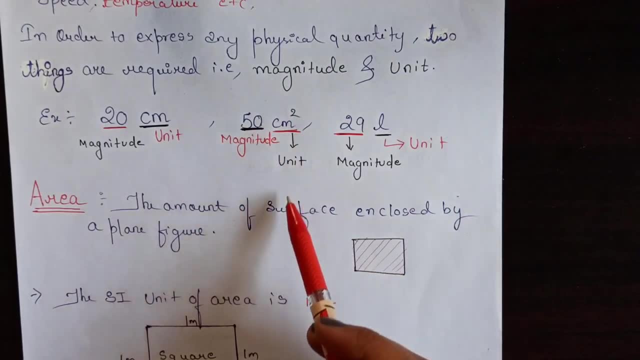 So see, the length is centimeter. We measure it in meter right, We call it unit. So here it is centimeter unit, This is area unit. Centimeter square: This is unit. This is volume: litre, So this is unit. 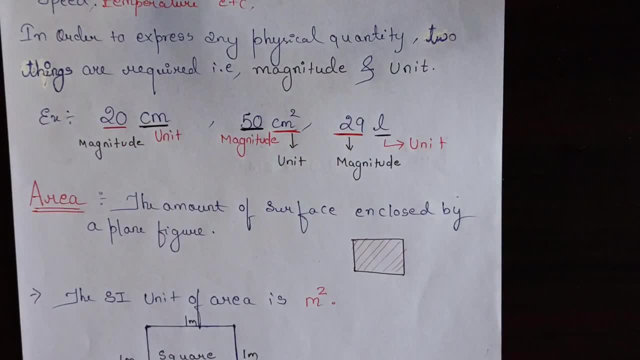 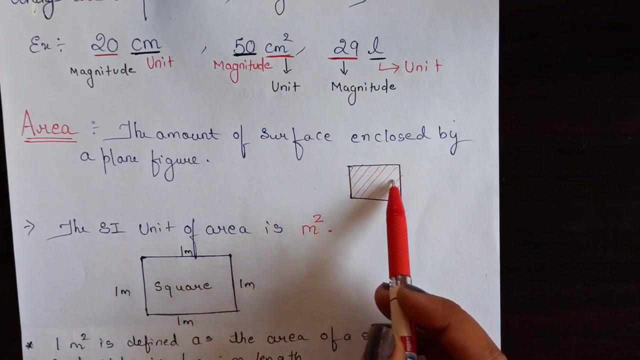 And the numbers which we can see in front are magnitude. Now we will first talk about area. Now we all know about area. We have studied in maths also. Area means amount of surface, mainly Amount of surface occupied or enclosed by a plane figure. 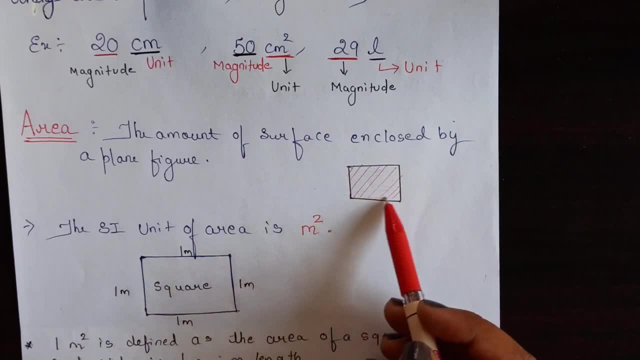 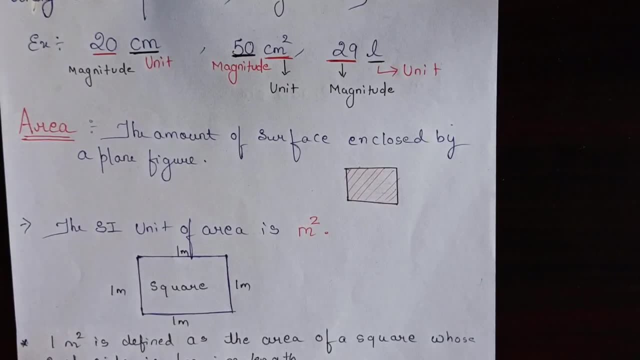 See if this is a plane figure. So how much surface is here? Amount of surface is how much occupied. I will call it area. This is different from volume. Now we have also studied that when we measure area, what is its unit? 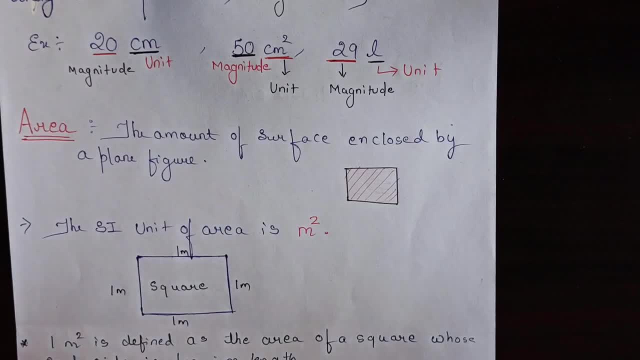 So normally the SI unit of area is the unit which is world wide accepted. World wide accepted: You may go anywhere. If you ask anyone about the SI unit of area, everyone would say meter square, Because it is internationally accepted unit. 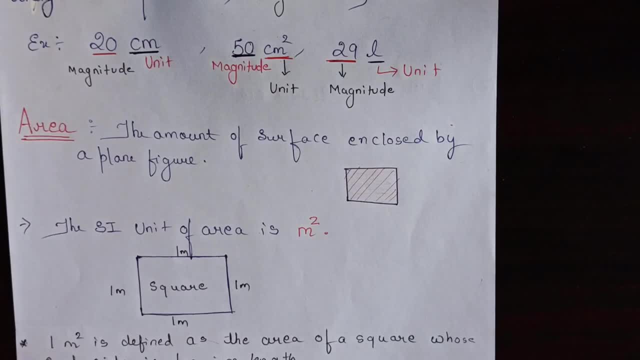 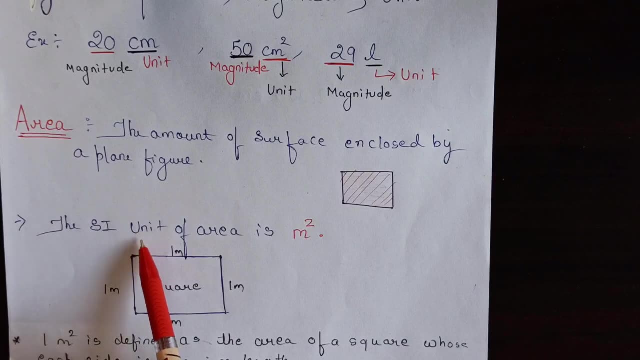 It is world wide accepted unit. If you have studied about this, I will not go into that much. so SI unit of area. when we measure area, the main SI unit of area, that is meter square. I can also read square meter, so this is a very normal thing. 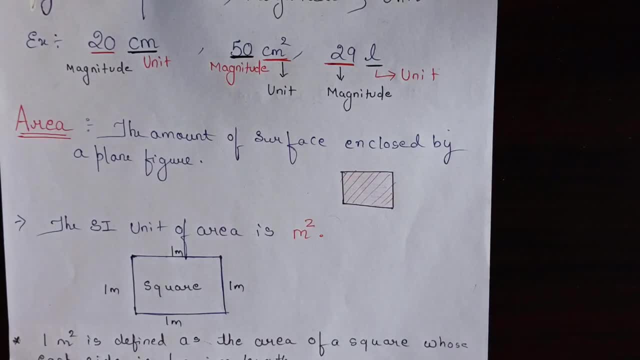 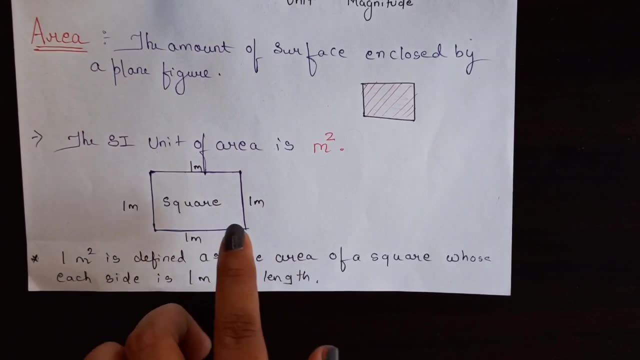 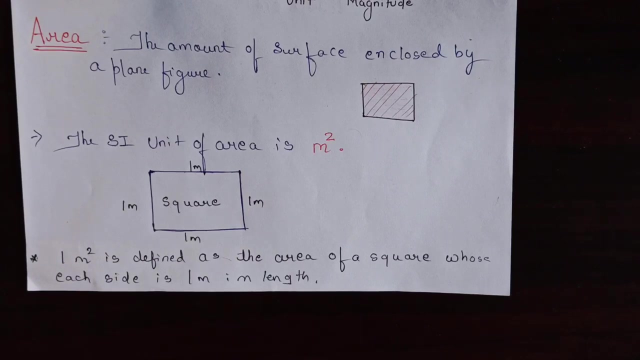 now look at the definition. it is asked in one word: SI unit is also asked. so keep that in mind. now think, if I am measuring area, then here is a square. think we have to measure square area. so we all know that square is a figure whose all sides are equal. 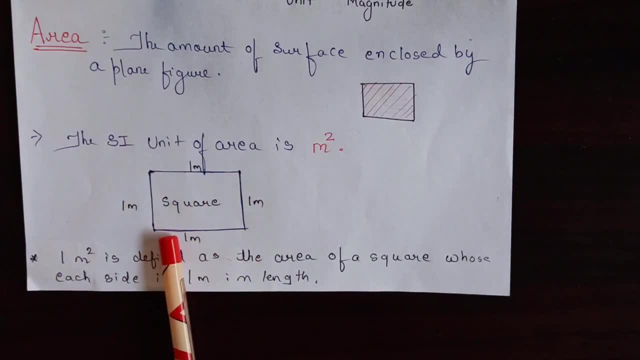 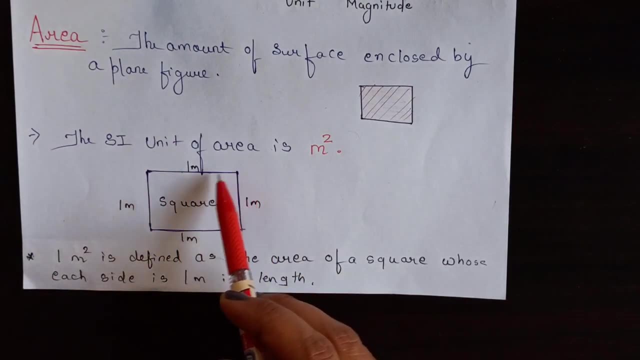 same. see, here is a square. its all sides are equal means: if this side is 1 meter, then this side is also 1 meter. this side is also 1 meter. if here is 2 meter, then this side is also 2 meter. if I talk about cm. 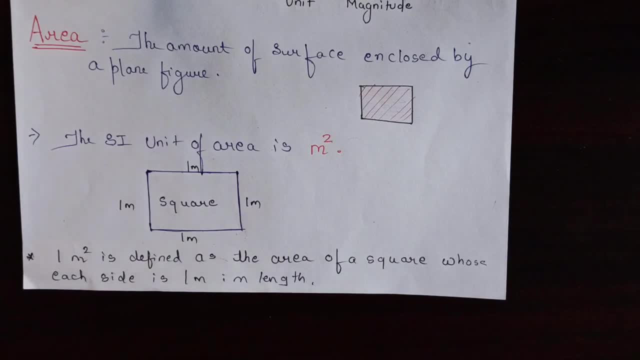 if this is 1 cm, then this is also 1 cm. this is how square works now. So when we read SI unit of area meter square, many times we get the question that define 1 square meter or 1 meter square? Now how will we define that? 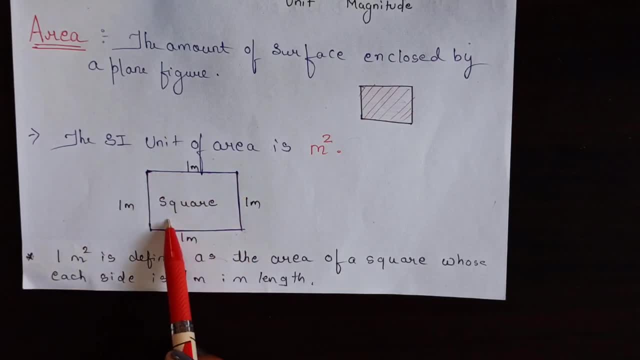 So think, here I have a square whose every side is 1,, 1,, 1, 1 meter, Every side. I have a square whose every side is of 1 meter. If I have a square whose every side is 1,, 1 meter, 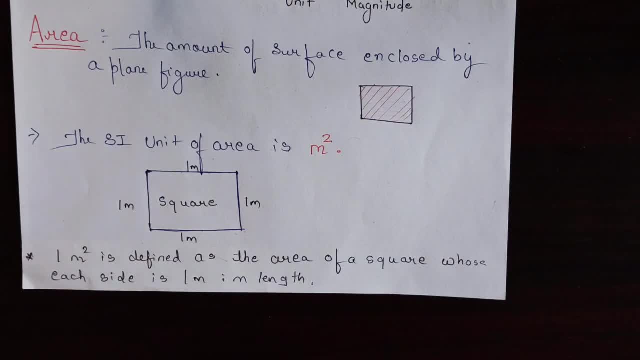 Every side is equal to 1, 1 meter. When we measure the area of that square, what will we get? What area will we get 1 meter square? So how will we define 1 meter square? It is the area of that square whose each side is 1 meter in length. 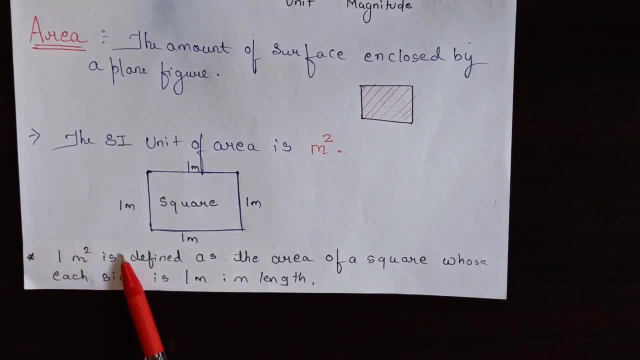 This is how we define 1 meter. square is defined as the area of a square whose each side measures 1 meter. 1 meter. So this question comes. This is very important Now if I talk about unit. So just 1 meter. 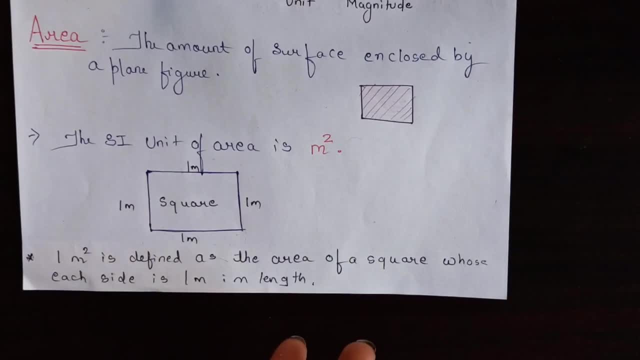 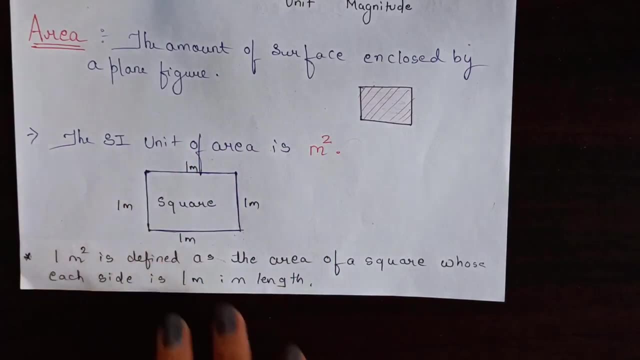 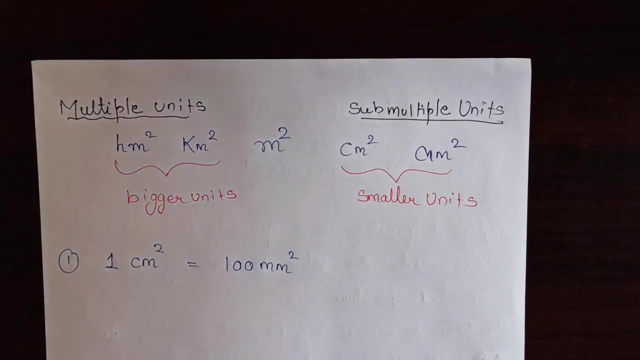 I will not measure it in meter square. It is not measured in meter square only. There are many units in which we can measure the area, But this is the unit of meter square, But if I talk about any other unit, So there are two different types of units like this. 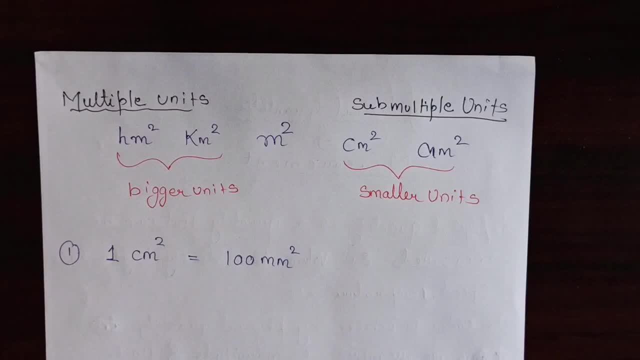 As I was talking about meter square Now I will not measure in meter square only. There are many figures like this whose side is very small. We have a square whose side is very small And sometimes when we measure the area then the side is very big. 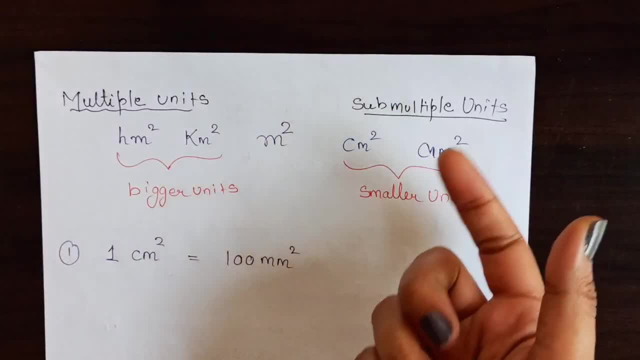 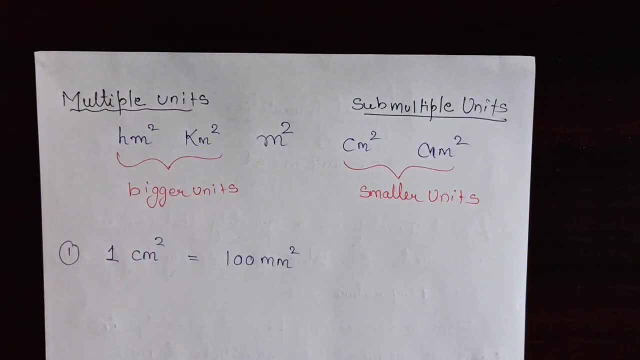 So normally all the multiple units are smaller than the meter, So this is normally the unit of meter square, But in this all multiple units are there, and multiple units are also there, So the ones that are smaller than the meter, I will call them all multiple units. 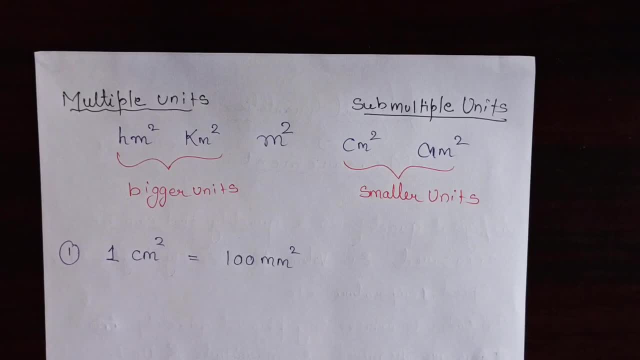 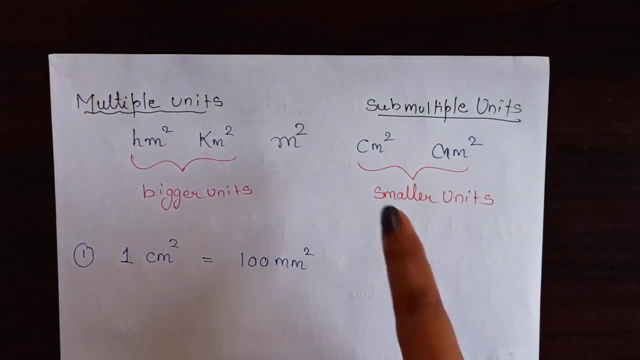 And the ones that are bigger than the meter. I will call them multiple units. So the one that is smaller than the meter will be your centimeter square, Millimeter square. So all these small units, we can measure the area in this too. 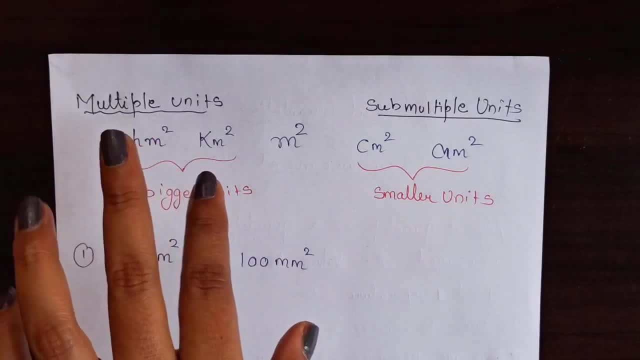 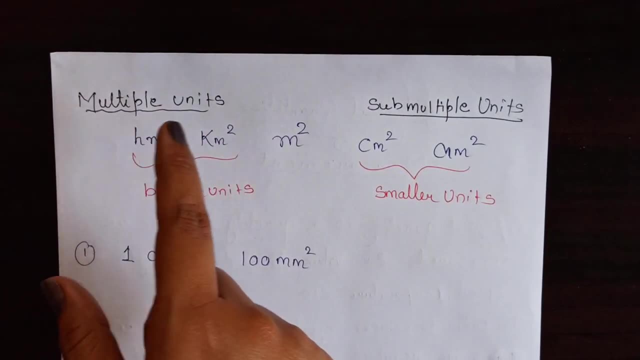 Now let's talk about multiple units. So this is a little bit. I have written it randomly like this: But if I talk about which one is bigger between these two, So the kilometer comes here and the hectometer comes here. So you don't have to understand that I have written this wrong. 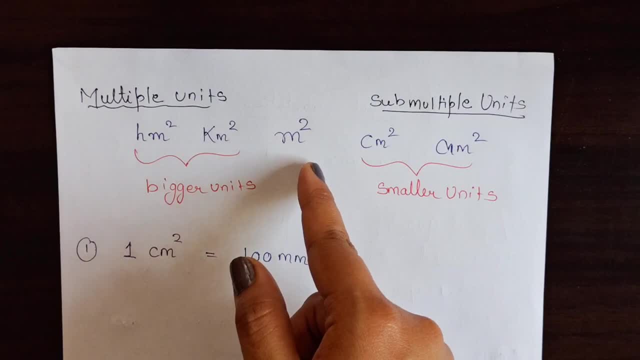 I have written it randomly like this, But here we have to see which multiple units are bigger than the meter square. So we have to remember kilometer square and hectometer square. These are bigger units. If one mark comes in the exam, then you can write it easily. 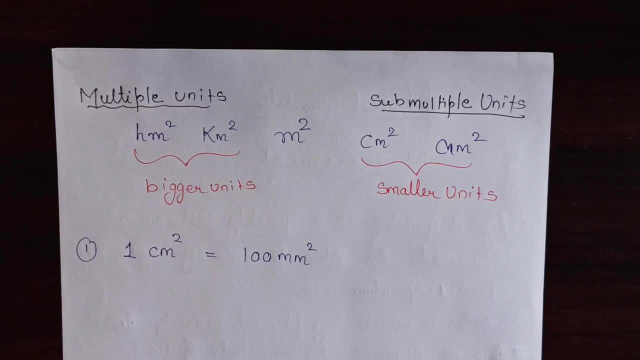 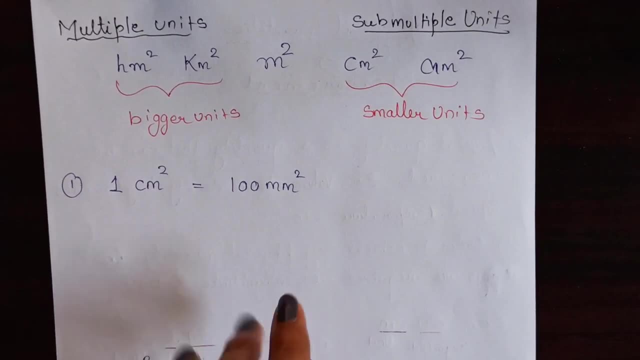 Now there is some relation between different units of area, So I have written it like this. We will try to find it, We will not mess it up And we get a question in the exam. One centimeter square is equal to how much millimeter square? 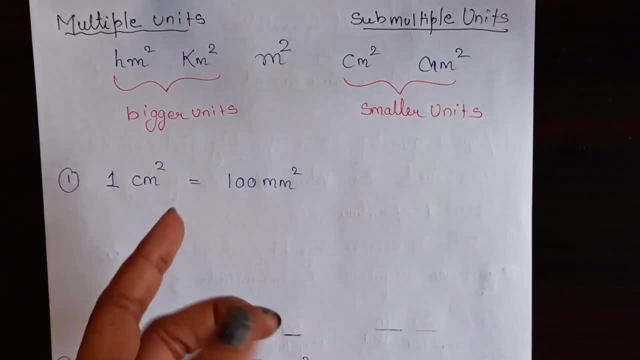 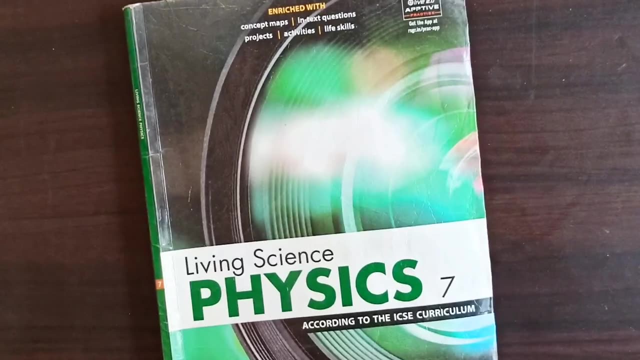 I will tell you how we can get it out, Because the poor kids remember and go, But they forget there. Someone puts an extra zero and someone puts a less zero. Anyway, Before reading further, let me clear one thing, Because I know this question. 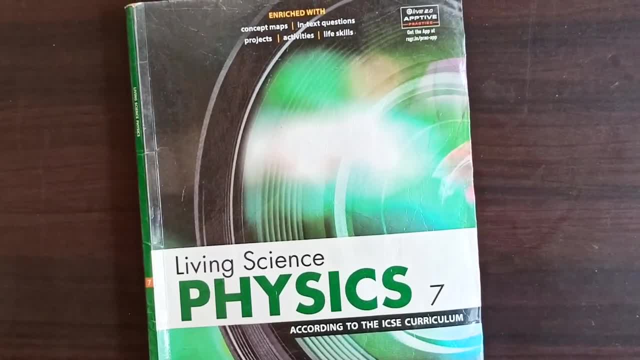 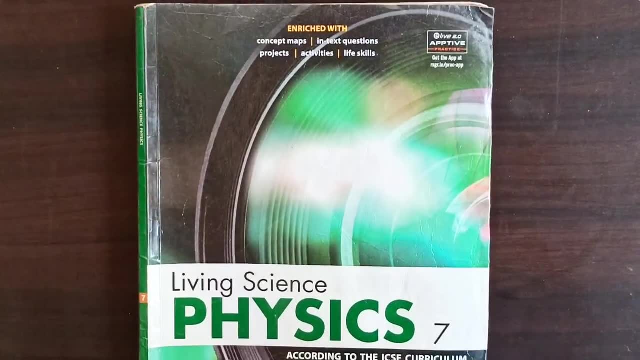 The kids will ask: Which book are you following? So this is that book: Living science, class 7. According to ICSE curriculum, by Ratnasagar publication. So this is that book. This is what I am teaching. This is what I am writing notes for now. 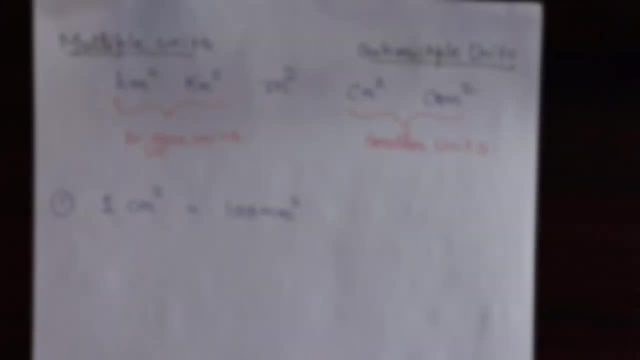 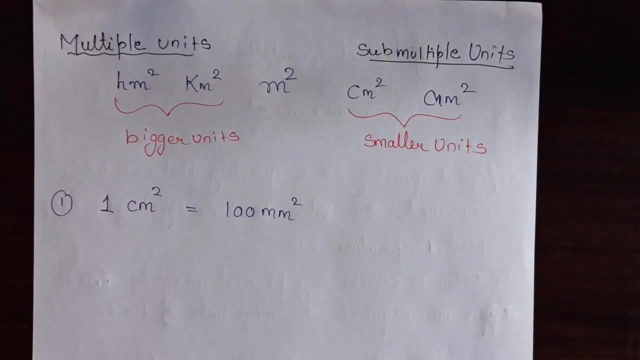 I don't have any other books available for now. Ok, So now we will see How to convert one centimeter square to thousand millimeter square. Now, this is one centimeter square. Now, this is one more question. It comes in the form of fill in the blanks of dash. 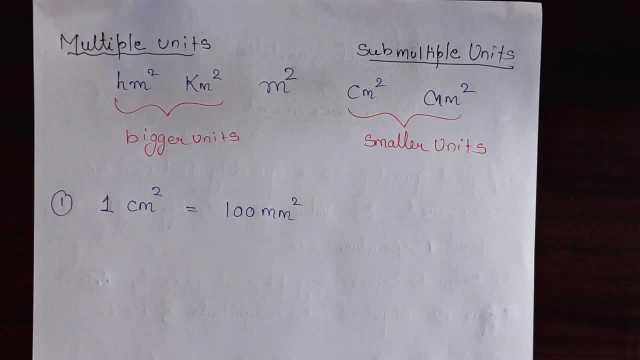 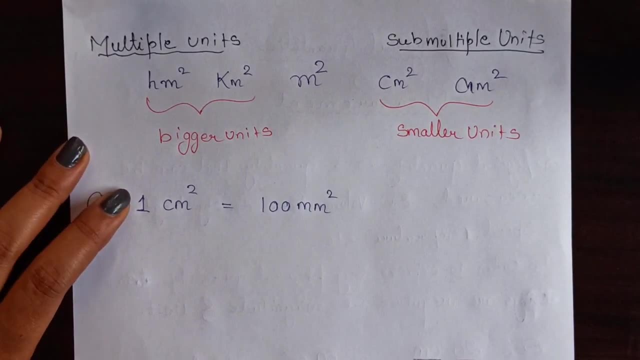 But what we have to do is Let's understand how we will convert it. So see, Now we have one centimeter square, We have to convert it to millimeter square. Ok, We will see it carefully. It is very simple. 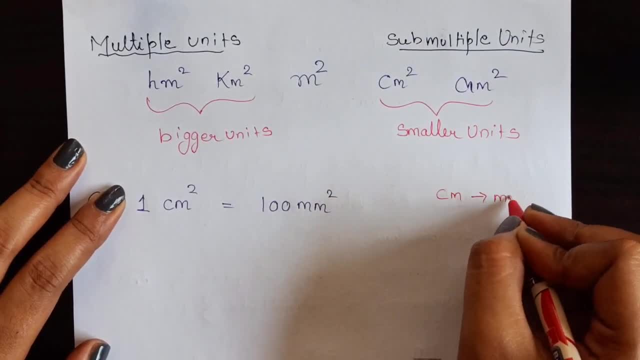 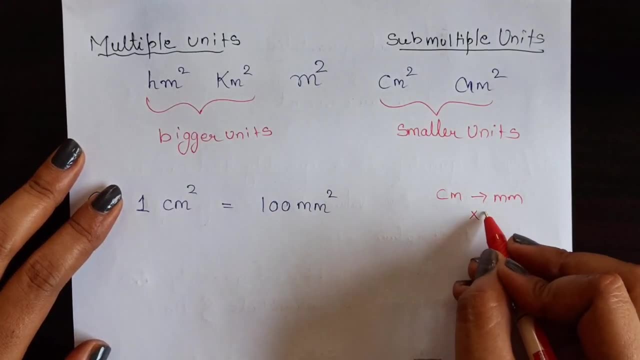 Now we know that when we convert a centimeter to a millimeter, So this is big and this is a small unit, Obviously. So if we ever convert a centimeter to a millimeter, Then we, How much do we multiply Ten? 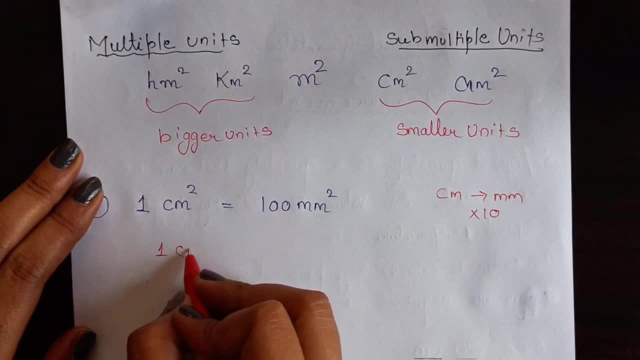 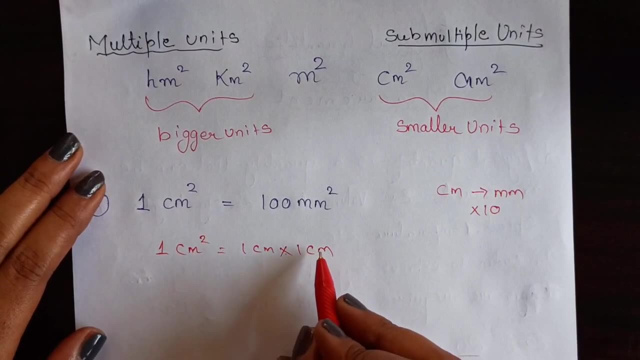 Here we start with centimeter square. So now you understand like this: This is one centimeter square. So can I write one centimeter square, like this, One centimeter into one centimeter? I can write, Because this is a centimeter square itself. 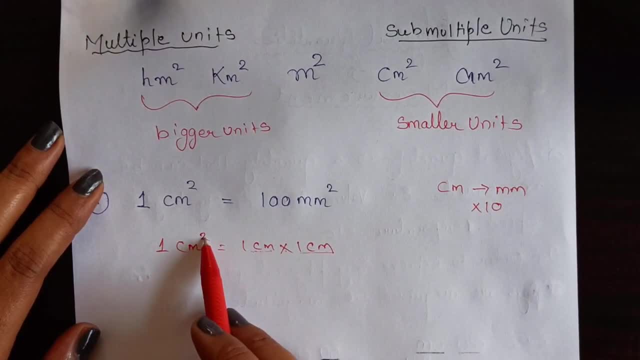 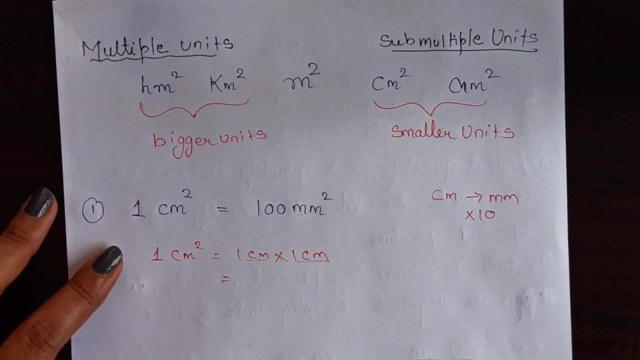 This means that this is definitely multiplied by two centimeters. That's why there is a square here. So one centimeter square is equal to one centimeter into one centimeter Now. So where do I have to convert this centimeter now? 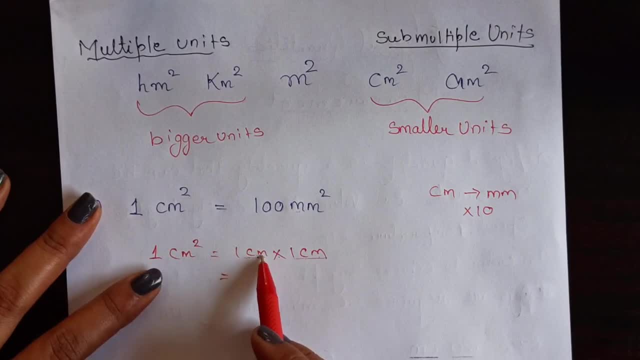 In millimeter? Ok, It is written here. Do it in millimeter Now. how many millimeters is one centimeter? Ten millimeters. Ok, Remember this thing a little. And what to remember. I will also tell you a way to do this. 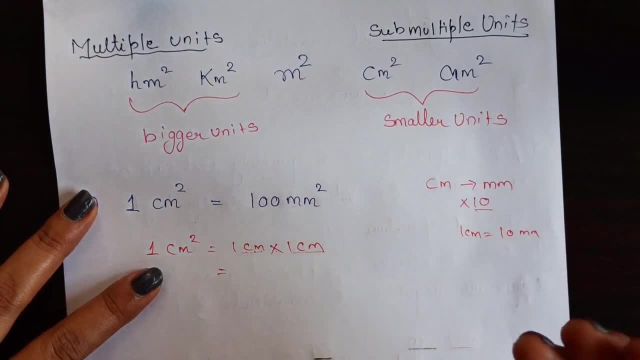 I have told the small children, like four or five students, Because this thing comes from then In their math. Ok, So it is very easy. We didn't know for a long time. Actually, we knew, but we didn't pay attention When we were small. 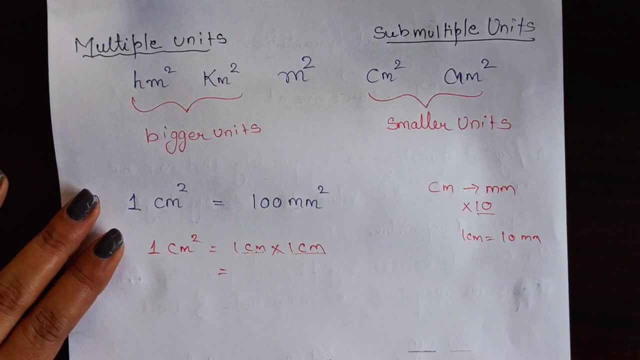 But now the children are paying a lot of attention And they don't hit the baton. Just tell them the way, and they do it easily. So one centimeter becomes ten millimeters. Now we have to convert it to millimeter, Ok. 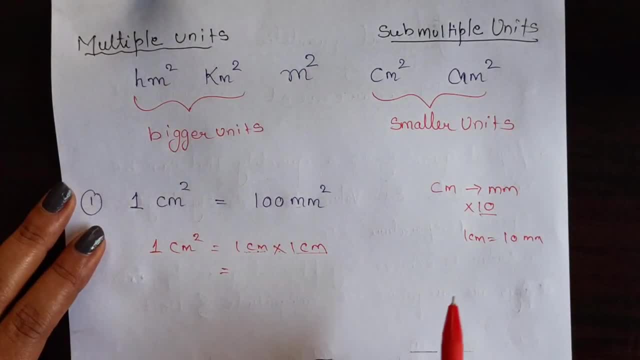 Now we have to remember this, Remember this, Remember this. So one centimeter becomes ten millimeters. So here, instead of one centimeter, I will put ten millimeters. Then again into For one centimeter, again we will put ten millimeters. 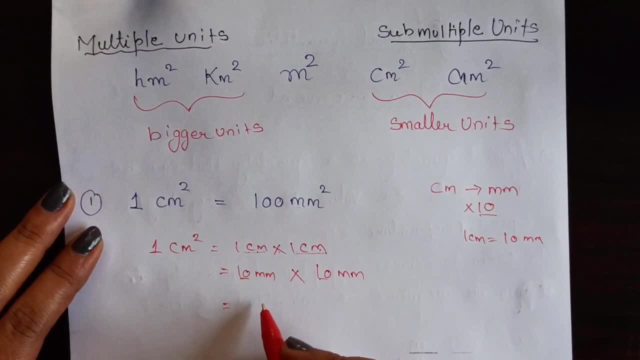 Now just multiply this ten and ten, So ten into ten is hundred. Millimeter into millimeter, Millimeter square. So see, Did we get it or not? Hundred millimeters square, So one centimeter square is equal to one hundred millimeters. 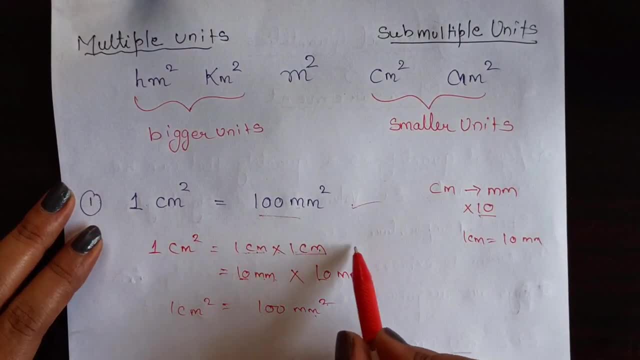 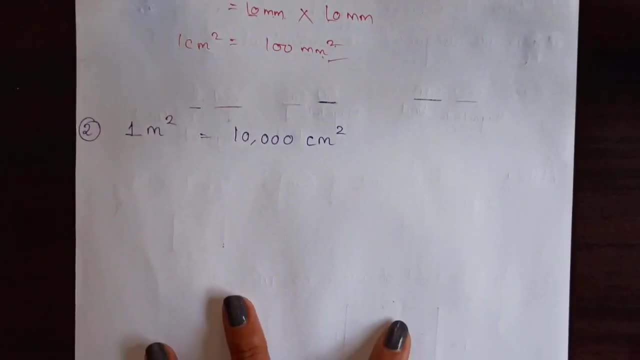 So where we were hitting it Now we are hitting it Here. we know how to convert this, How to convert So this. you can do it easily. Similarly, this is all related to the area. Ok, You have a relation between different units. 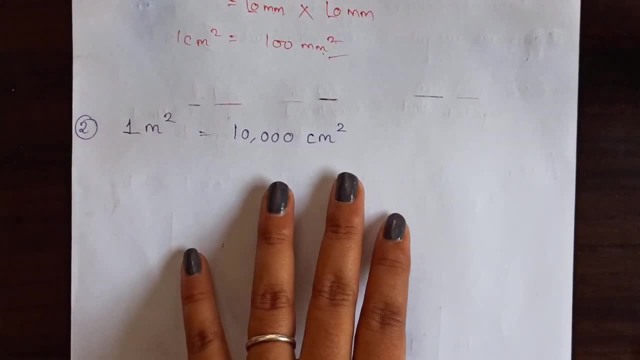 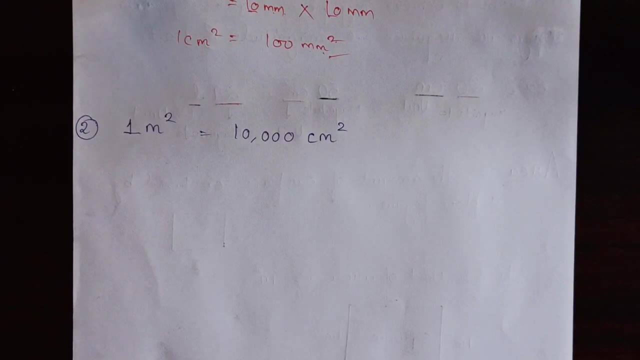 How one unit is related to another. We'll see now How is meter square related to centimeter square? So let's do this too: Convert this too. See Again: Here is a meter and here is a centimeter. That means, if I have to convert from meter to centimeter, 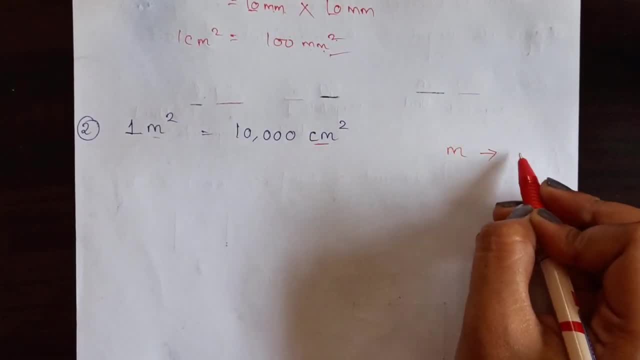 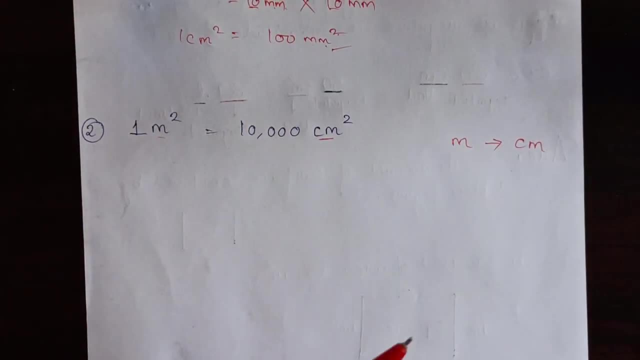 Yes, then I will also use this. I have the meter, Which is some little bit of money, with my Okay, So it is happening, isn't it? It was a meter. it is changing it to a centimeter. Square is. square means okay, square is. we will see. 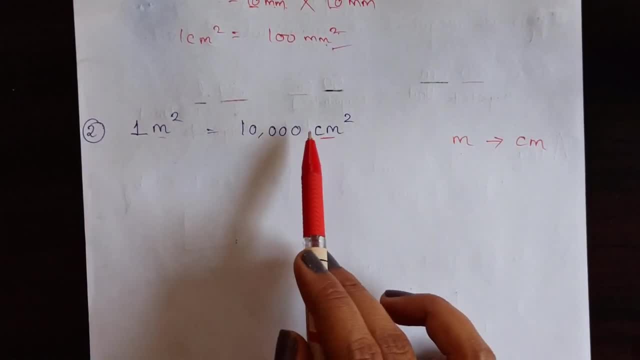 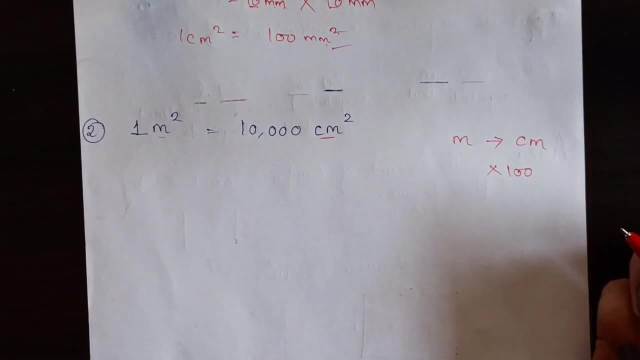 But first pay attention to this: Here is a meter and write meter In which to change In centimeter. So to change meter to centimeter, always, always, what do we multiply 100.. And one more thing we know. 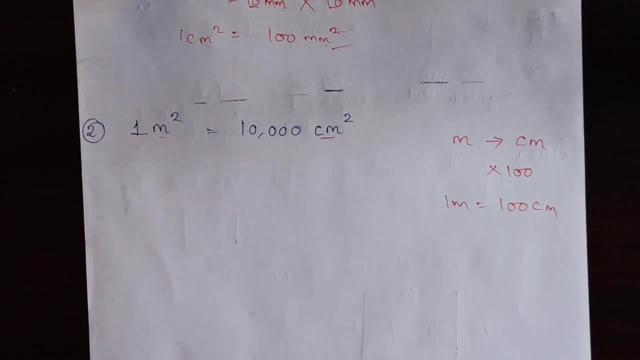 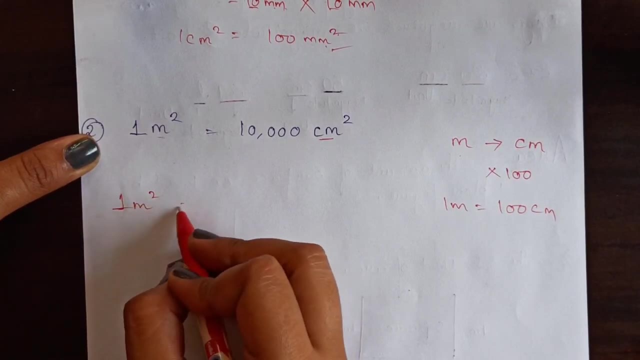 that 1 meter is equal to how many centimeter, So 100 centimeter. So we will use that only here. Let's start from here. Write 1 meter square. Can we write 1 meter into 1 meter? 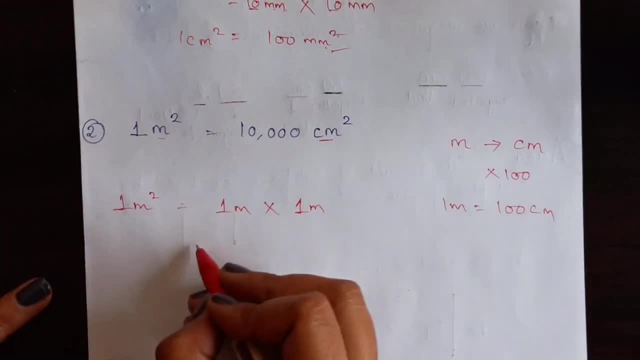 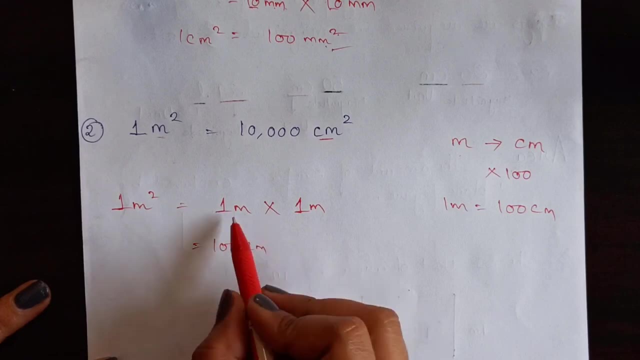 Yes, we can. Did we break this and write? That's it Now, it is so easy. 1 meter is 100 centimeter, Because I have to do meter in centimeter. By saying I am writing 1 meter. 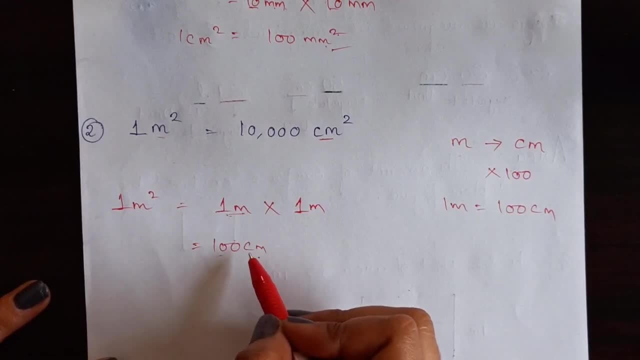 as much as centimeter is happening Here. you don't have to write kilometer, kilometer, kilometer, Whatever is required. we have to put that only Again into for 1 meter. again, we will write 100 centimeter. 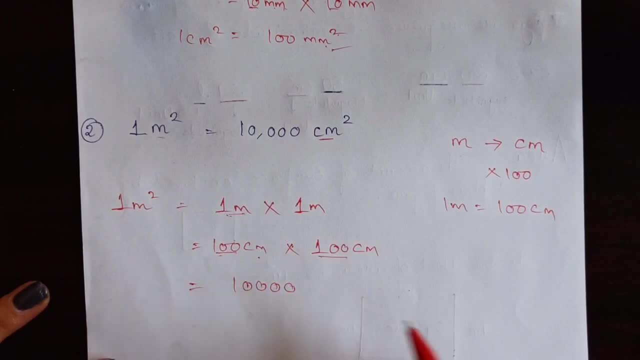 Now let's do into 100, into 100.. How much is this? 10,000 is done Then centimeter square, Because centimeter into centimeter, centimeter square. See, I got the same thing here. 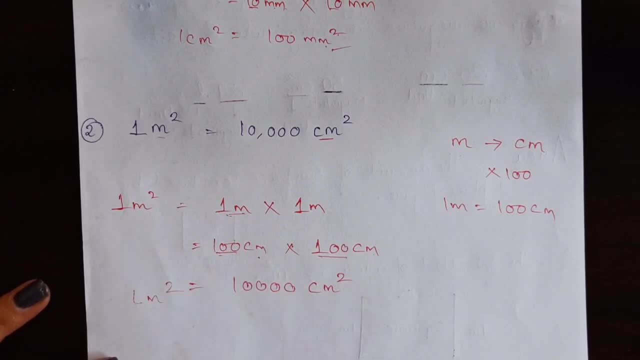 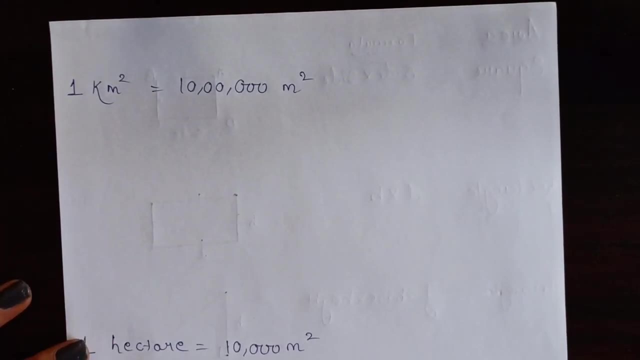 So 1 meter square is equal to 10,000 centimeter square. This is very easy. There are two more to do. We will do that too. Now, 1 kilometer square is equal to how much is this? 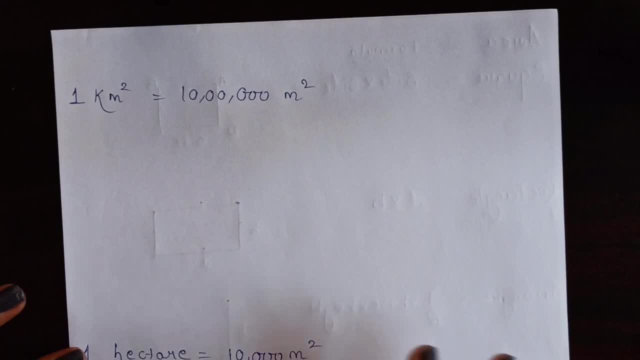 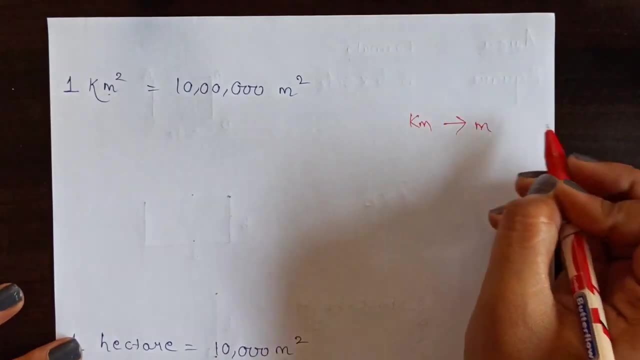 10 lakh meter square. 10 lakh meter square. Let's convert this also. Again, this is kilometer, so let's write kilometer And this is meter. It means we have to convert from kilometer to meter. 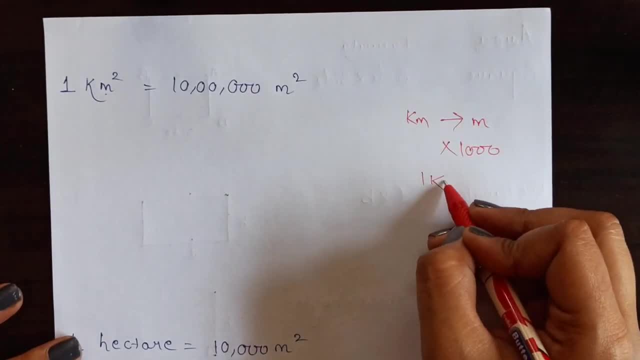 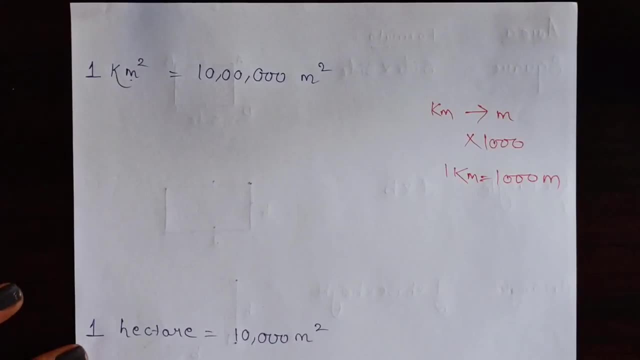 So how much do we do? 1000.. That means 1 kilometer is equal to 1000 meter. If you remember this, you will be able to do this easily. Okay, Now write 1 kilometer square. 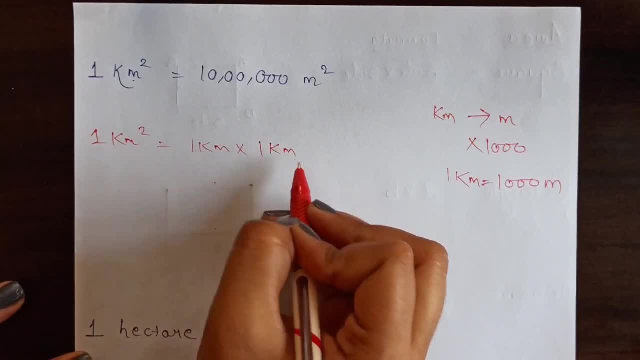 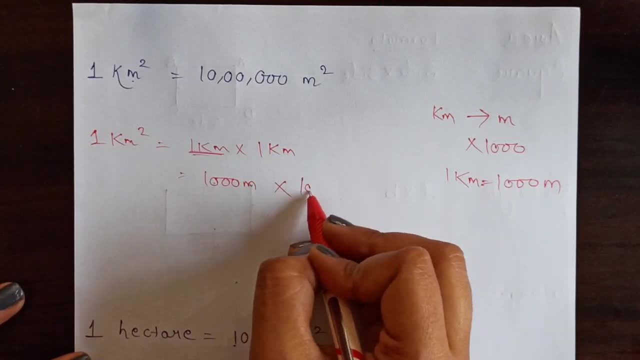 Break this. What will this be? 1 kilometer into 1 kilometer. Now 1 kilometer, how much is meter 1, 1,000 meter into 1 kilometer. Again, we will write 1,000 meter here too. 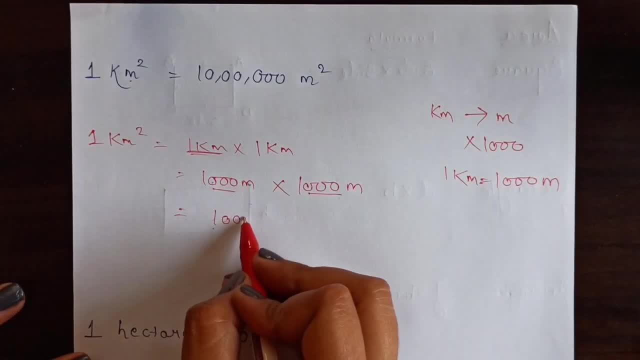 Now, here 3 zeros, here 3 zeros. We will multiply both of them. So what do we have to do here? We have to put only 6 to 0.. One more thing Here. see, this is 1.. 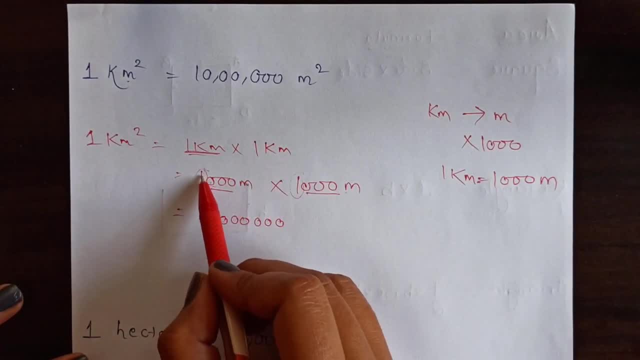 Because in the back everything is 0.. In the back everything is 0.. Multiply the numbers in the front: 1 into 1 is 1.. Now multiply the remaining zeros here, Then meter into meter. meter square. 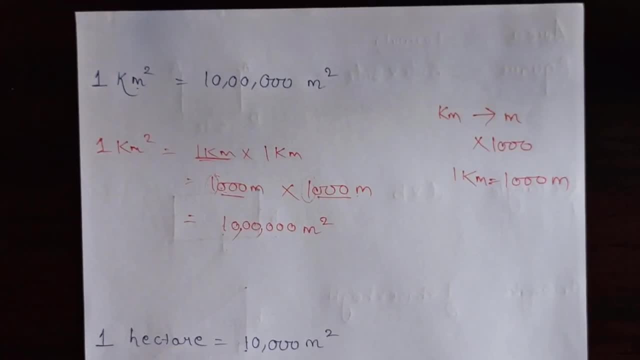 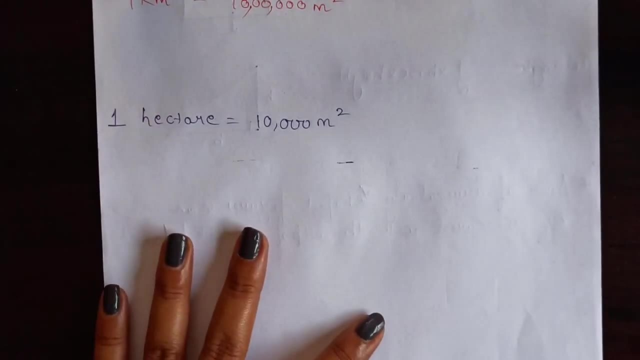 So see, did we get this or not? 10 lakh meter square. This is also easy. It will be done easily. Next, And this is the last one, This is hectare. Now, how much meter square is 1 hectare? 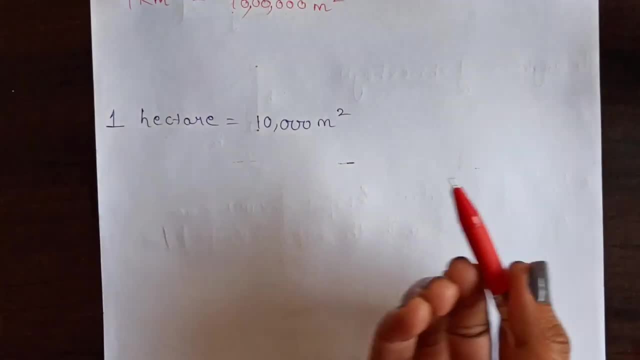 We have to see this too. Now again what I told you: this is 1 hectare right. Yes, this is 1 hectare. Now see, normally we read this conversion: one right. What I told you. I tell the children we do it like this. 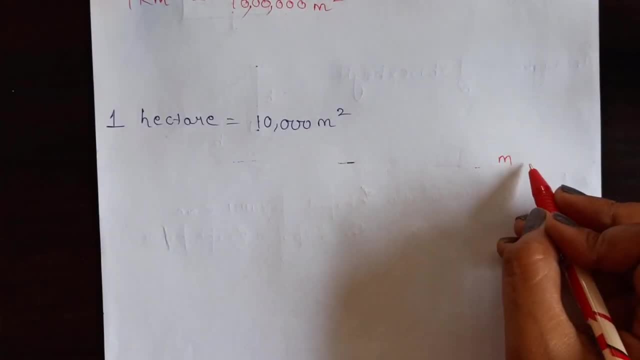 See, like this is meter. right, I wrote meter here. Meter is smaller than decimeter, See meter, then centimeter. I hope you can see it. then it became millimeter Bigger than meter is decameter, then hectometer, then kilometer. 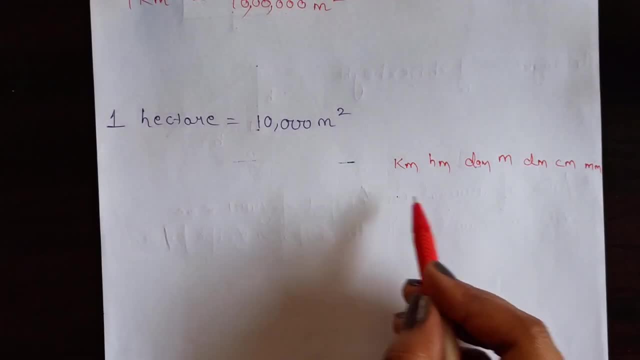 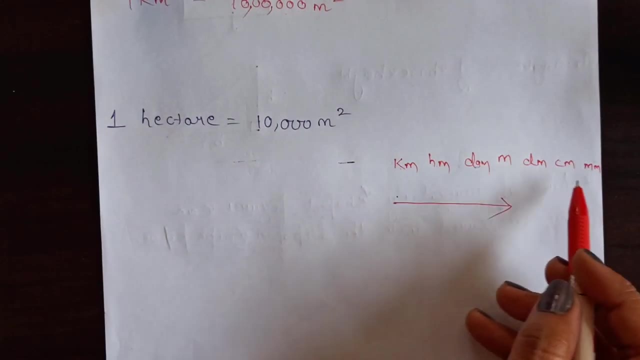 See, we do it like this. This is actually the way Now. this is bigger than small. Whenever you go towards bigger than small, decreasing order, because this is big, kilometer meter is small, these are all small. Whenever you go towards bigger than small, you will convert. you will always multiply there, always. 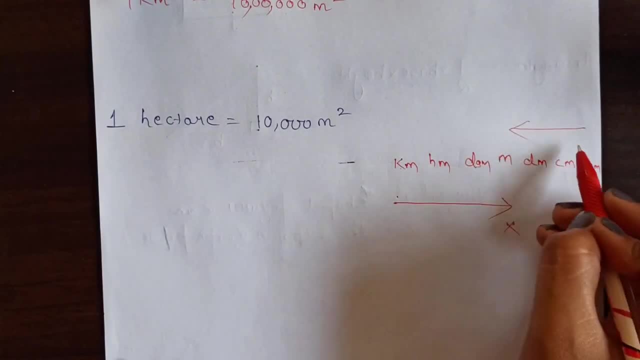 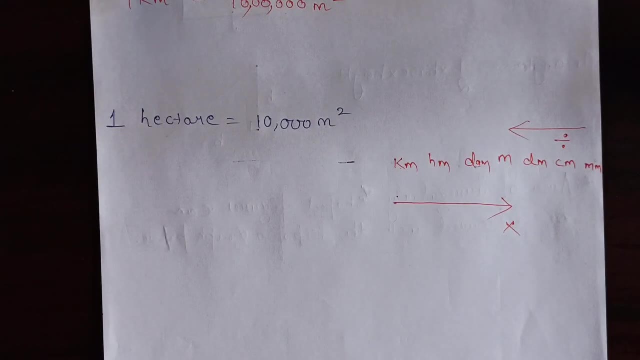 And if you are going in reverse, if you are going towards small to big, then we divide there. Now you will say, madam, what to divide and what to multiply. We will not multiply any number, right? Yes, we don't have to do anything at all. 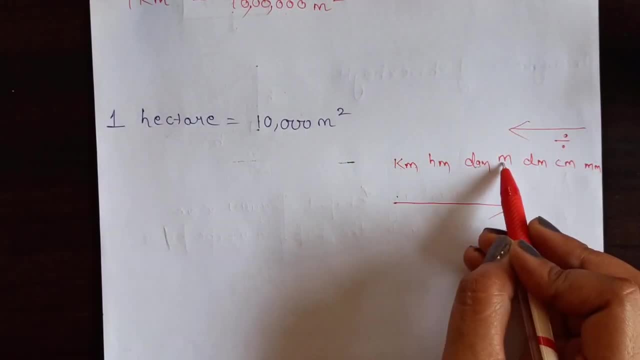 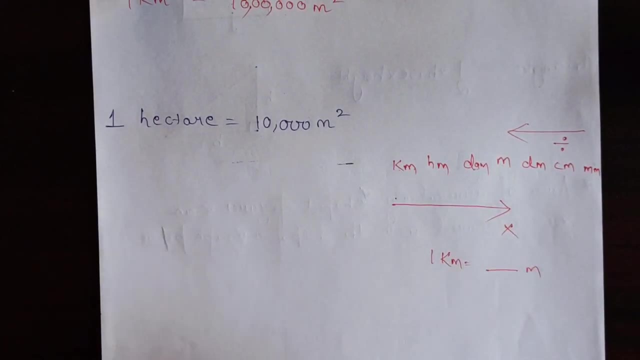 Now, as you think, I have to go from kilometer to meter, So I am writing it like this: how much will be 1 kilometer? Normally I am writing 1, 1.. Now from kilometer: see what is given first: kilometer. 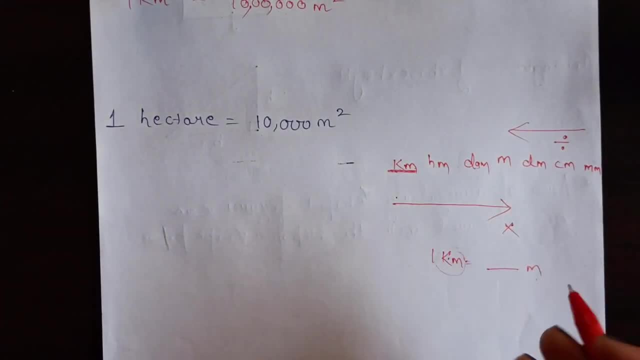 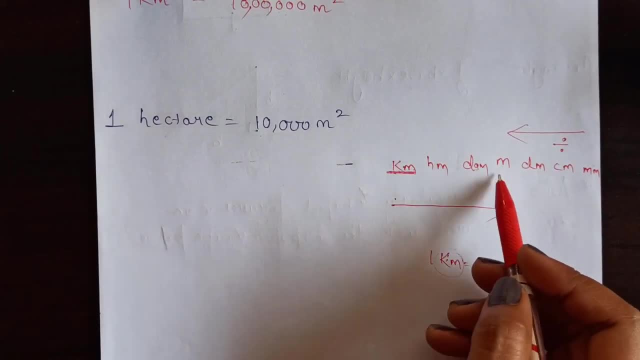 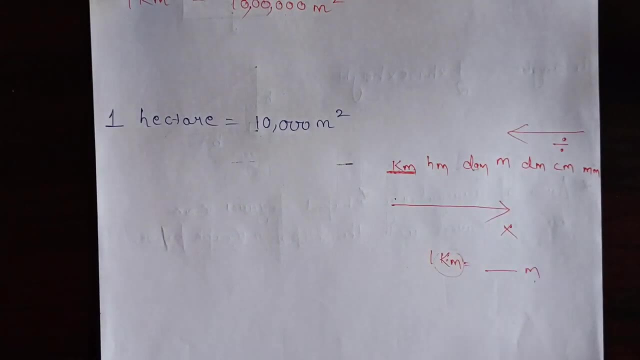 So I saw kilometer. is this Now? where is meter? Meter is here, Meaning I will go from here to here. How am I going Towards? bigger than small. So what I have to do Into, But what do I have to do? 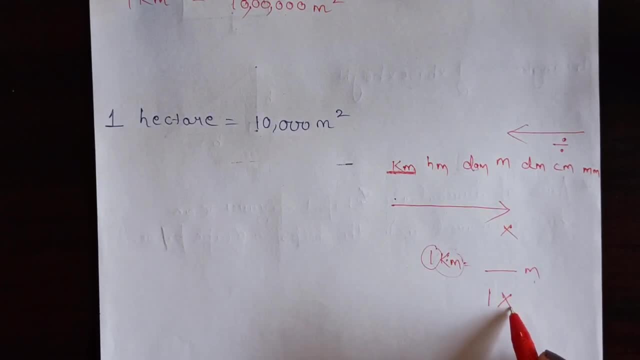 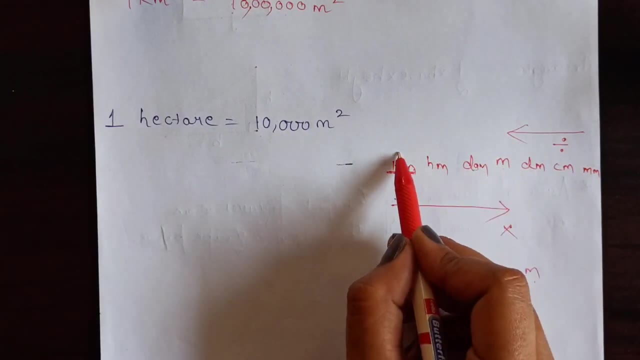 So whatever number is here, say 1,, so 1 is written into. Okay, Now I have to convert it and do it into. Now, from kilometer to meter you have to jump 1,, 2,, 3.. 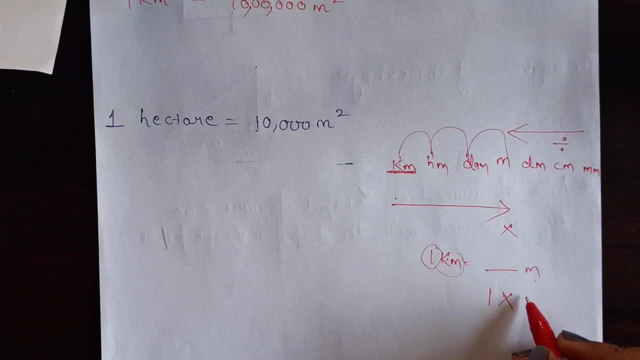 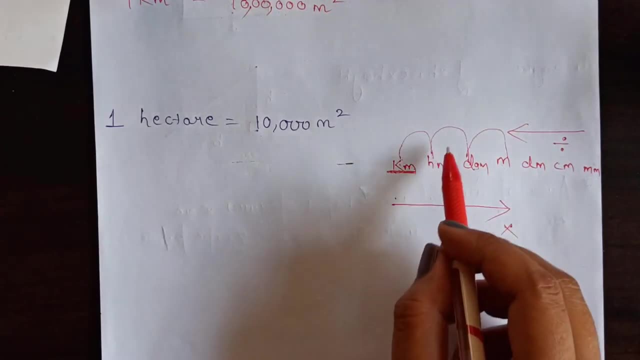 How many times we jump? 3 times we jump, Okay. So here apply 1 and then apply 3 zeros. don't apply 2. here it applies with 1 only. Ok, you guys jump 3 times, and if you are going from big to small, then multiply it. 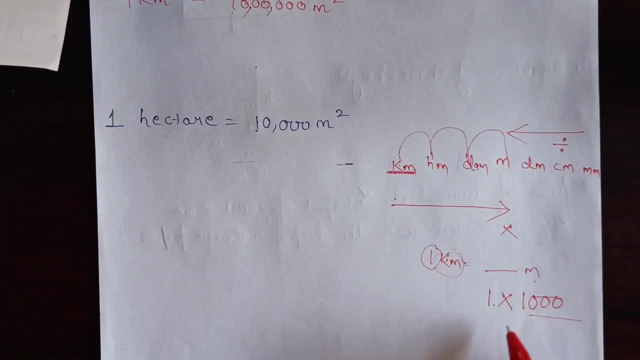 And if you jump 3 times, then apply 3 zeros with 1.. Now what will be? 1 into 1000? 1000 meters. So you guys say for yourself: you don't know that 1 kilometer is 1000 meters. 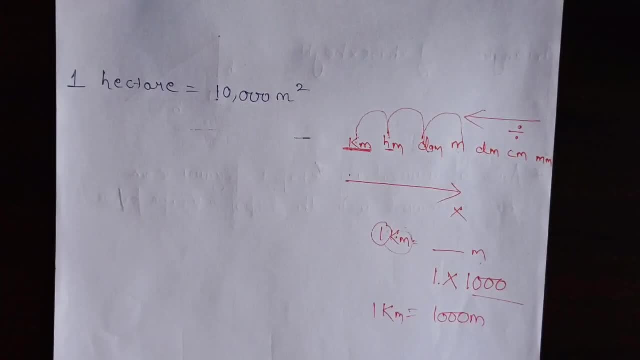 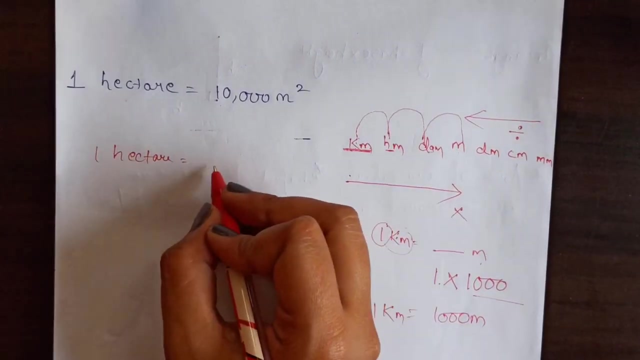 Now we will use the same thing in Hector. So now let's convert 1 hectare to meter square. See how will we convert this. So before that, know that 1 hectare is 1 square hectometer, 1 hectare actually means 1 square hectometer. 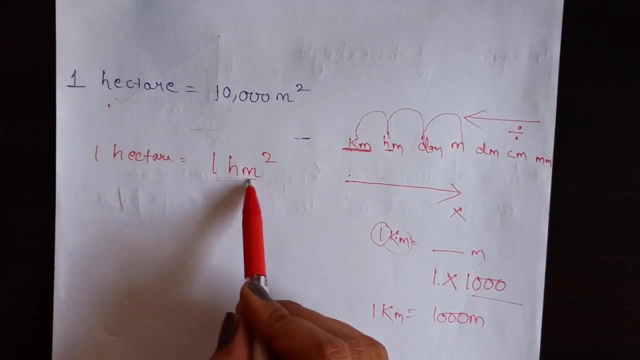 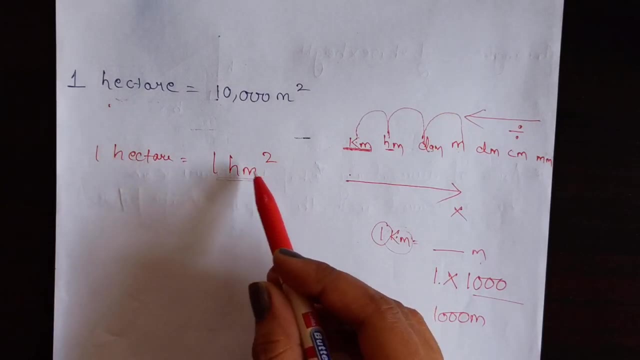 So now I will use this in place of this. Ok, so let's start. So here already I have written 1 hectare, For that I can write 1 hectometer. Now I can divide this 1 hectometer like this: 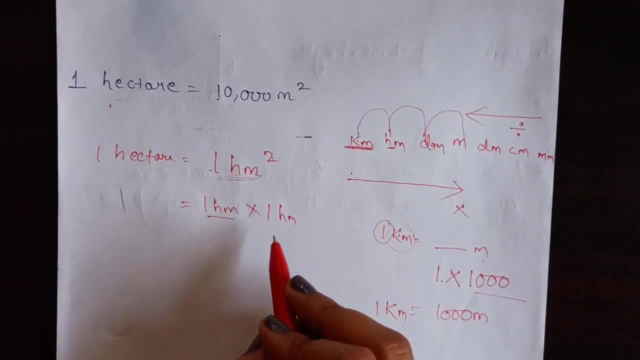 1 hectometer square is equal to 1 hectometer into 1 hectometer. Now see this hectometer in which I have to convert In meter. So how to convert it. See where is the hectometer. Here it is. 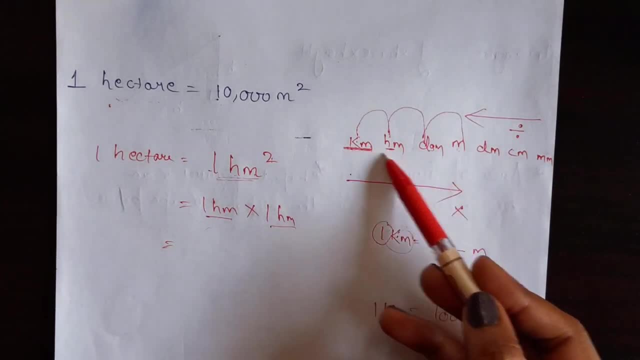 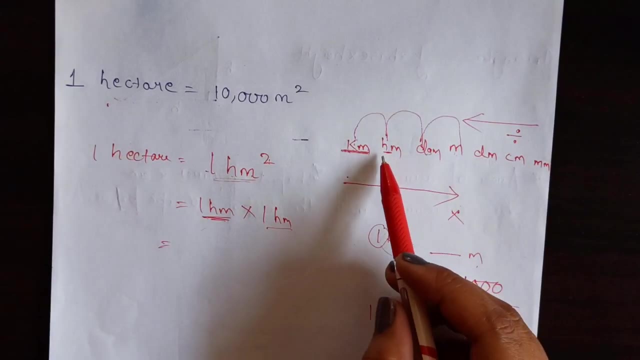 Where is the meter? Here it is From big to small. we will go like this. So what will we do? We will multiply. So let's do one thing: This is 1 hectometer. Now let's see what we will multiply. 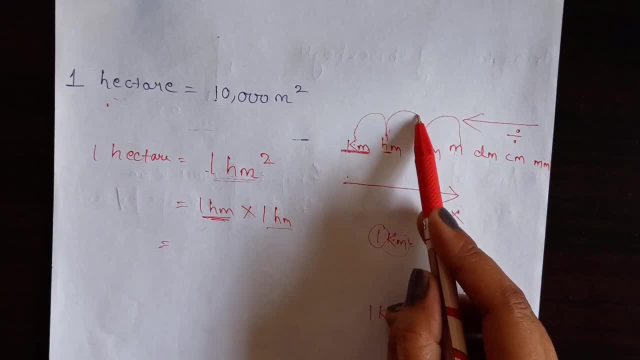 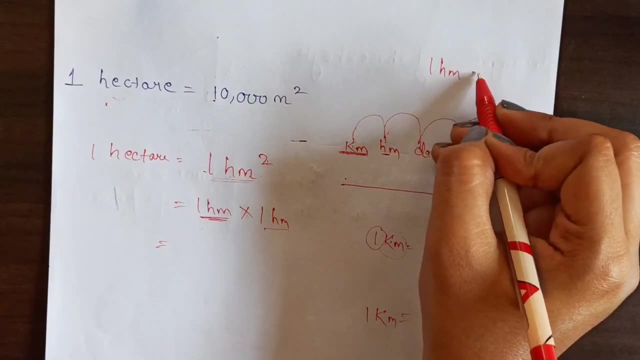 What will we write in place of this? Ok, So 1, 2.. We are jumping 2 times here. 2 times means, if this is 1 hectometer, we are jumping 2 times, right. So here we will multiply by 100.. 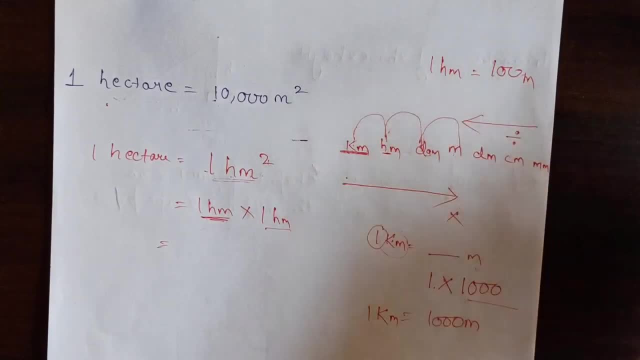 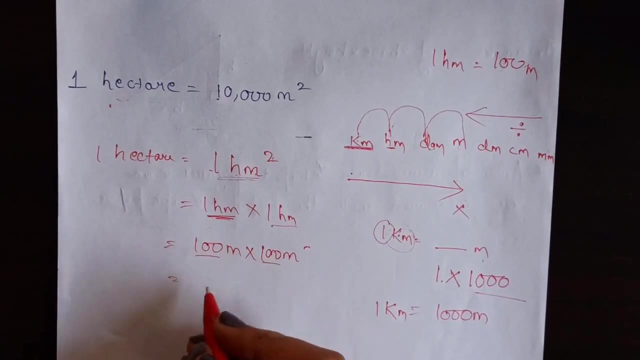 With whom? With this: 1. Because we are jumping 2 times, so this will be 100 meters. So, in place of 1 hectometer, I can write 100 meters into 100 meters, And this will be 100 into 100.. 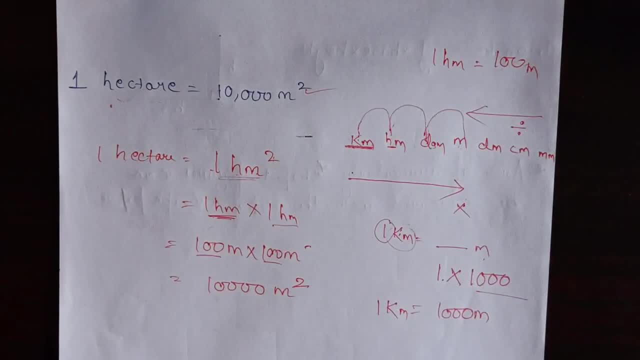 How much 10,000 meters square. So I got the same thing. I got the same thing here, Ok, So in this way you can easily do conversion without any hassle, Because it is related to this in the exam. It won't take much time. 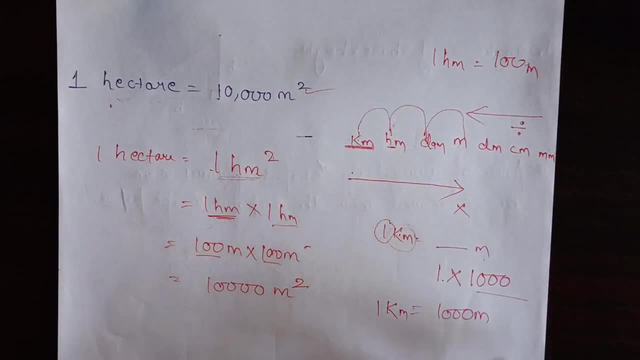 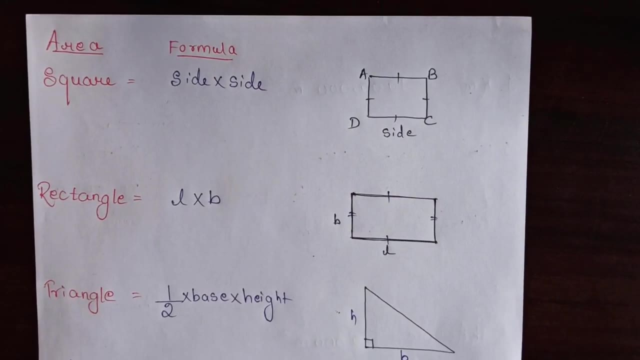 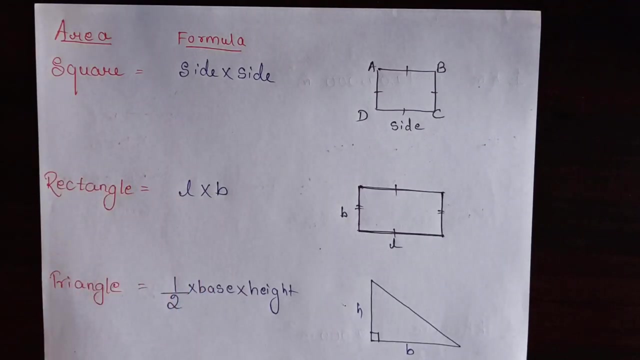 If you remember this thing, then you will do it easily Now. Now let's see some of the formulas to calculate area for different figures, Like here: I have a square, So we have read that if we want to calculate area for square, 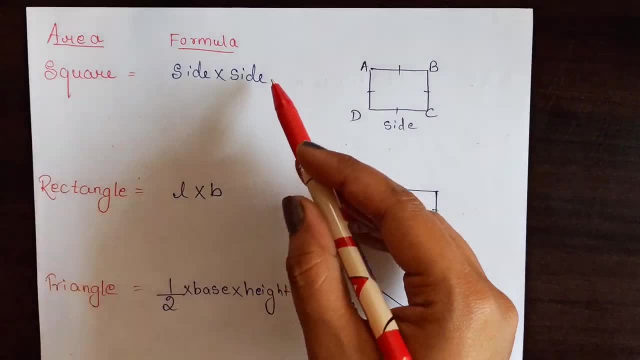 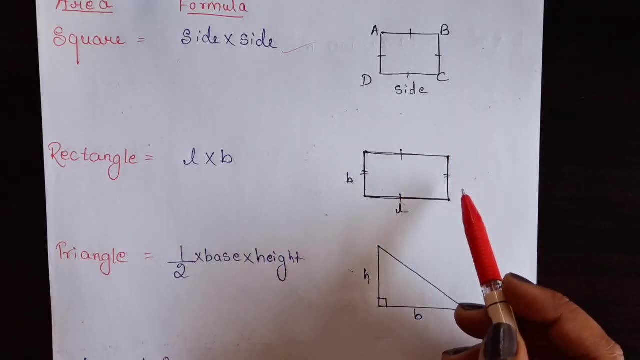 because side of square is same, so its formula is side into side. This is a simple thing. See, This is rectangle. We know, in rectangle, two sides have length and two sides have breadth, which are equal. Now here you will think. 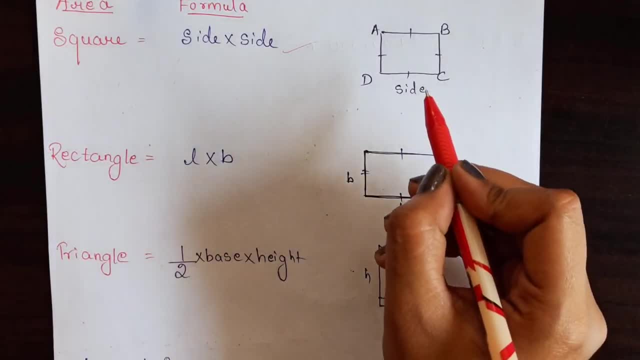 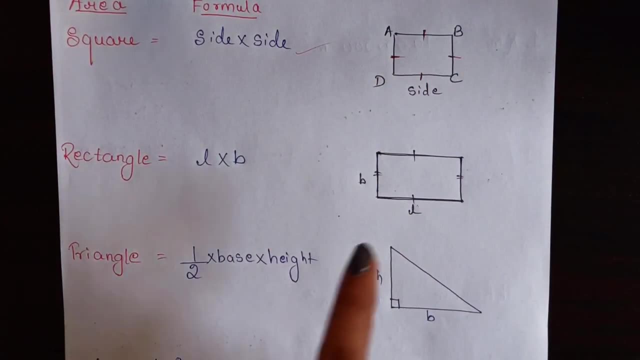 what have I done? Like, if I start from square, then you see, I draw a line from each side like this. So you see, when you go to higher classes in maths, you will see that there is a figure like this and there is a line like this. 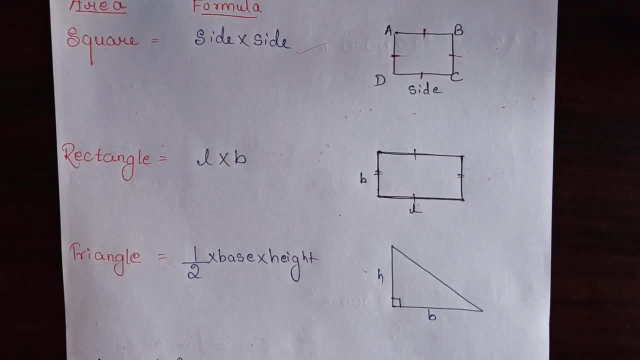 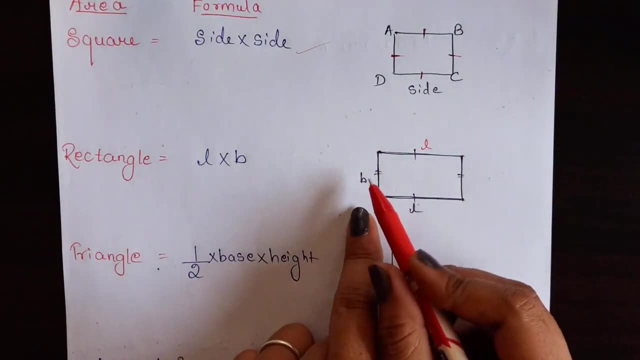 This means, like these four lines are same in all four sides, so these four sides are equal. Similarly, this is length And the line I have here, the same way I am up. so this length is same And similarly breadth is same. 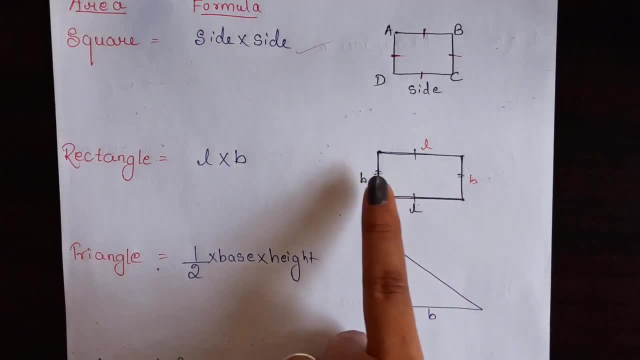 Whose Of rectangle And see the line I have drawn. two here means this side, this side is same and this side, this side is same. Its area formula is length into breadth, Now triangle. so this is our right angle triangle. 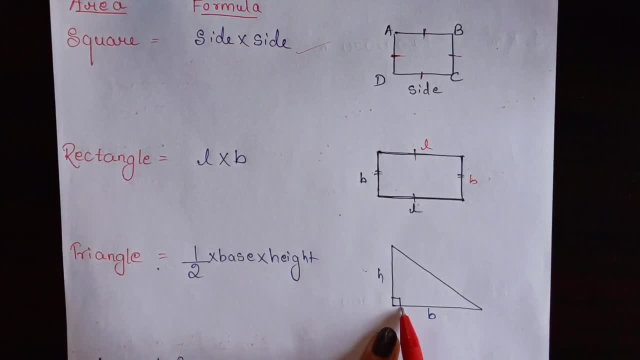 whose height is, which is also called perpendicular, And this is the base. If I have to find its area, its formula is: half into base into height. This edge means here is the height. This is also called perpendicular. Now in the book. 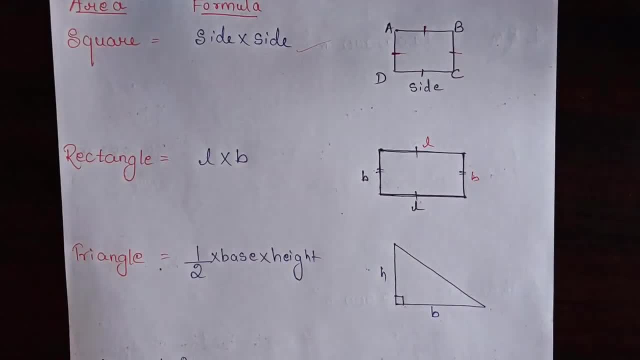 measuring area of irregular figure is given For this normally what we use, We use graph paper. I will tell you that some other time, So now we will read about volume. So now let's see some volume Now. 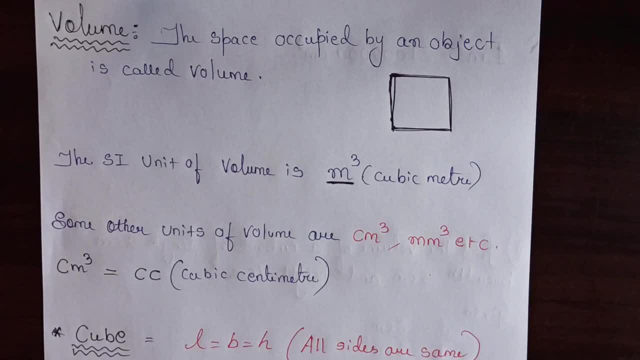 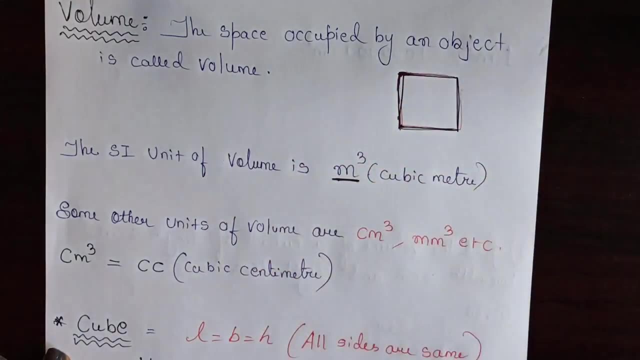 everyone knows about volume. Volume means it is the space occupied by an object. For example, this is an object. This occupies as much space as it takes. This occupies as much space as it takes. What do we call this? This is called volume. 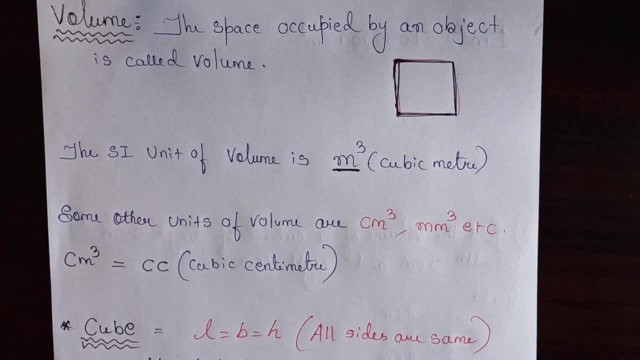 Now if I talk about any solid thing, hard thing, if I have to measure the volume I mainly see here, I am taking the name of solid thing. I am talking about solid Its volume. we measure in meter cube Here. 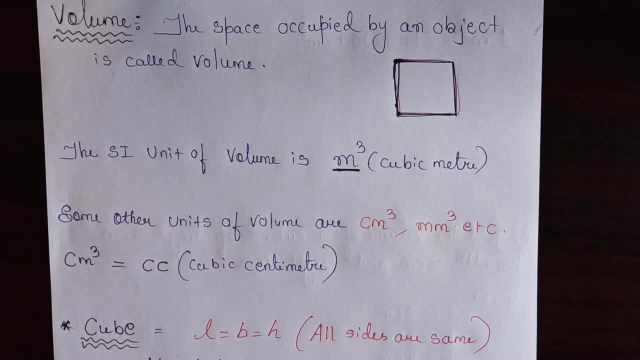 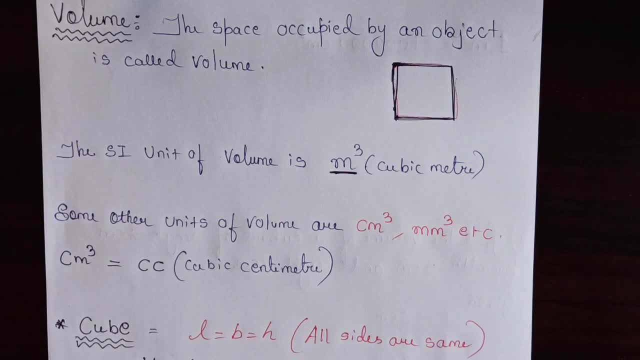 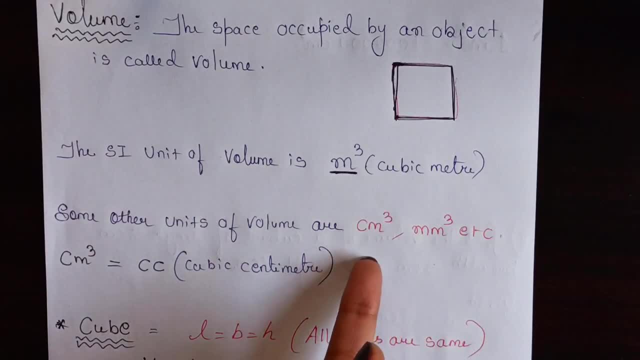 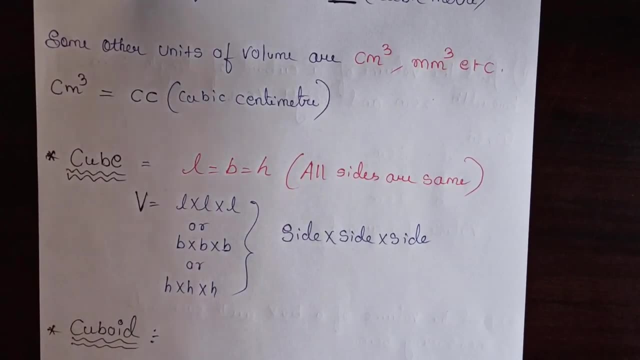 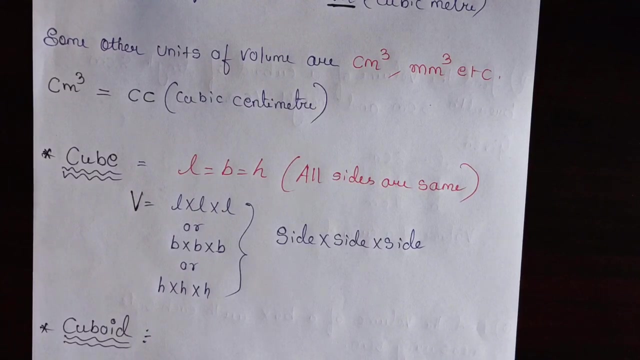 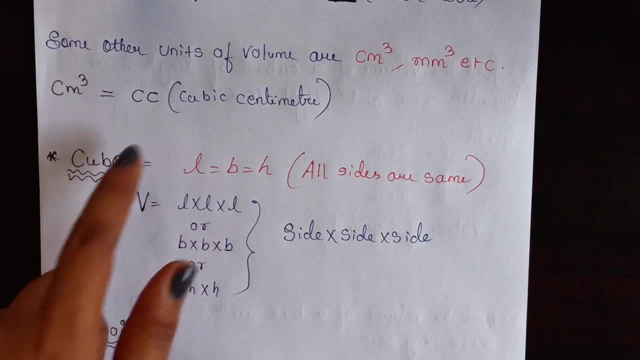 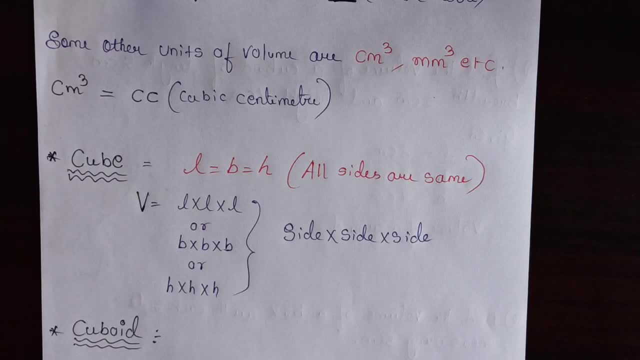 ice cube in ice cube. it is of cube form. its length, breadth, height are all equal. cube is such that its whole side is equal. I will try to make it. I hope it is made, because it is not made quickly. cube word is always made. 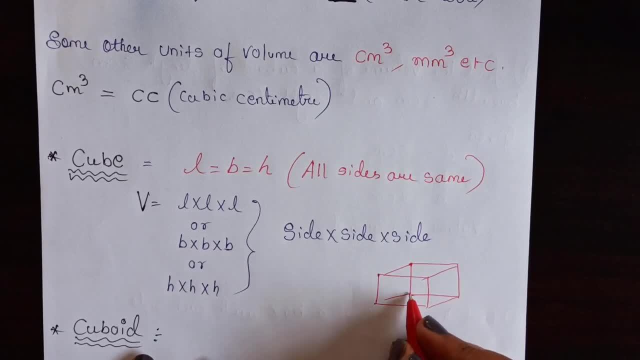 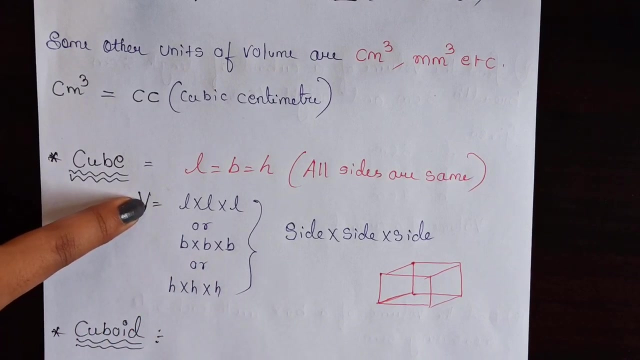 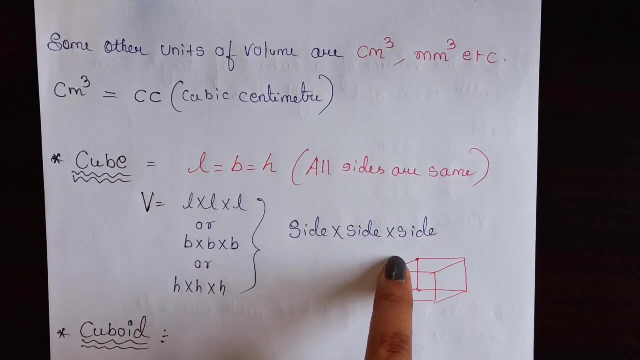 ok, so you guys understand that it is cube. in cube, length, breadth and height are all equal. every side is same and we will find its volume. to find its volume, the actual formula is side into side into side. side into side into side is the formula of: 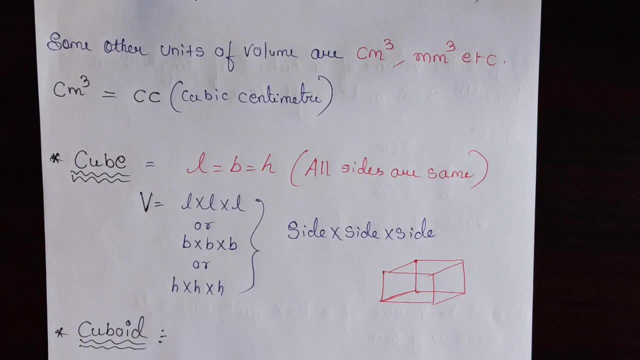 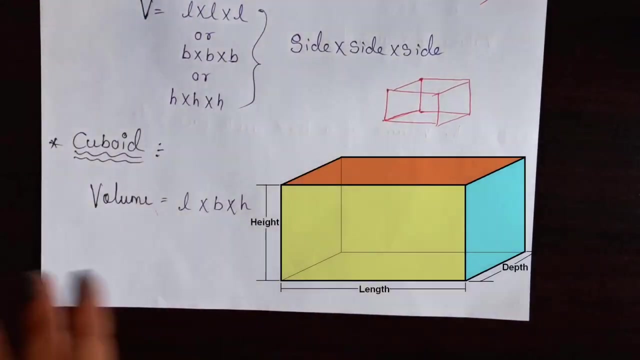 the volume of a cube, for example, we can take ice cube. so many people have studied like this: length into length into length, everything is same. or breadth into breadth into breadth. or height into height into height, everything is same. now cuboid. cuboid looks like this: 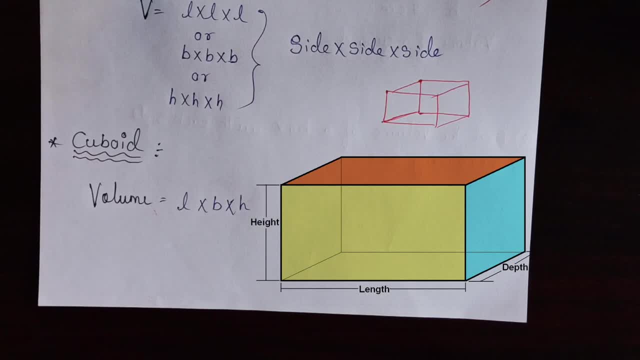 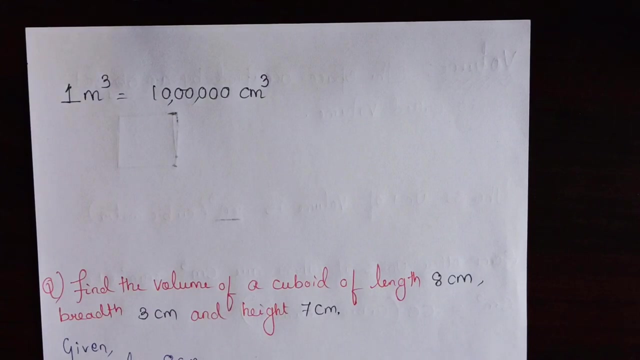 but its length, breadth and height are different. they are not same like cube. so we will include all three, like I mentioned, length, breadth and height in cuboid: length into breadth, into height. so this is what formula of volume of a cube. now we will see some conversion in this. 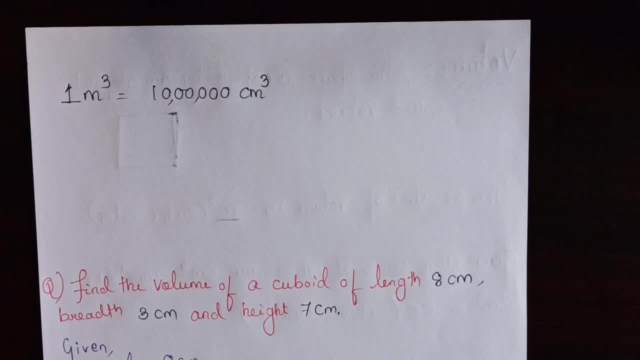 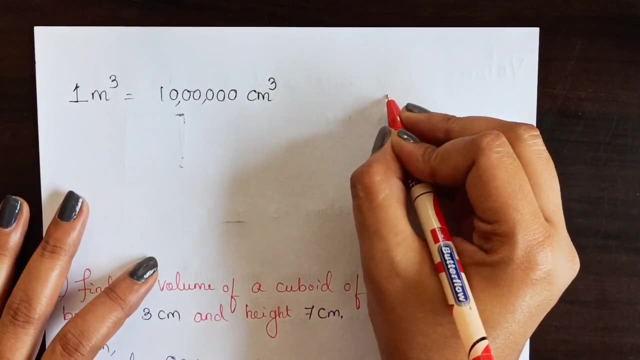 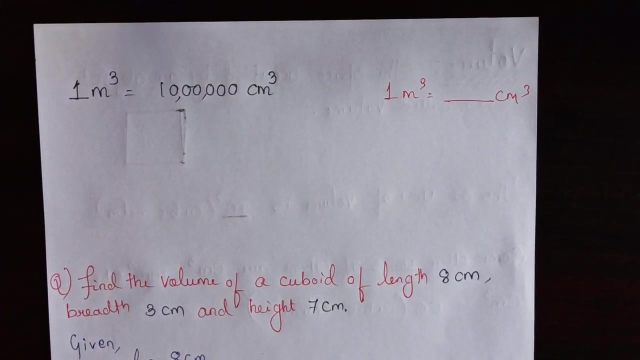 now. now we will see how to convert one meter cube to centimeter. cube means one meter cube, because in exam you will get this question: one meter cube is equal to dash centimeter cube. now, kids actually remember this, but kids forget this. they study so much so they do wrong. 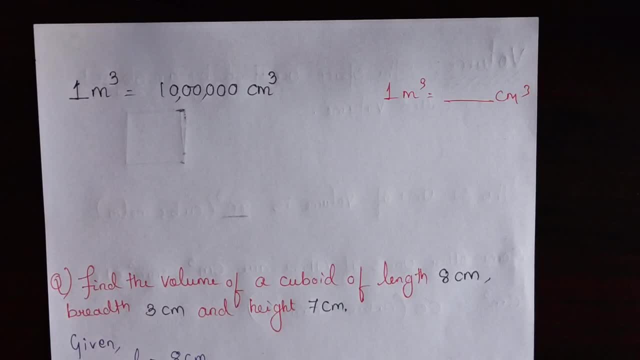 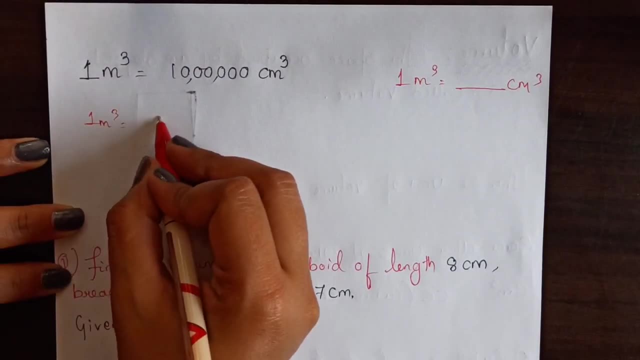 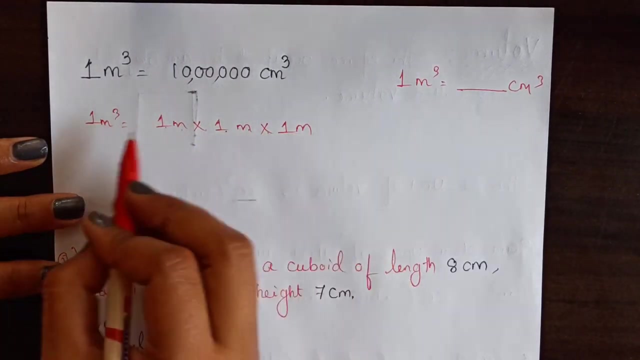 so now there is no tension, because I have told you the trick. we will do the same in this. now see, this is one meter cube. one meter cube means three times meter, like this: one meter into one meter, into one meter. so this is meter cube, this meter cube. 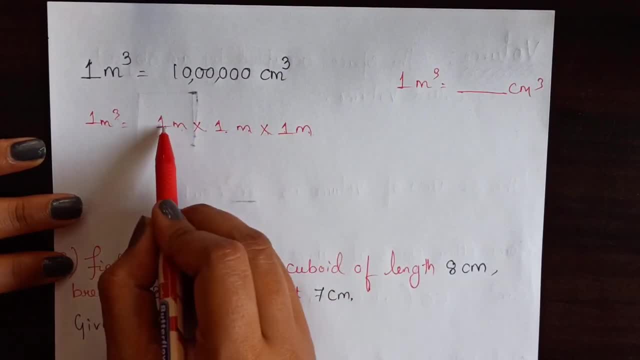 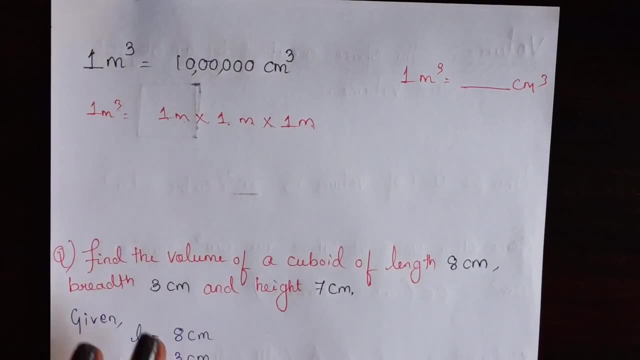 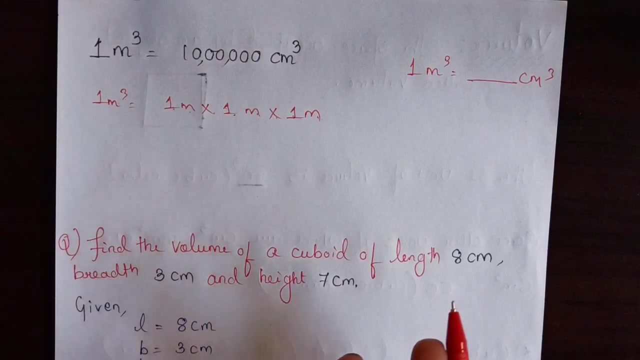 is: m into m into n three times, and one into one into one. no matter how many times you do, the answer will be one. many kids may have doubt. so now you are clear. I can write one meter cube, one meter into one meter now, in which we will convert. 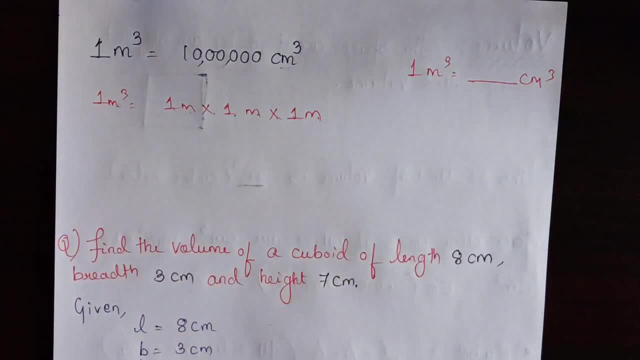 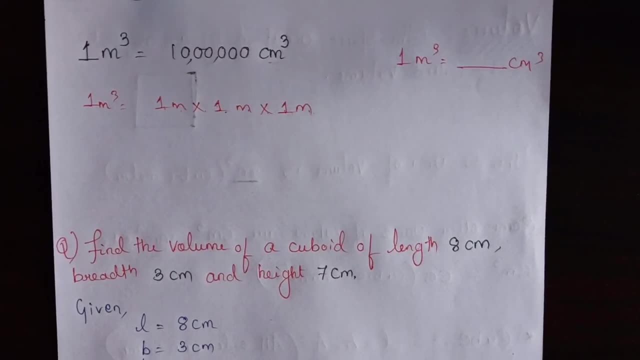 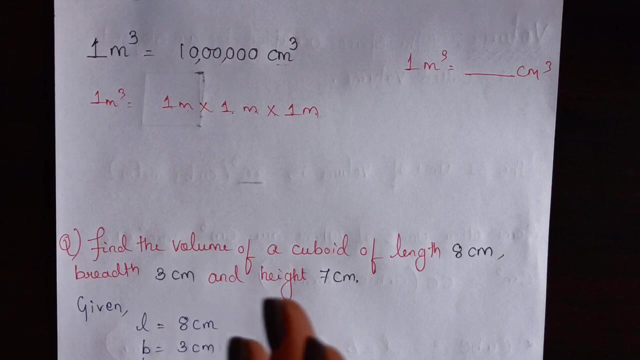 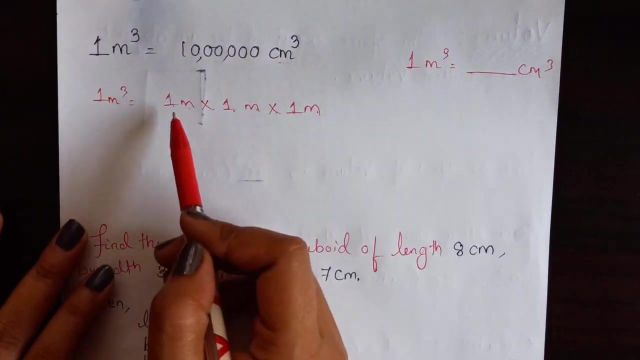 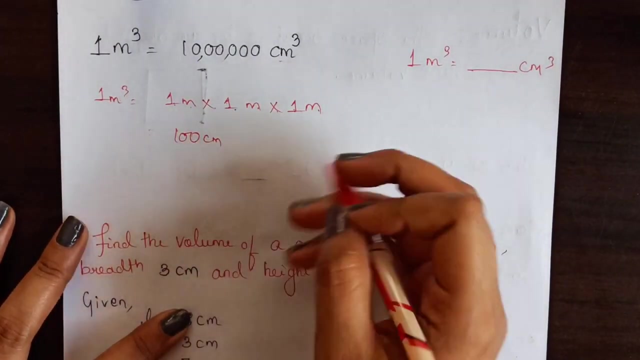 in centimeter. one more thing many kids will skip, then they will not understand. if you will submiss, then they know what you are reading, soanda, so that all your children will think. so now decide, where do you want to passage. consider the mostly visible while, hundred centimeter, and if I make that one like centimeter here, sorry, this is meter. 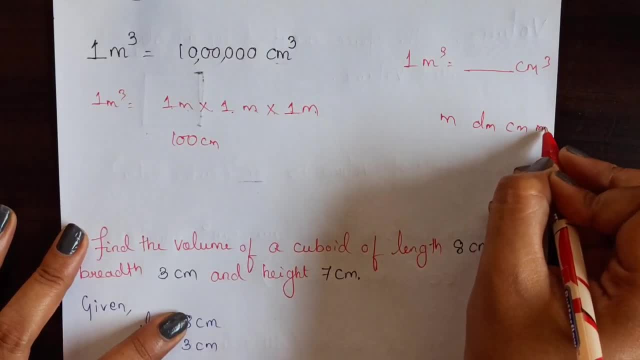 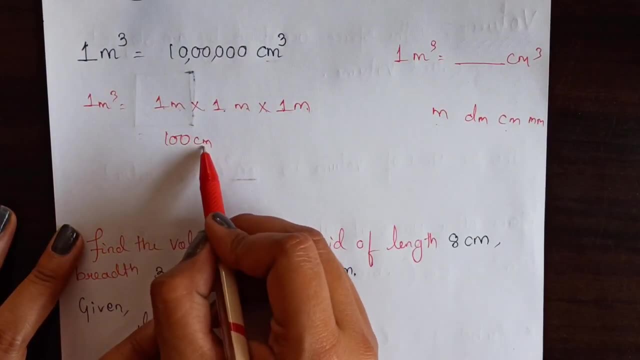 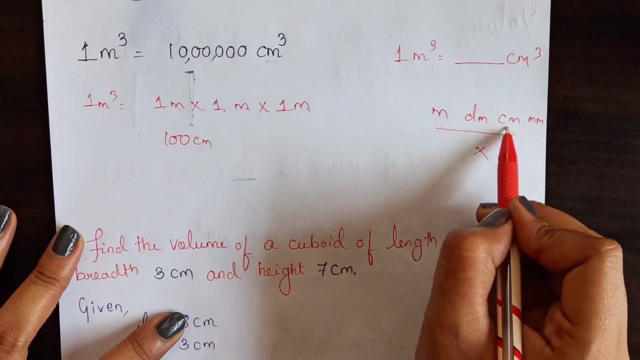 here, then decimeter, then centimeter, then millimeter. just remember this thing. let's convert this. we have to go from meter to centimeter. we had to go from meter to centimeter, so we are going from big to small. if we go from big to small, then we do INTO. how many times will we jump from meter to centimeter? 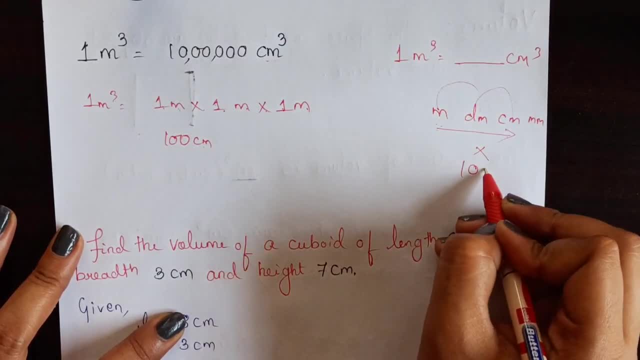 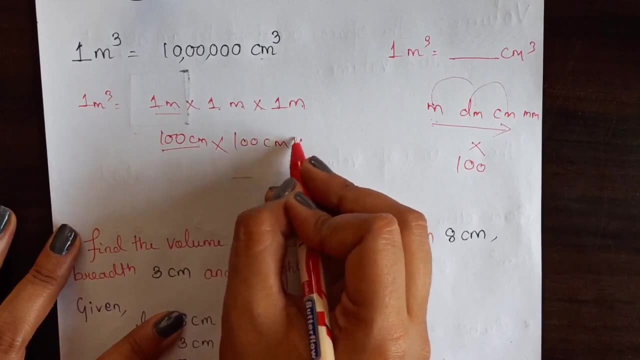 1, 2, 2 times. if you jump 2 times, so with 1, 2 zero is one, so one meter becomes 100 centimeter. similarly, same will go for 5x2 and 5x2. same will fall now 100xX100, anew 100x100. 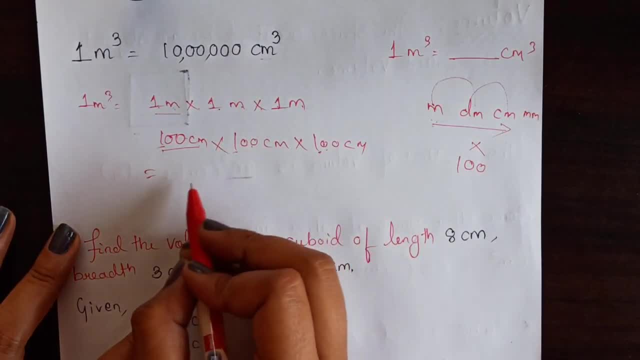 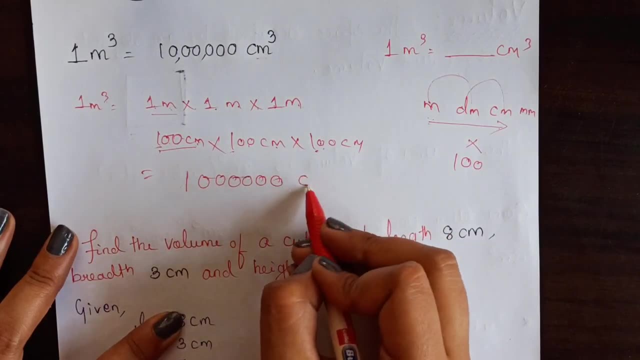 one and tre isn't same". if we match types of centimeter and breath out, new function will costs 0, 0, 0. you'll get same answer. same thing after every count. ok, because we don't give you a reason for saying no to balani means you'll get same answer here. 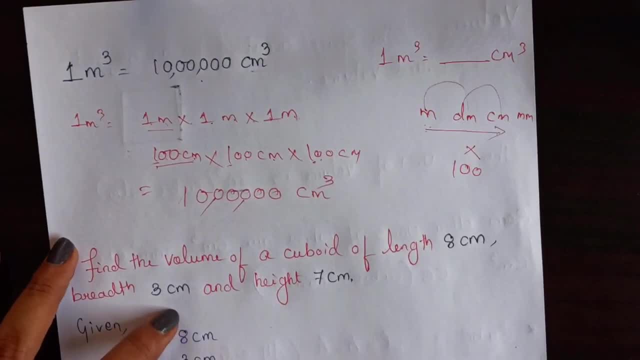 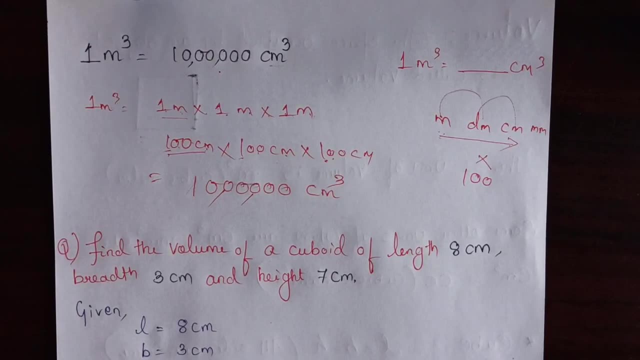 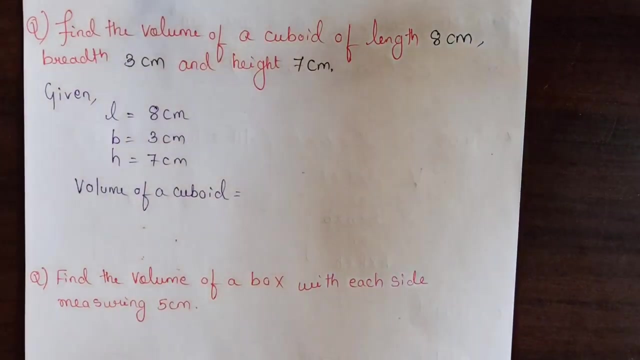 Let's put a comma in it in Indian style, like in Indian place value system. So it is 3, 2, 2 and it is matching. so this way we can convert it very easily. Now let's talk about some numericals. it is very simple: find the volume of a. 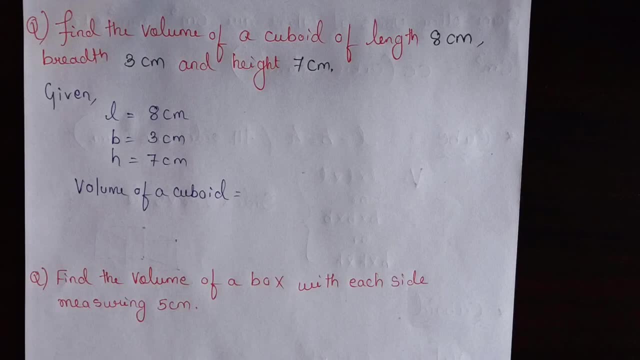 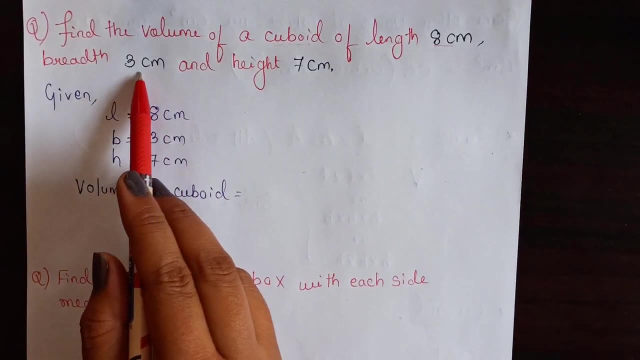 cuboid of length 8 centimeter, breadth 3 centimeter and height 7 centimeter Means we have here a cuboid of length, breadth as well as height. Here it is giving, give, volume. so first given is discussed that how we solve this. 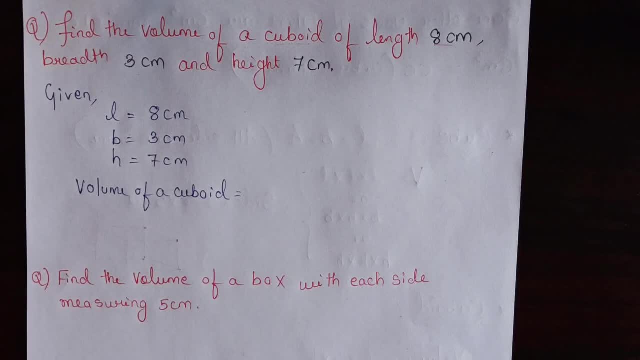 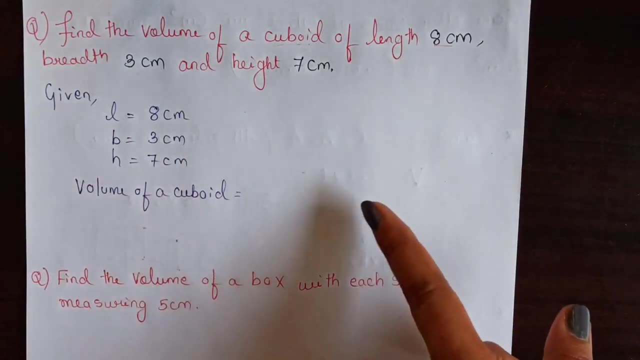 solve numericals in physics, We do the same in maths. First we write: given What is length? Length is 8 cm. Write it Then. breadth 3 cm and height 7 cm. Now how to calculate volume of a cuboid. 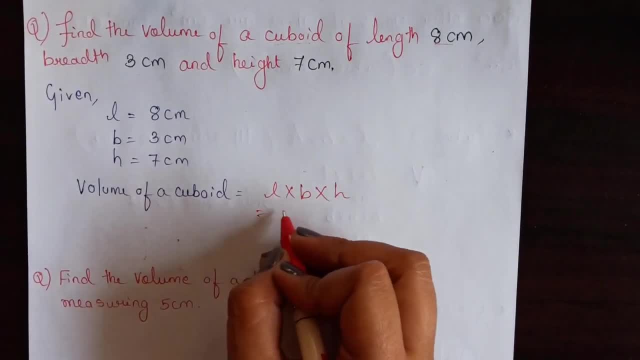 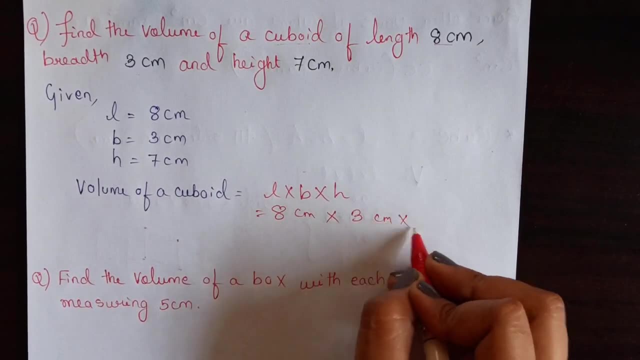 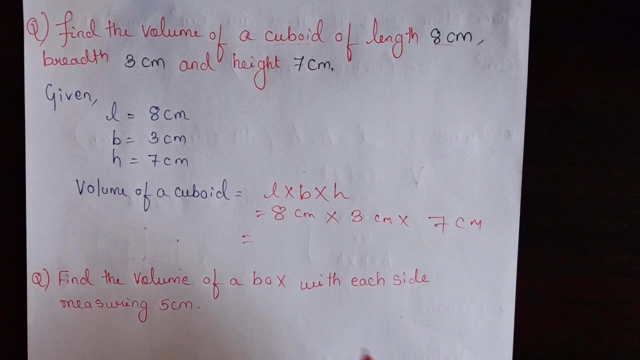 There is a formula behind Length x. breadth x, height. Length, 8 cm. Write it in the distance Or else it will be mixed. And height is 7 cm. Now we will just multiply it. Write down the answer Here: it is cm3.. 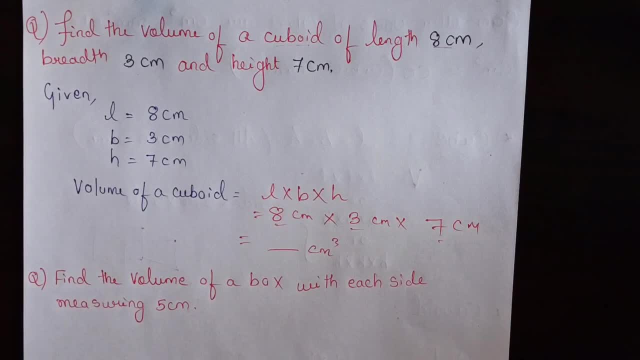 Multiply 8,, 3 and 7.. You will get the answer Now. This will be 168 cm3.. Let me check. Yes, 168 cm3.. So this was a very easy question. It will come now To calculate volume of a cuboid. 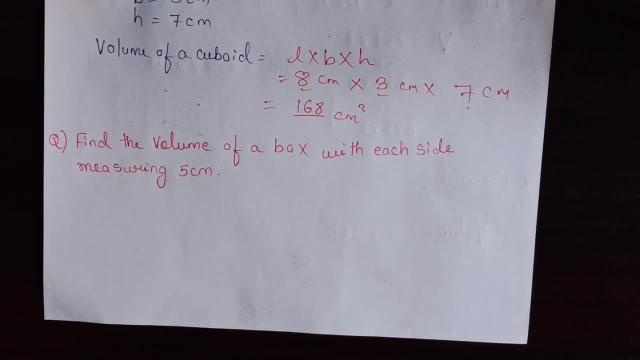 Now We will find the volume of a box, with each side measuring 5 cm. Now look at this question. He is talking about a box, But he has not mentioned anything like whether it is a cube or a cuboid. He just said: find the volume of a box. 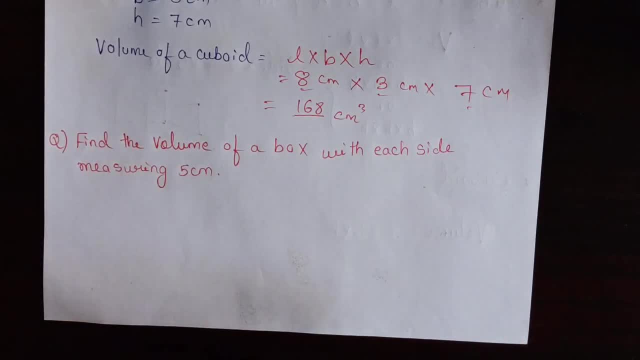 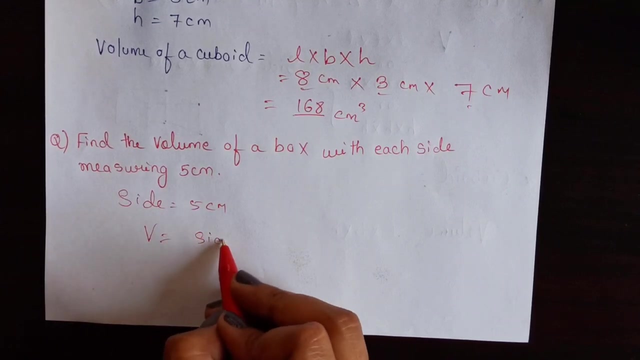 with each side measuring 5 cm. Whose side is 5 cm? Now tell me Which is a solid figure, whose volume is same on all sides. Which is a cube Means here, each side is given 5 cm of cube And he is asking to find the volume. 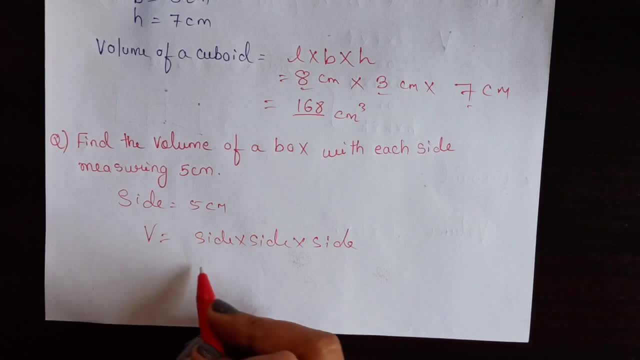 So what is its formula? Side into side, into side. Now write 5 cm into 5 cm, into 5 cm. So this will be 125 cm cube. So this will be 125 cm cube. This is how the question comes. 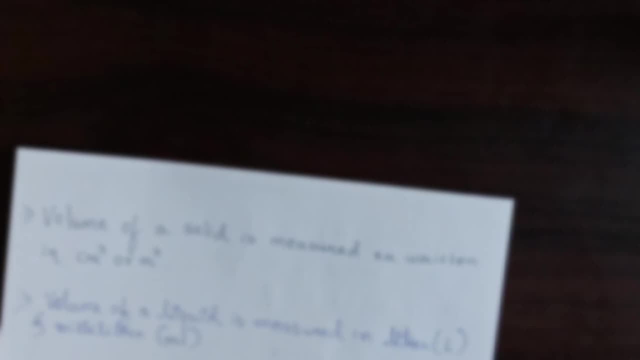 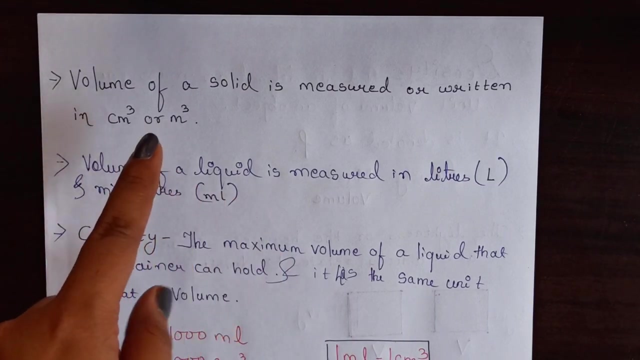 It is easy Now. next, Now, When I was studying: If we measure the volume of a solid, Then we write it in cm3, m3.. But if I measure the volume of a liquid, Because we will only measure the volume of a liquid- 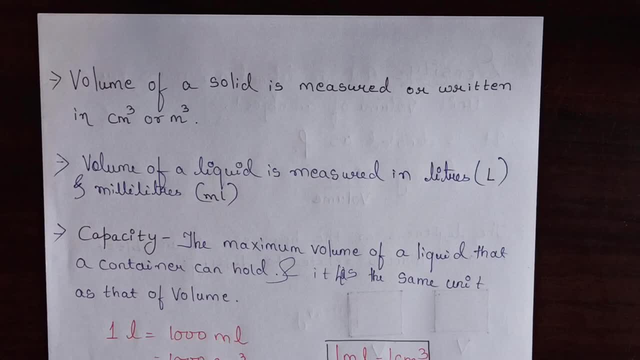 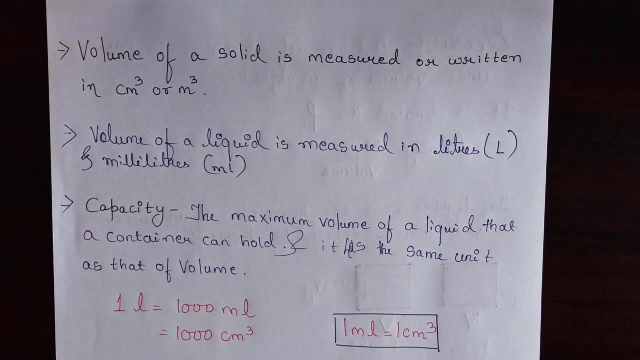 Ok, So when we measure the volume of a liquid, Like take oil, Like milk, Like water, Like cold drinks- See, when we go to buy cold drinks- Then it is written in the bottle. It is written that it is of 1 litre or 1.5 litre or 2 litre. 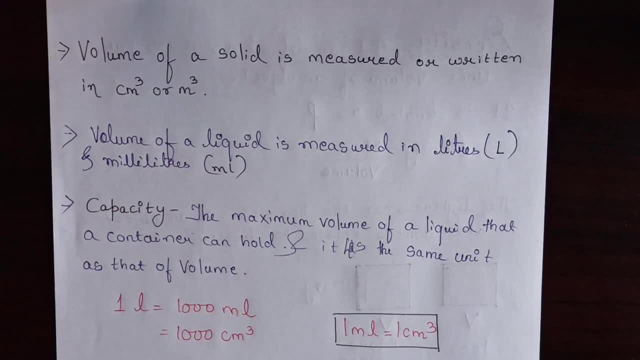 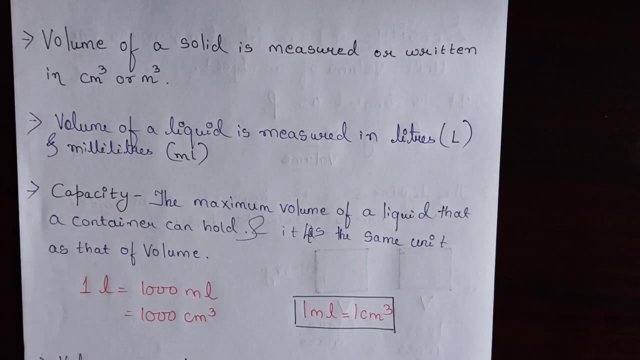 Ok, So volume of liquid is actually measured in liters or millilitres. So volume of liquid is actually measured in liters or millilitres. Mainly, these are two things In this. we measure either in litre or millilitre. Now we will talk about capacity. 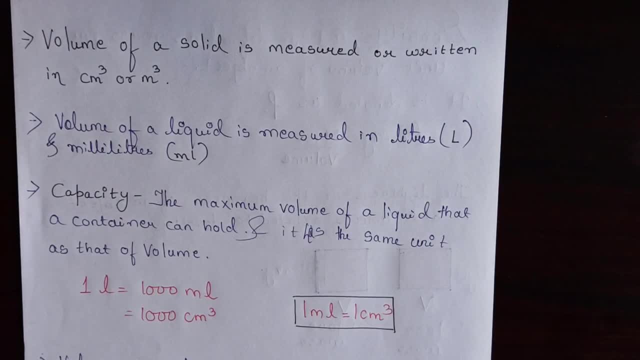 Now we will talk about capacity. If I talk about any container, If I talk about any container, Like we talk about the bottle of cold drinks, Ok, Any bottle or any container. How much liquid can hold? Maximum volume Or amount? 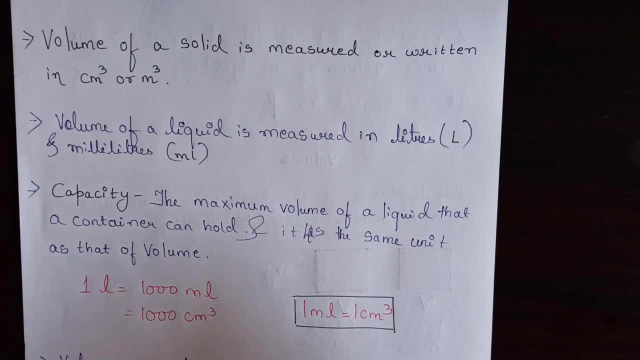 Or quantity, Or quantity of liquid a container can hold. How much and in what quantity a container can hold liquid. That is called Capacity And the capacity can be seen like towards 2 litre bottle, 2 litre liquid can comes in it. 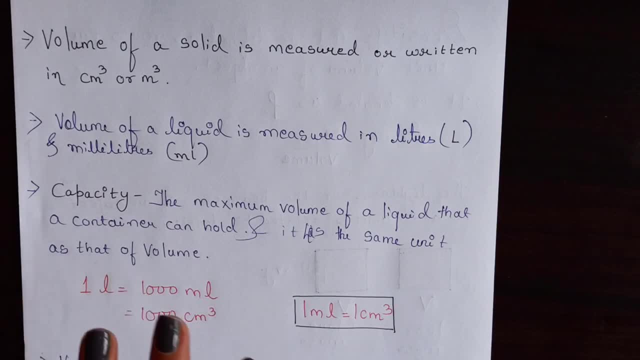 2L cold drink can comes in it Normally liquid's or bottle. So the capacity of the bottle is equal to That is equal to volume of the liquid which can be present in it or which can hold it. and as I told you earlier that if we measure the volume of liquid then we write it in liter and milliliter. similarly, 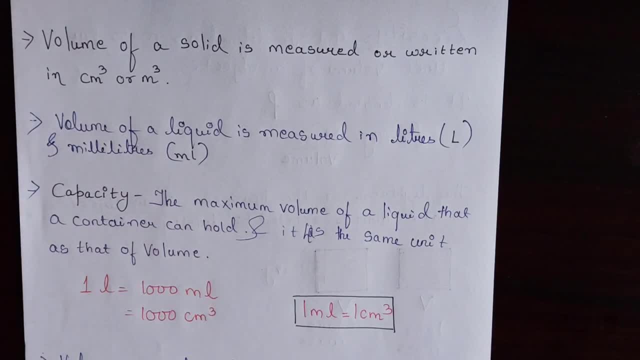 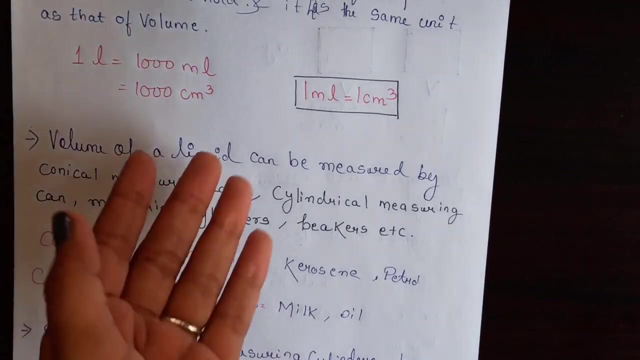 capacity also has the same unit, as if we write the unit of volume in liter and milliliter, then we write the capacity also in liter and milliliter. why? because that too is measuring volume. only now we will see the relationship between liter and milliliter. so one liter. 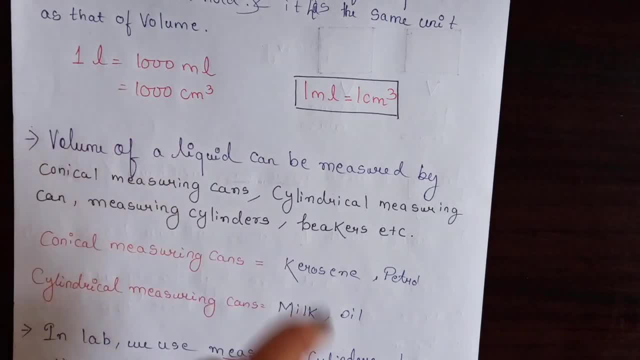 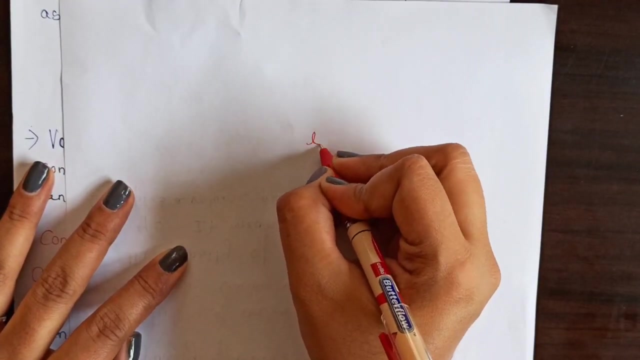 is 1000 milliliter. yes, one liter is 1000 milliliter. this is fixed. and if you want to see it, like I told you earlier, in this type, which I told you about meter and centimeter, so what happens in this, think that here is liter. so, from liter to milliliter, you can see the difference between. 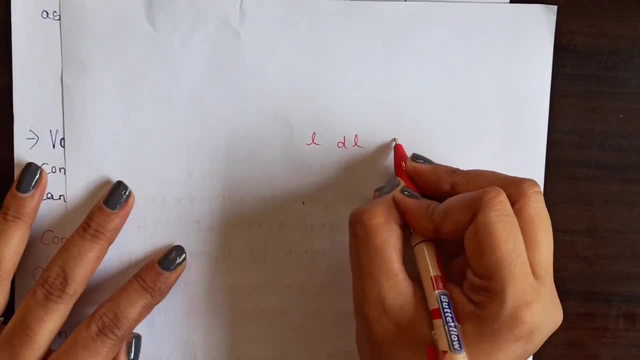 liter and milliliter. so what happens in this think that here is liter to milliliter, so from liter to milliliter. you can see the difference between liter to milliliter. so from here I will go to a small unit, so one will be deciliter, then centiliter, then milliliter, and if I go here then it will be decaliter. 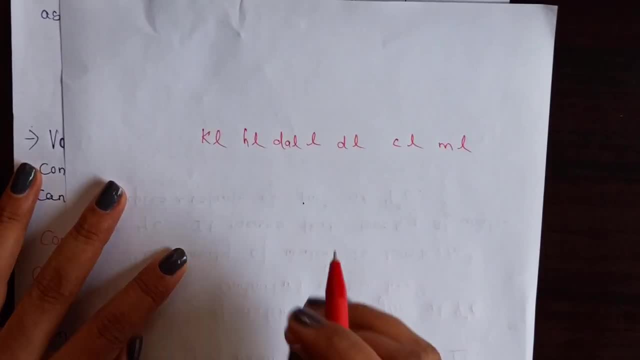 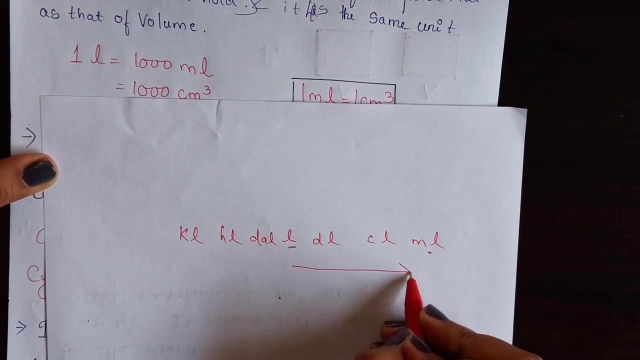 hectoliter and kiloliter. now we are talking about the relation of liter and milliliter. so see, here is liter, here is milliliter. so we are going from big to small and I have already told you that, if we go from big to small, 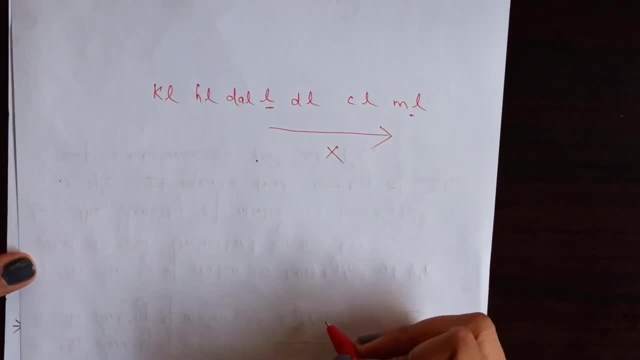 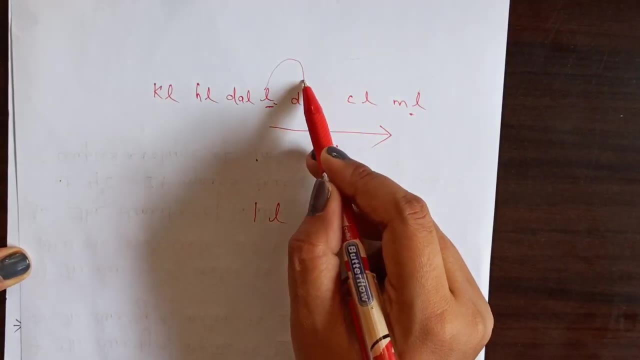 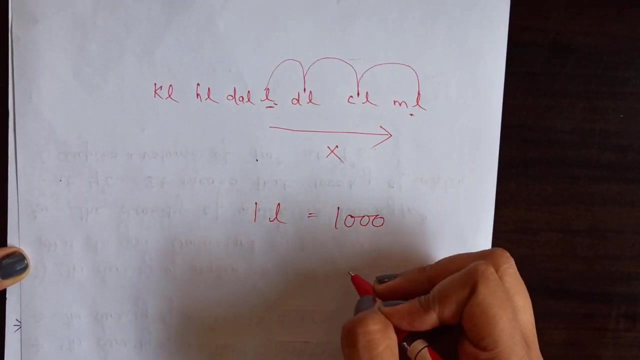 while measuring. so what do we do? we multiply there. now how much to multiply I have to do? one liter, so go to milliliter. by liter, so go by jumping one, two, three. the number of times we jump means three times. we have to put three, zero with the one that becomes milliliter. 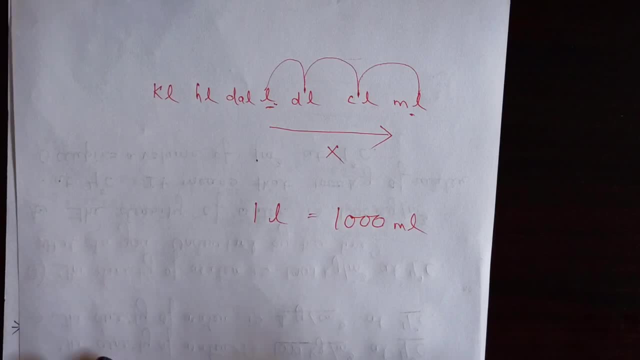 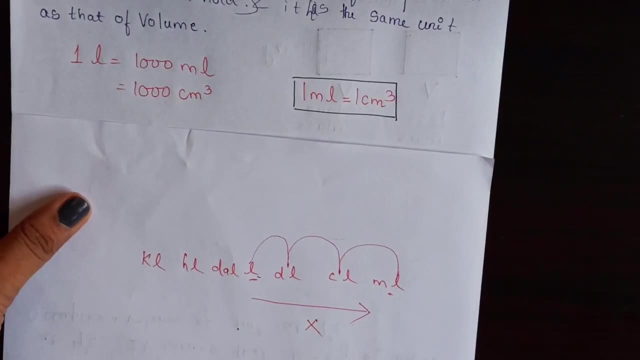 so one liter is equal to 1000 milliliter. here I have told you again the method, and here I have written directly. now there is another thing: this milliliter, milliliter is equal to centimeter cube in both the volumes. so this is the number of liters, and then this: 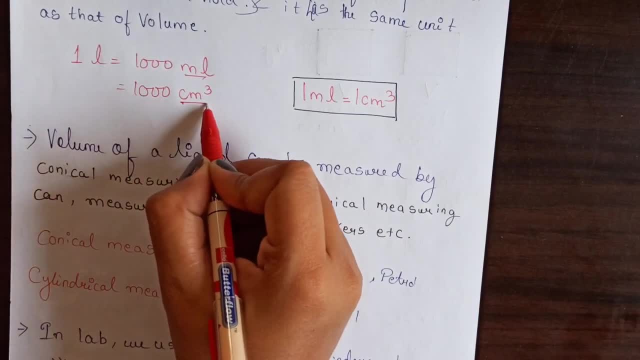 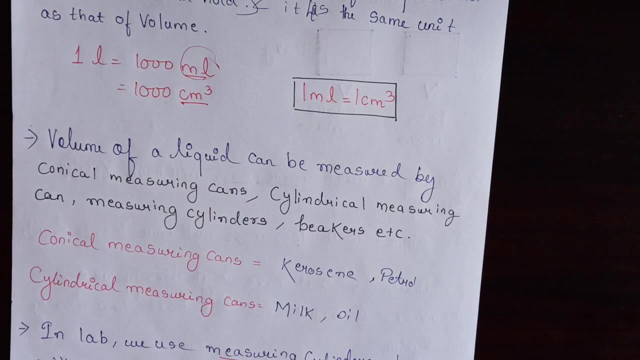 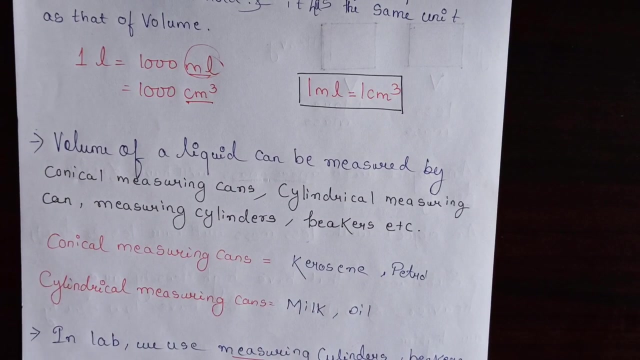 so milliliter and centimetre cube is same. so in many places milliliter and centimetre cube is written, so both are equal. so don't get confused in this. now, if I talk about if we measure volume of liquid, then in which way we will measure it. 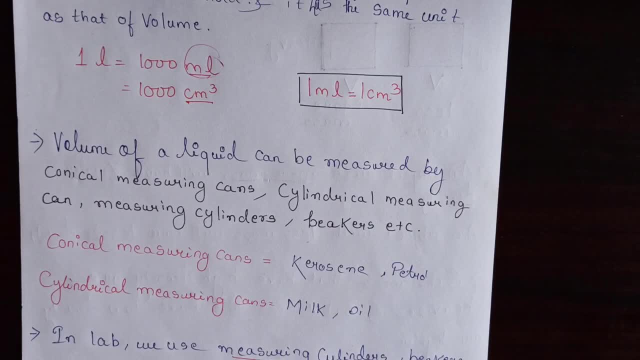 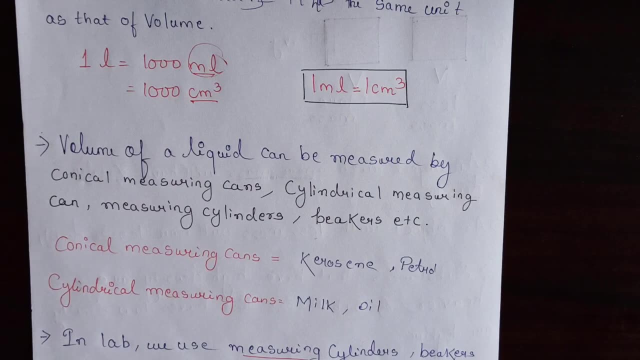 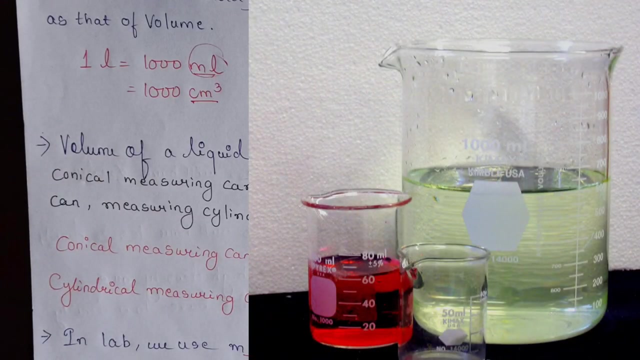 normally what happens? to measure volume of liquids we need container of different capacity. obviously we need container, as you have seen earlier on the side. I will give you a picture of beaker here you can see beaker, this beaker. actually we use it in lab to measure volume. 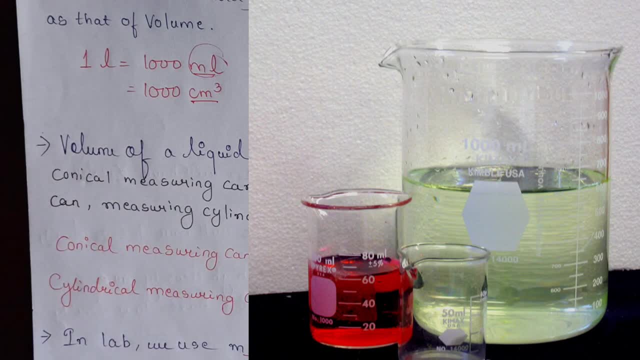 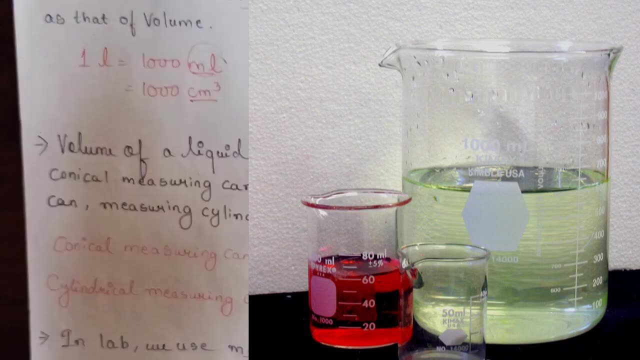 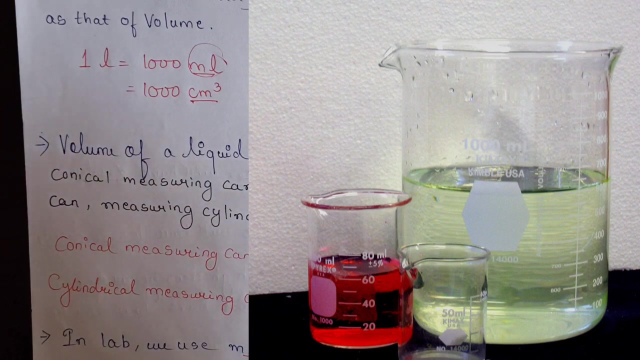 how much milliliter liquid I need. centimetre cube liquid I need. whatever we use beaker. how much quantity chemical or water we need. that is graduated beaker. graduated means scale is made there. number of measurements will be mentioned here, so it is seen here. 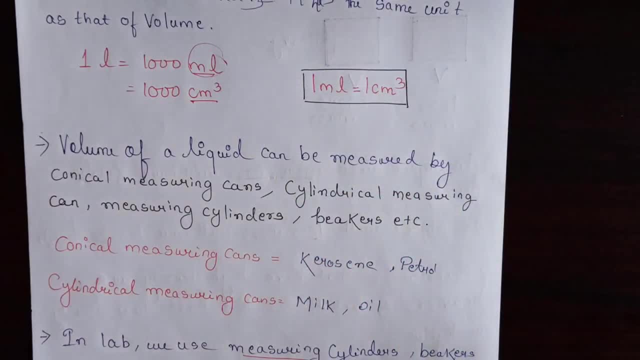 so same as just in lab. we will not measure volume in different cases we will measure the volume of liquid, like when we go to buy milk, then you have to mind you go to buy the packet milk, but normally when we go for buy the milk so he measure. 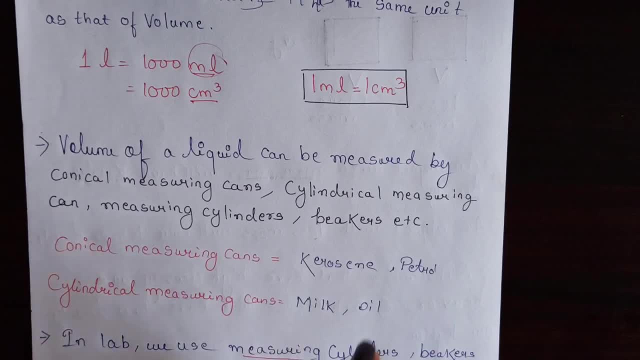 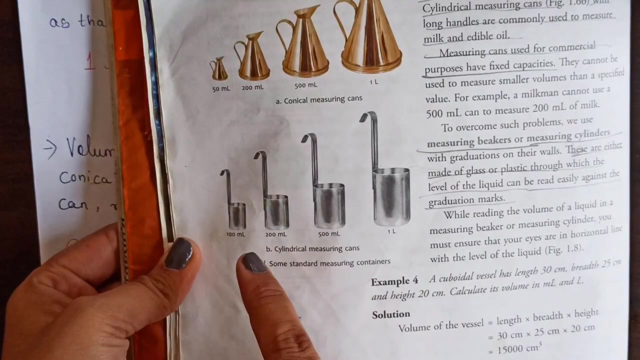 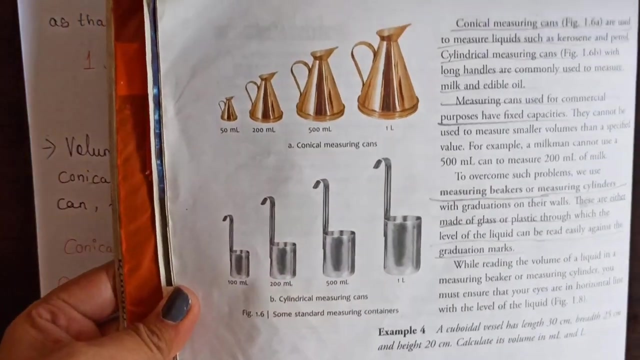 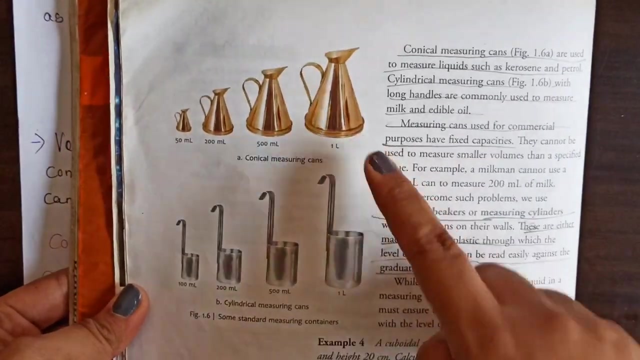 when he gives milk. that is called cylindrical measuring can, which is used to measure the quantity of milk or the quantity of milk kept in the container, is called cylindrical measuring can. You can see in your book. there are photos in it, like this photo is made in the book. you can see it in your book. you will see it well, and I will give it on the side too, like photo. yes, look here. you can see this. this is a cylindrical measuring can. okay, this can measures the quantity of milk and is given similarly. if you say this too, it is a measuring can, but look at its shape differently. it also measures the capacity of the liquid. it will also measure, but the shape of both is different. this is a little cylindrical measuring can. 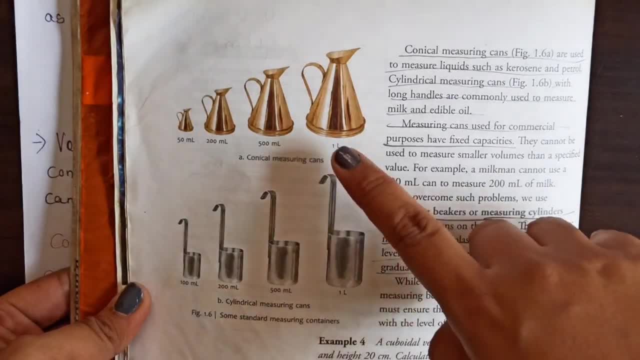 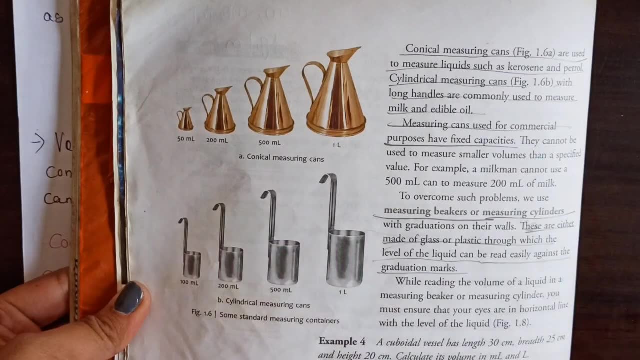 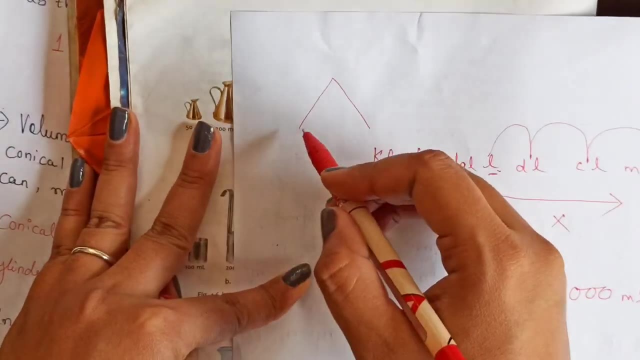 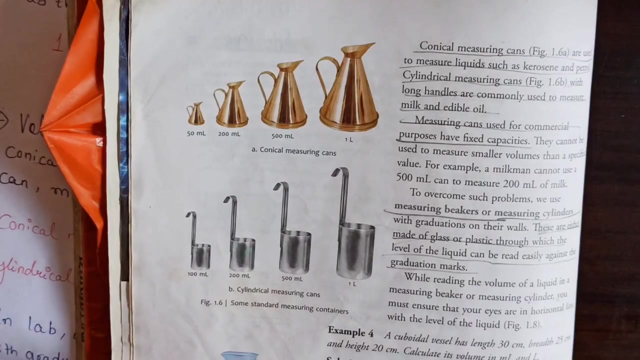 it is in cylindrical form, so its name is cylindrical measuring can. it is in a little conical form. conical shape means this type of what you see, right, it is called, like you have to mind, the volcano. the volcano, you must have seen, it is a little like this, it is like this, it is like a mountain, so this is also a little conical shape. okay, so look here, this is a conical shape measuring can. this is in cylindrical form. so what is the work of both? to measure the volume of the liquid. 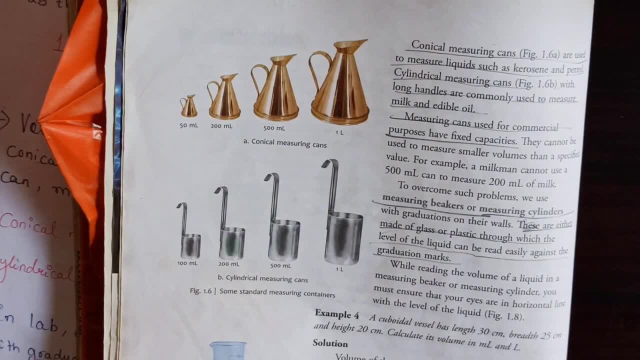 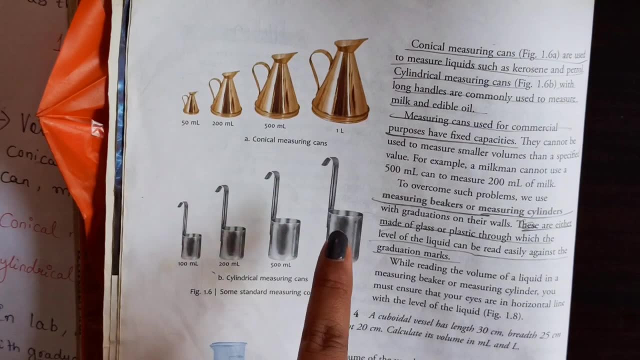 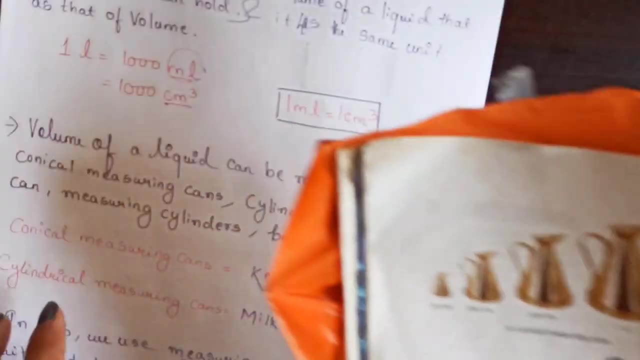 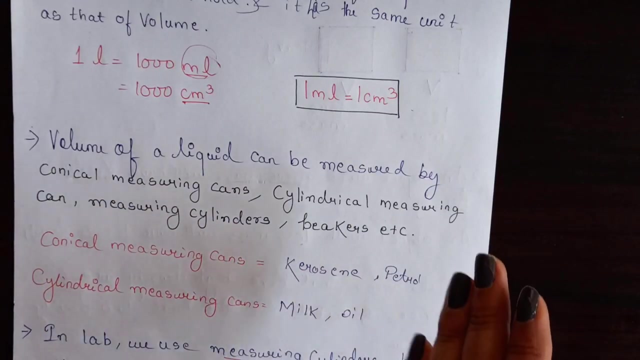 okay, normally, like in books, like what is given, normally it happens that we if we have to measure the volume of the liquid, if we have to measure the volume of the oil, then look at it. this type of mainly is used but for kerosene petrol, normally this conical measuring can. it is used a little and there are many more, like I have written here. measuring cylinder. you will see in the book and here I have given a photo on the side. measuring cylinder. it actually uses the exact volume. 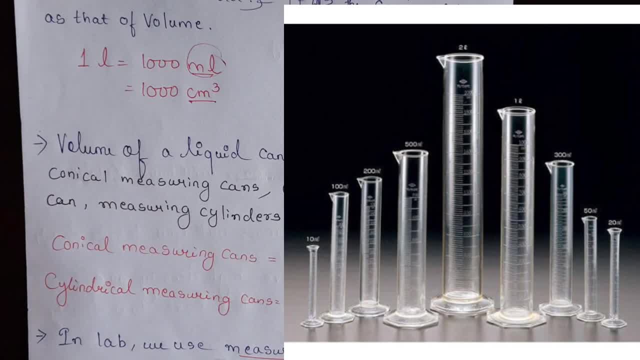 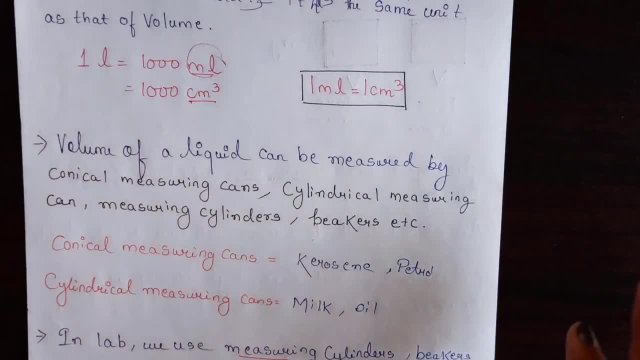 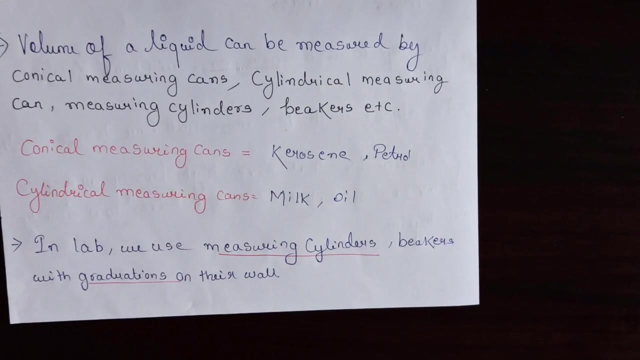 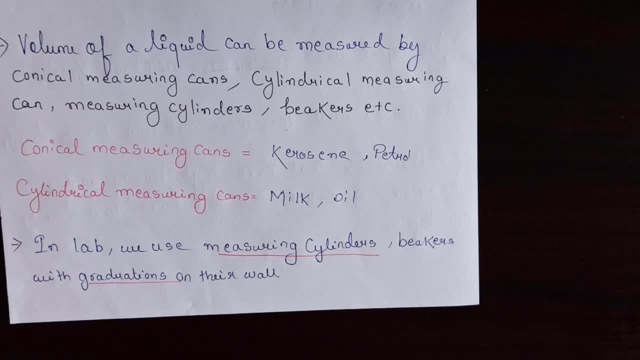 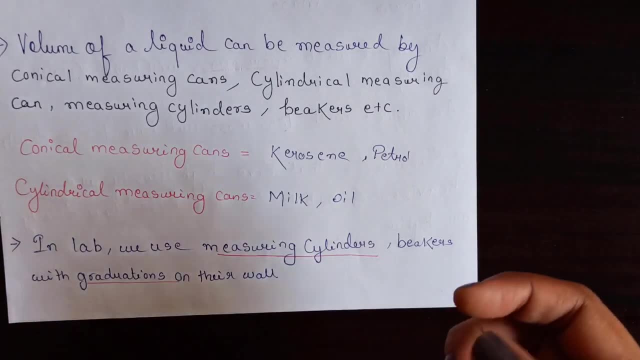 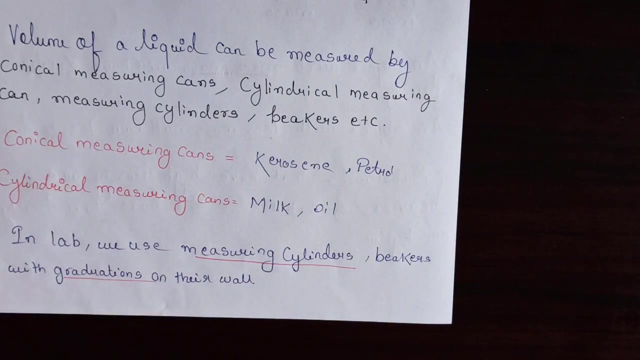 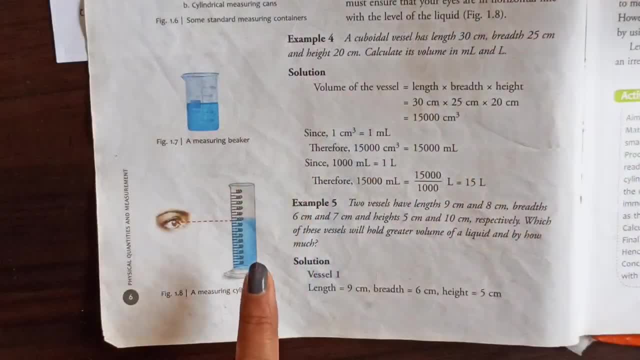 It is looking good. Just wait, Okay, as you can see, this. This is measuring what Cylinder. See, it has a scale in it. It has graduations on its wall. It is like from zero. Here it is given in 10-10 difference. 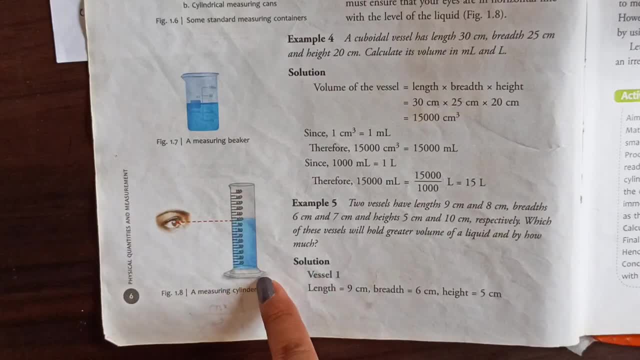 It is like from zero. It has a very simple reading, So it has a scale in it. We can say that we can measure exactly. and take the liquid. It is actually used to measure the volume of a liquid. See, there is a measuring beaker here. 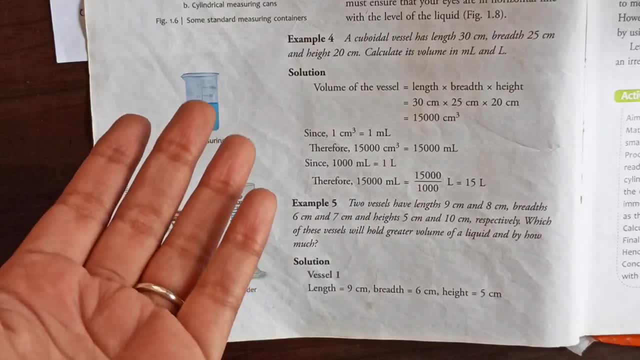 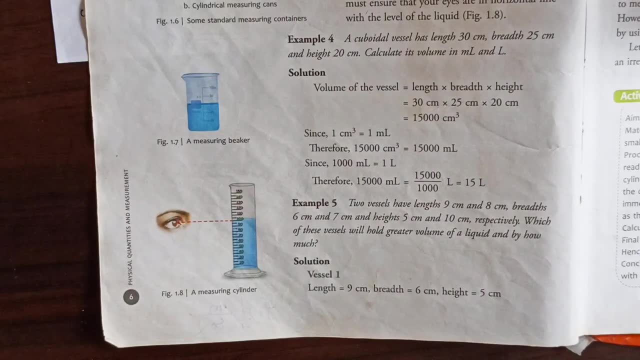 This scale is also made here. You can see it from near. It will be clear, So it has the same scale in it. It has graduations on its wall So that we can measure the volume properly Whenever we do some reactions. 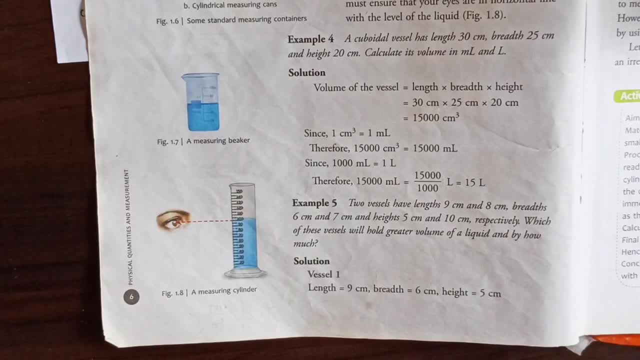 like chemistry. mainly, it is very good. Now, 6-7 year old children do not do it by themselves. When we were in 9-10, we were not taken to practical lab, I don't know why- In class 11-12,. 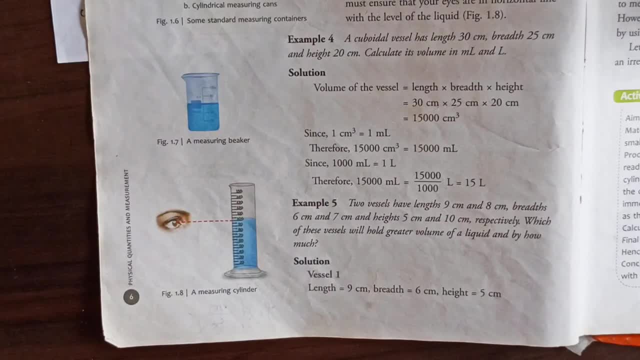 we did everything by hand, But I don't know outside children are taken to the lab. Tell me if you show the whole experiment in the lab or not. But whenever we do experiments in chemistry in higher classes, we measure the exact things. 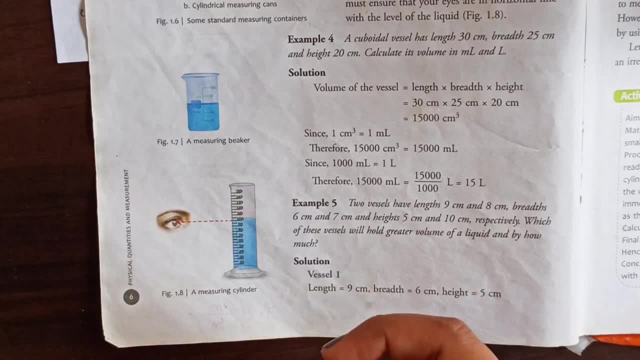 Exactly. If you want 20 ml of water, it will be used in experiments. If it is more or less than that, then the reaction can be wrong. So we can use all these things to measure the exact volume and use it in experiments. 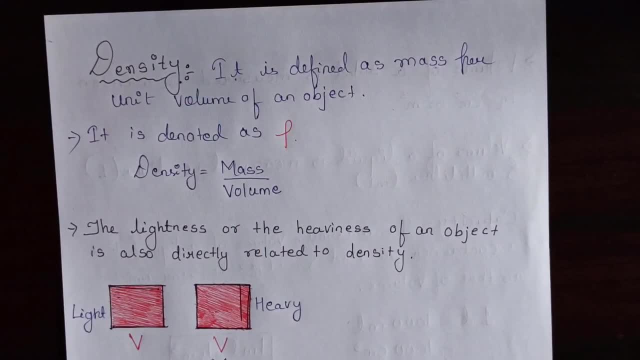 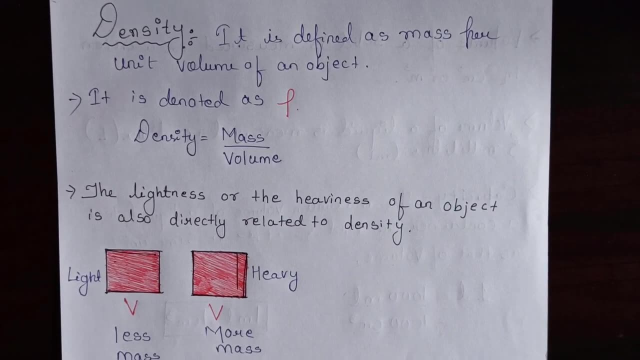 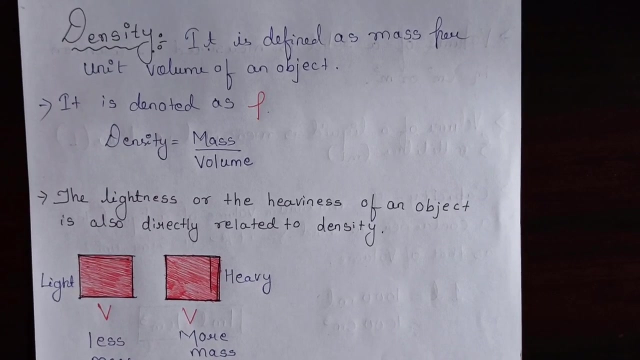 Now, after this, the topic is measuring the volume of irregular solids. So for that I also need a measuring cylinder, which is not available at the moment. We will do that, Or I will put a small video so that you can see and understand. 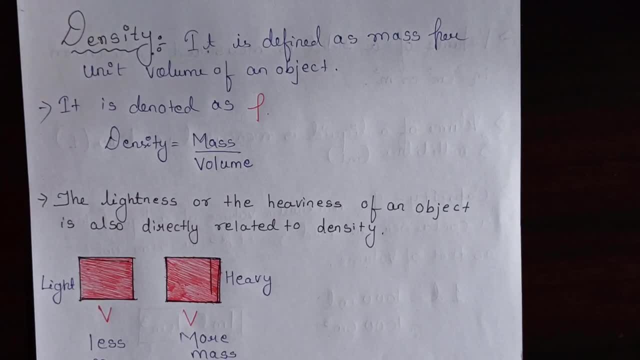 Ok, So Density. Now see what is density. Density is very easy. If you want to understand what is density in a simple way, just remember one formula for density: Mass by volume. You know the meaning of mass, I have told you. 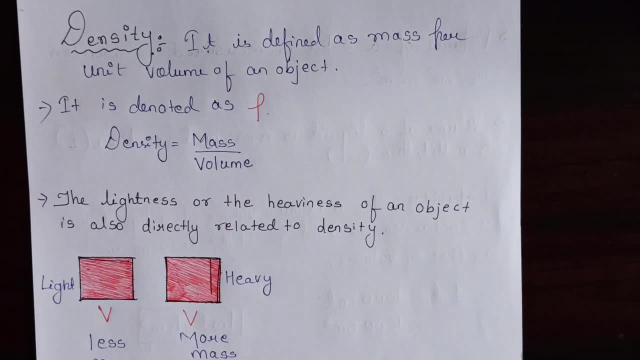 You also know the meaning of volume. So density is mainly defined as mass per unit volume of an object. I have already told you that in the language of physics we can use anything, anything, anything, anything, anything, anything, anything. 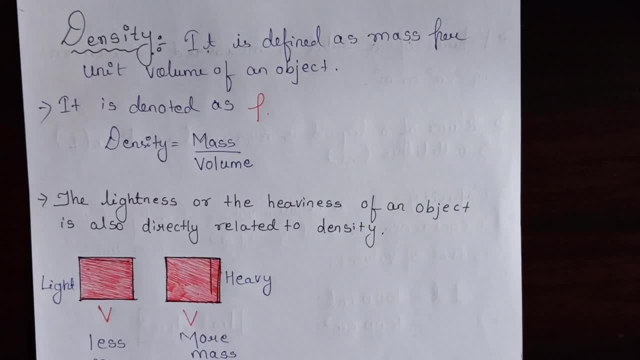 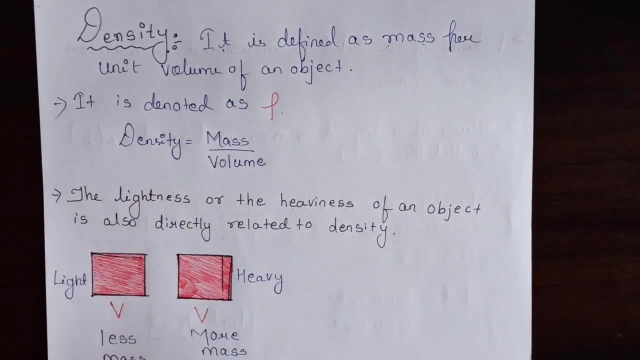 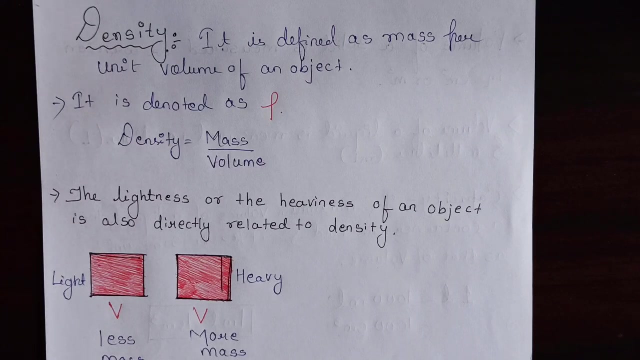 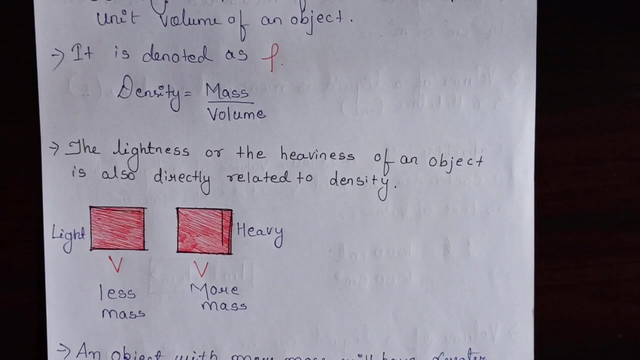 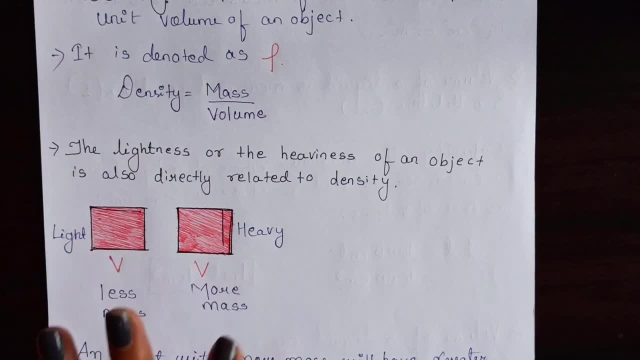 you all know the meaning of volume. if I have two objects, both have same volume, but one looks heavy and the other looks light. so whether I write light or heavy here, both have same volume. but if this one is heavy and this one is light, so the one which you think is heavy 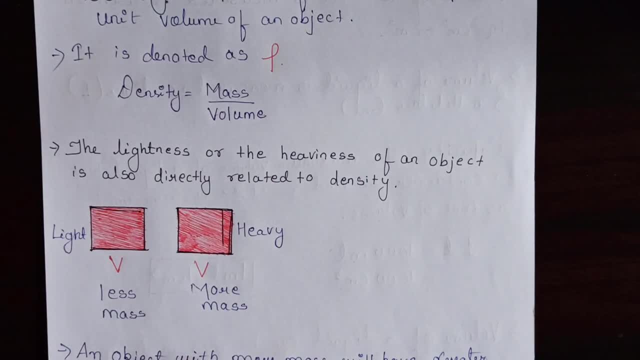 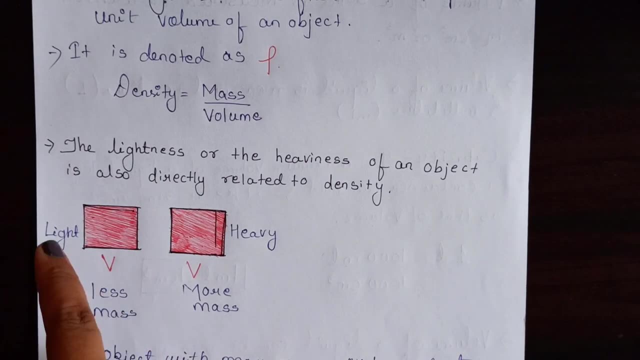 means it has more mass. if it has more mass then it will be more in density. see here: if it has more mass, then it will be more in density. similarly, for this object I have written light here. light means it will be light. light means it will be less in mass. 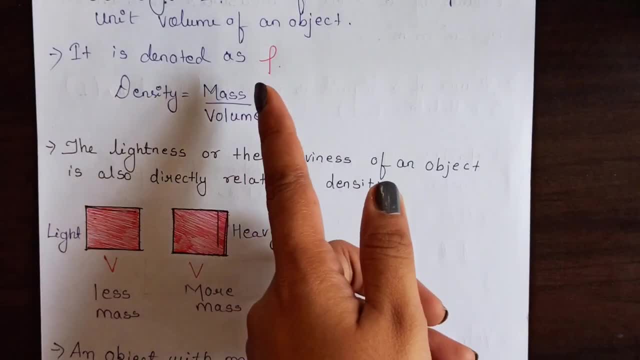 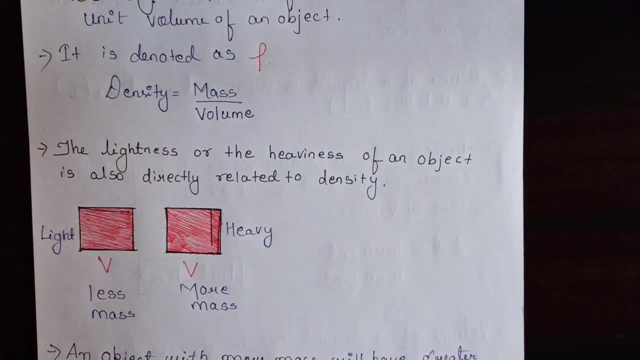 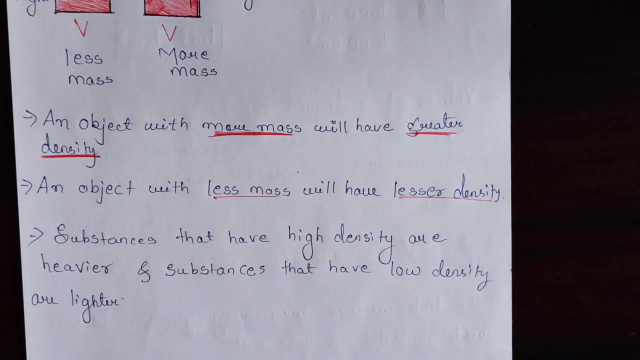 if the mass is less, then the density will be less. if the mass is more, then the density will be more. if the mass is less, then the density will be less. so for that, look here. I have written something like this, because this can ask you a question. 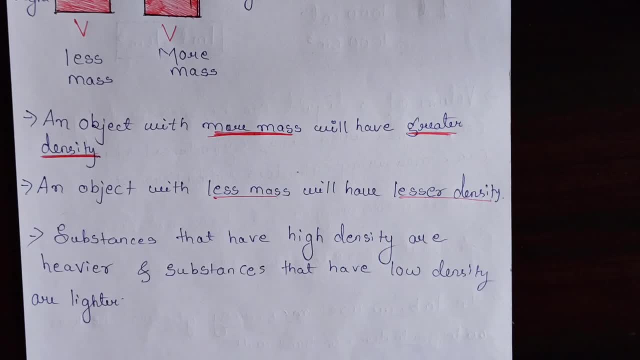 that an object with more mass. if an object which has more mass, what will be its density? obviously it will be more greater density, opposite of that, an object with less mass. if an object has less mass, what will be its density? density will be lesser. so a substance, or any substance, 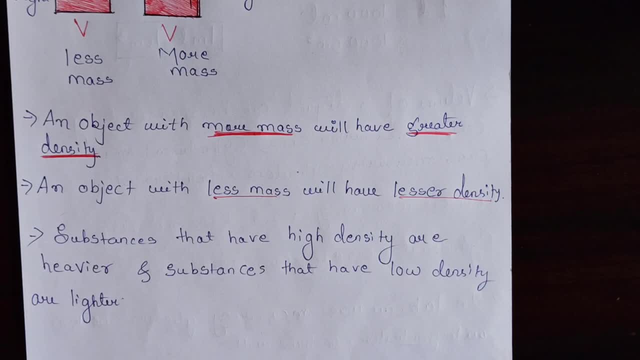 if any substance has more density, then I can say it is heavier, or you can say it is opposite of that. if an object is heavy, that means its density is more. so I have written something like this. it is very simple. you can do it easily. it is not that hard. 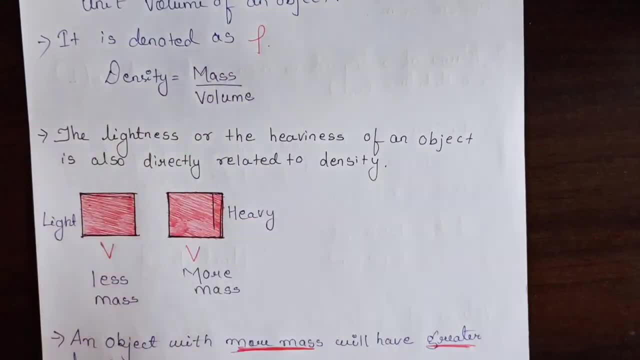 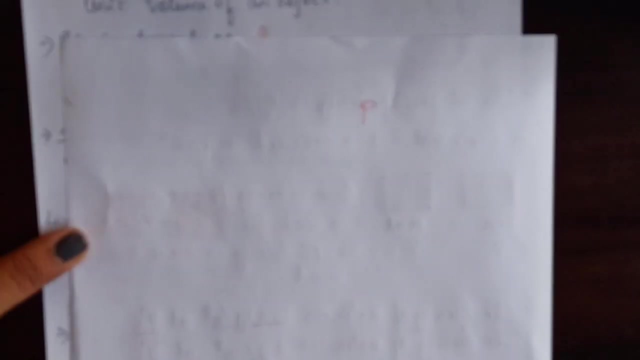 one more thing which is left here. this is RHO. it is called RHO. it is a greek letter and we write it like this. I will write it again. I will write it here. see how we write it. many children make it P. don't make it P. 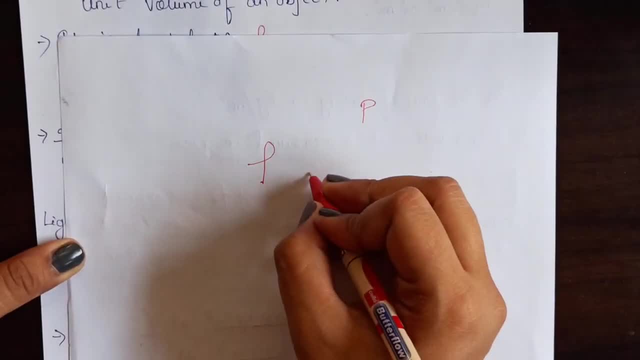 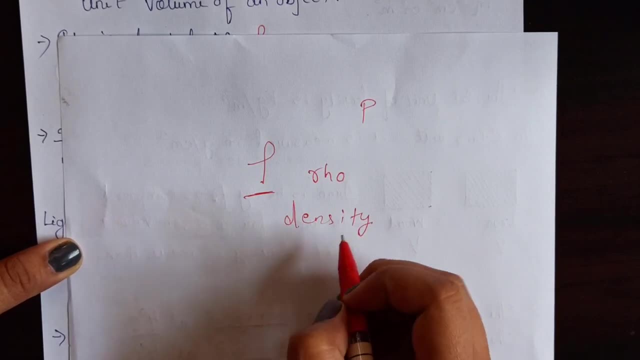 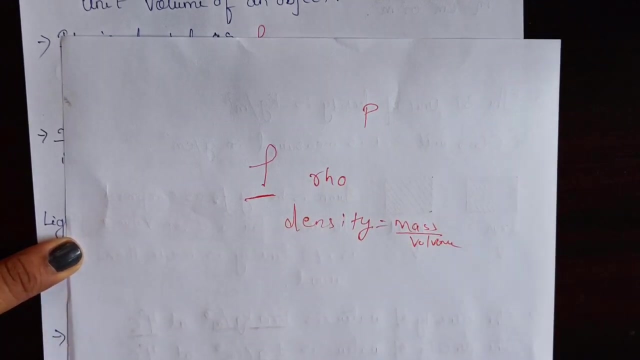 don't make it P, do it like this: RHO. so this is a symbol which we write for density. and what is the formula of density? it is mass by volume. now, if I write it in every place using some symbols, then how will I write it for density, RHO. 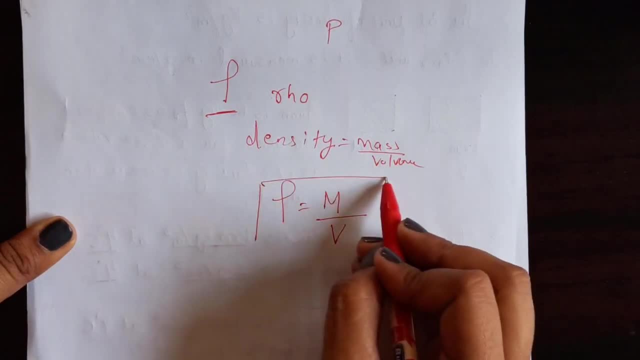 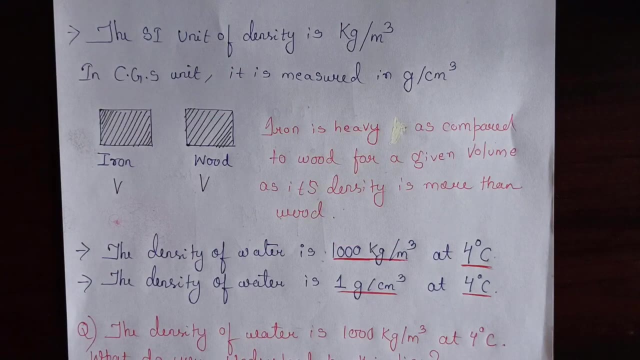 for mass M, for volume V. so this is the formula of density. now, now, now we will see its SI unit, because before this we have seen the SI unit of many things, we have seen the SI unit of volume, we have seen the SI unit of area. so how can we leave the density? 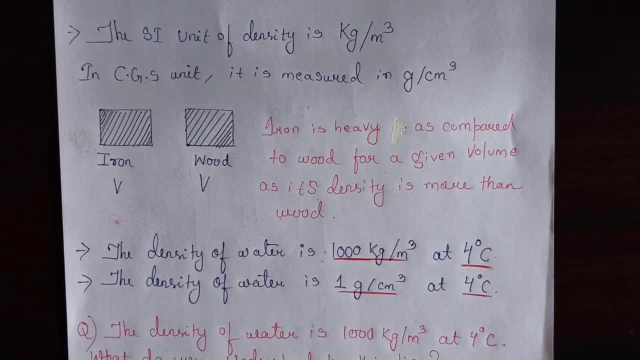 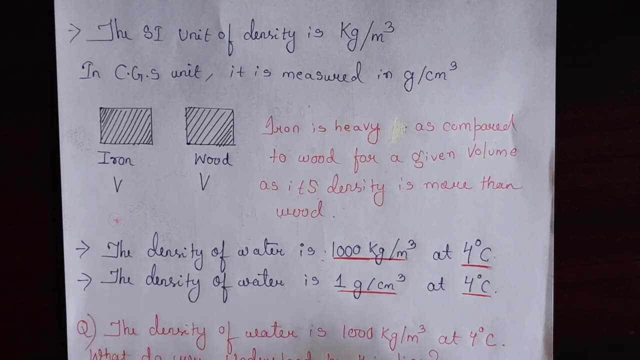 we will see the density. yes, I got my pen. let's see it. see how we will make it. now I am telling you the method. don't mess it up. it is a very easy method. you will make it easily. see how to do it. first of all, 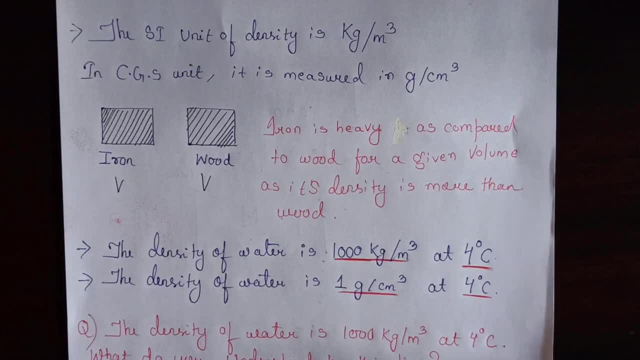 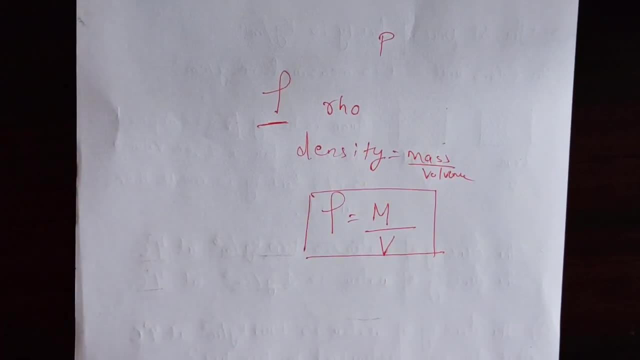 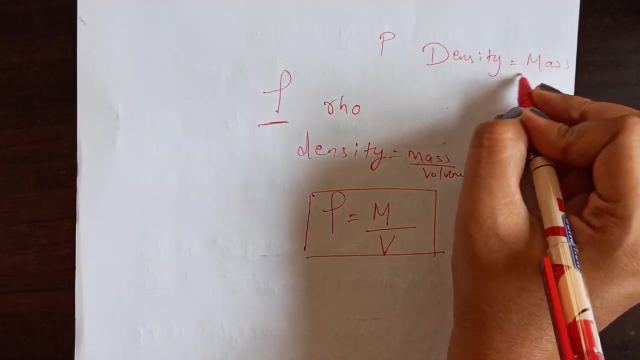 what I was telling you. write the formula of density. we will make it from here, we will make it from the back. I have the formula now. you have to remember a little bit. so for density, the formula is: density is equal to mass by volume. write this much. 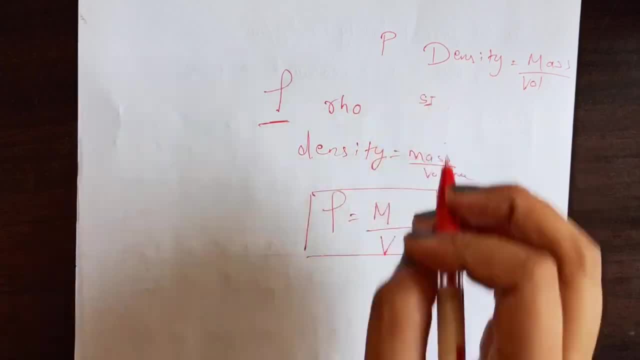 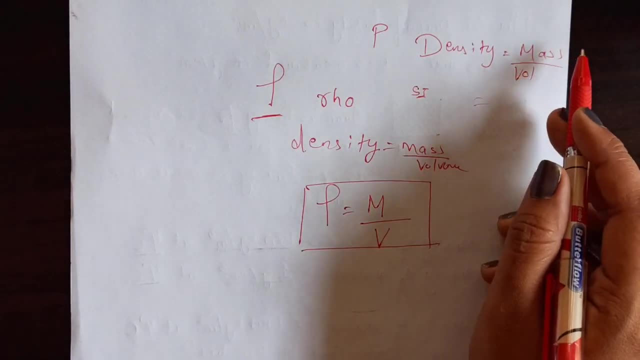 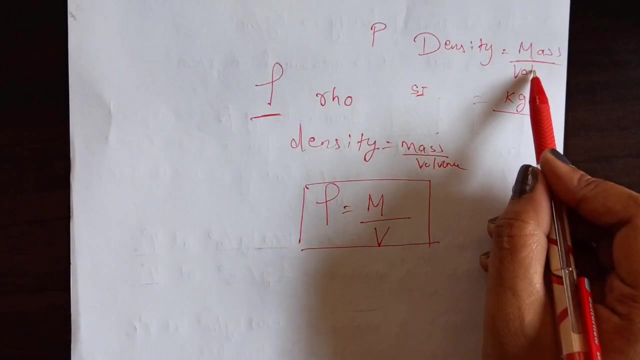 now I have to write its SI unit, which is internationally accepted, world wide accepted. now I am giving a question like this: mass's SI unit. mass's SI unit is kg and below it is divided by below. it is divided by 2, now volume. what is the SI unit of volume? 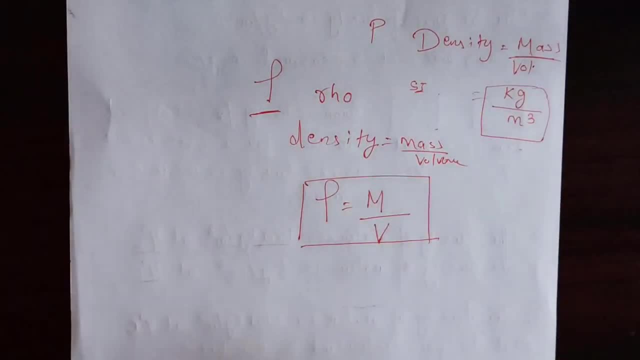 meter cube. so this is the SI unit of density. see how simple it is: kg by meter cube. this thing no one told us in the starting, but in the 11th class then we were told this method. I wish I had told you this method earlier. so 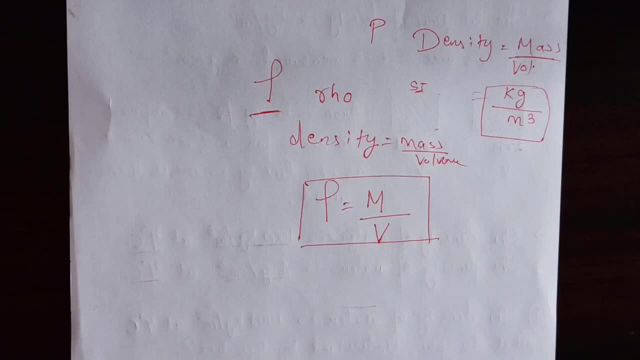 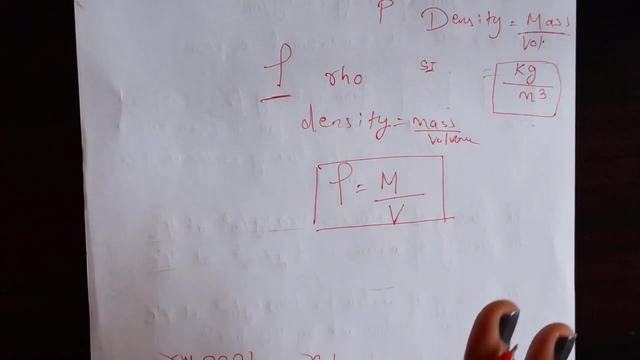 we used to work so hard. it used to be a problem, so I am telling you this from now so that you don't get into trouble. ok, so this is the SI unit- kg by meter cube. one is CGS unit. ok, CGS unit is actually a little smaller than SI unit. 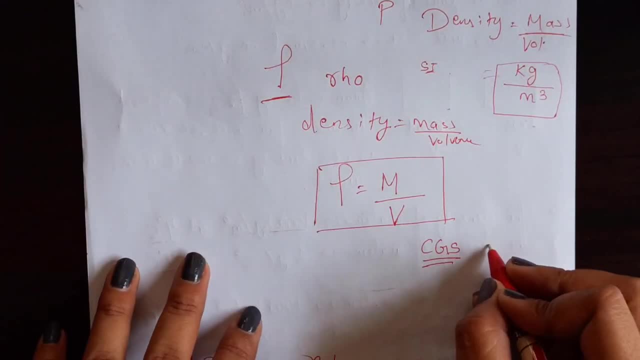 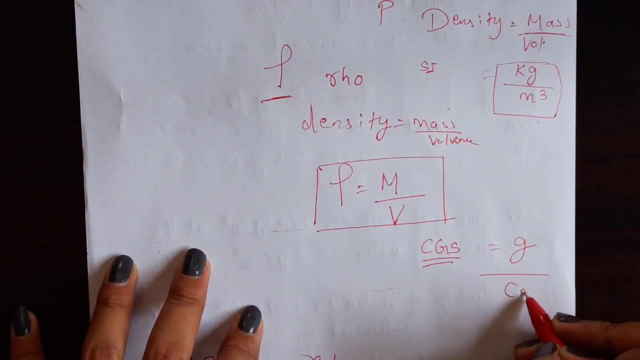 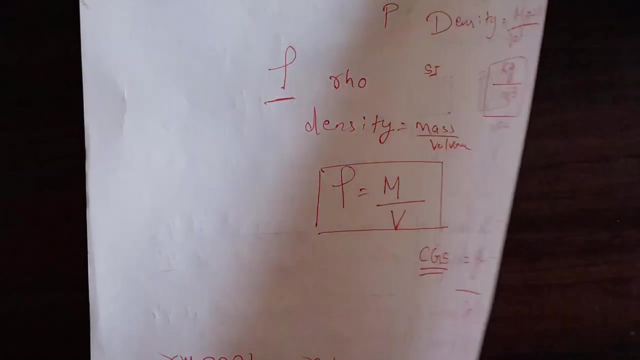 ok, so for kg we will use see. the same SI will be made, but for kg we will write g and for meter cube we will write cm cube. so this is the SI unit of density and this is the CGS unit. I have written it here very clearly. 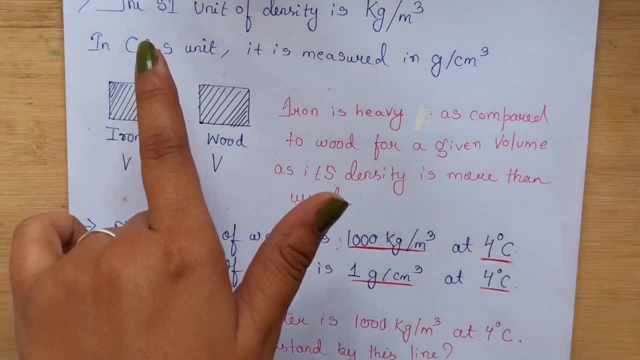 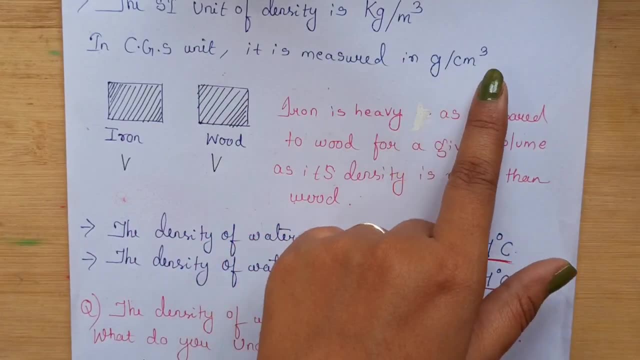 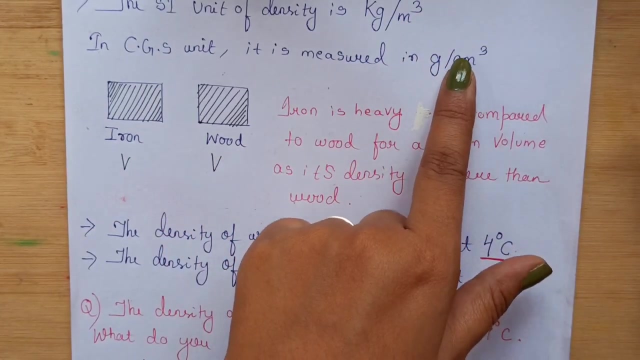 in the handwriting. so for that we have written here in CGS unit that the unit of density, CGS unit, that is g per cm cube. so this g came from kg and here as we had written meter cube, this became cm cube. now what you are seeing, 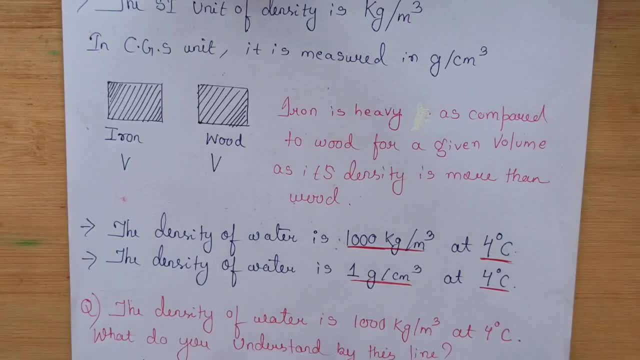 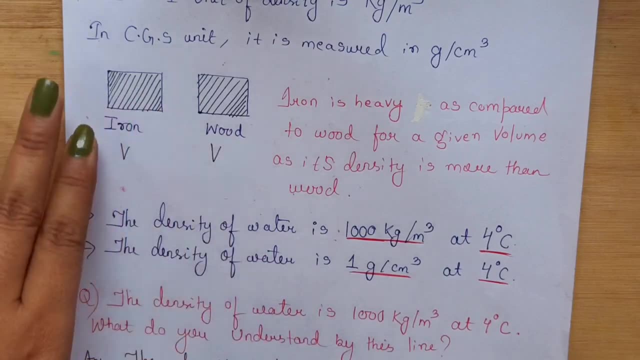 is a very important part. from here a question comes, like: think I have two objects here. one is iron object, second is wood. ok, think one is iron object and this is wood. both of them have same volume. if both of the objects which you have available, if both of them. 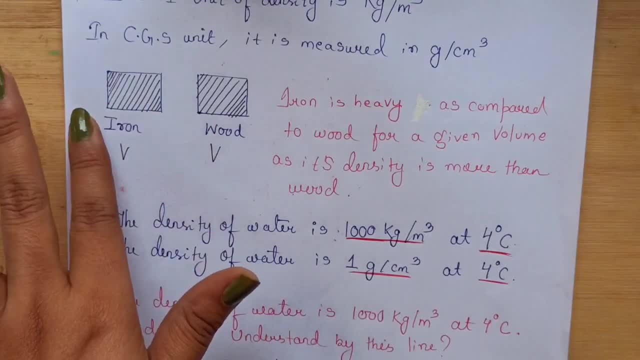 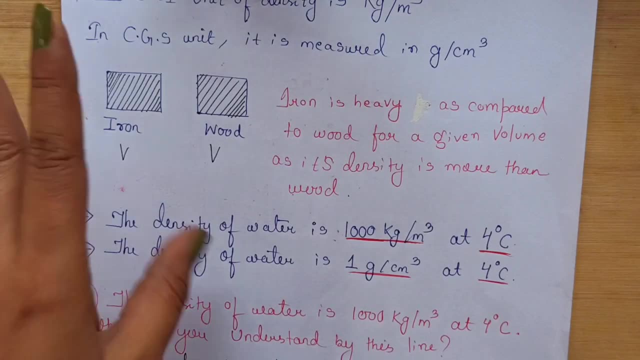 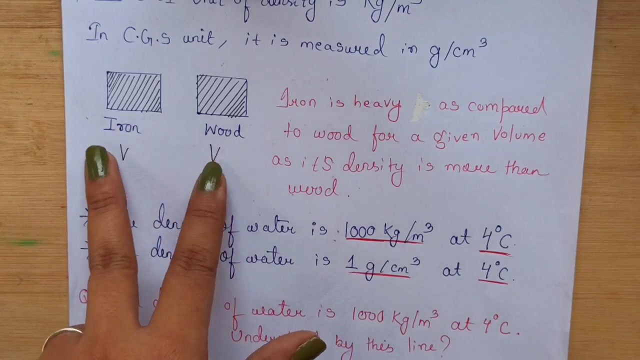 have same volume. so now we will compare that, which one will have more density, which one will be light and which one will be heavy, relatively ok. so here see if, if we compare there, which one is light and which one is light. so if you feel like, when you measure, 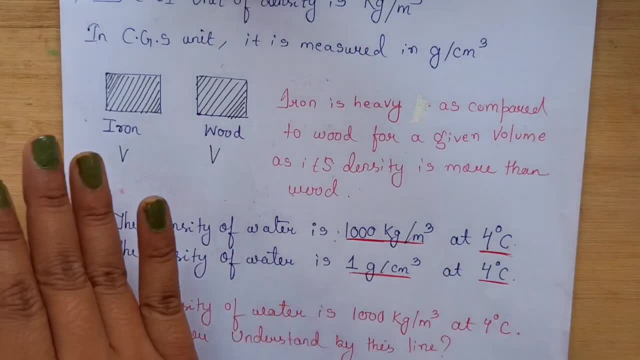 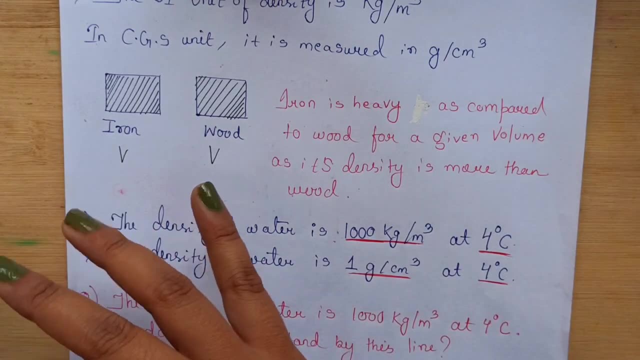 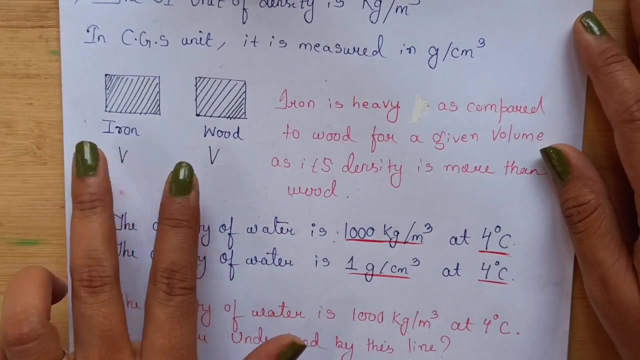 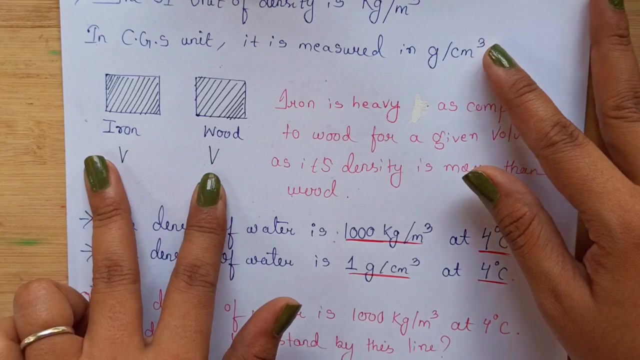 that iron. obviously, if volume is same, iron would be more heavier iron would be heavier than wood. why? because here iron density is more than wood. volume is same. this is the condition. if they have same volume, two different objects. but if their volume is same and if you are comparing, 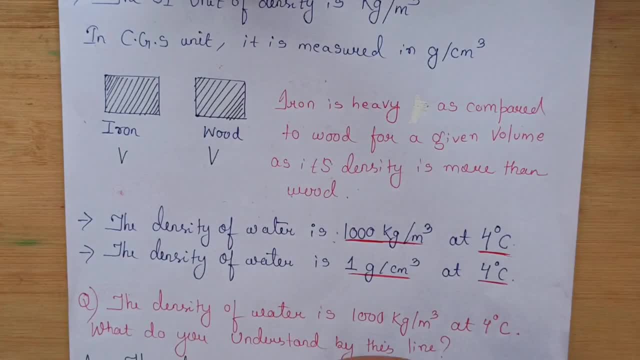 and if one object is heavy and one is light. so here, when we compare, so we got iron as heavy as compared to wood. so what will be the reason? the reason will be that the density of iron is more. iron density is more as compared to wood. so this is a simple. 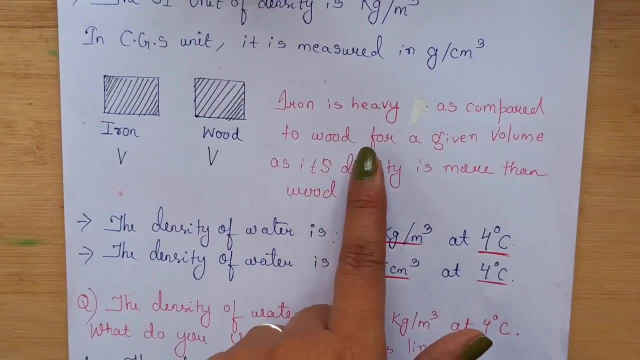 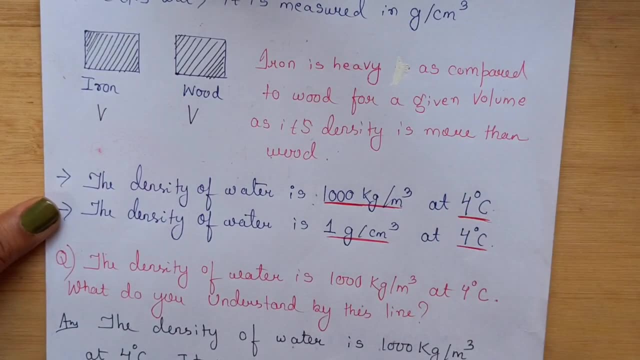 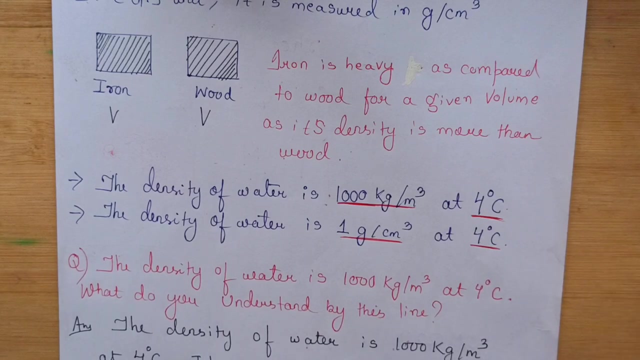 explanation. the question related to this comes. iron is heavy as compared to wood for a given volume, so we will be able to write it easily. this is simple to write and there is nothing much now. now see, till now we have two units of density. one is SI. 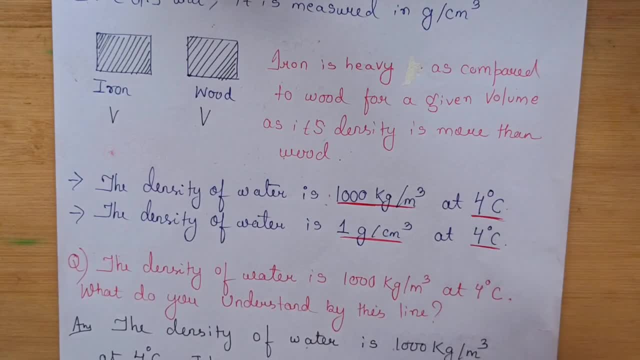 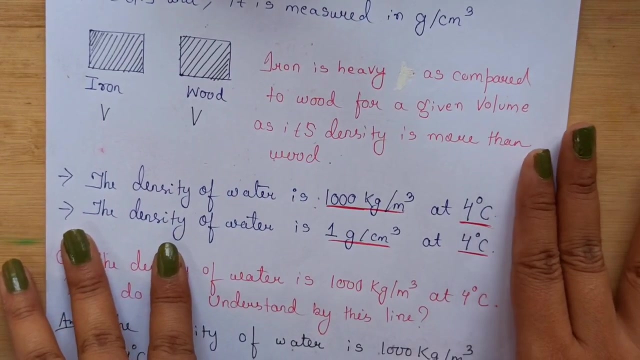 and one is CGS in SI: kg per meter cube. in CGS: gram per centimeter cube. we get to see now there is a term, not a term. a value is given here, like normally. if I consider water, water is normally considered at 4 degree Celsius. 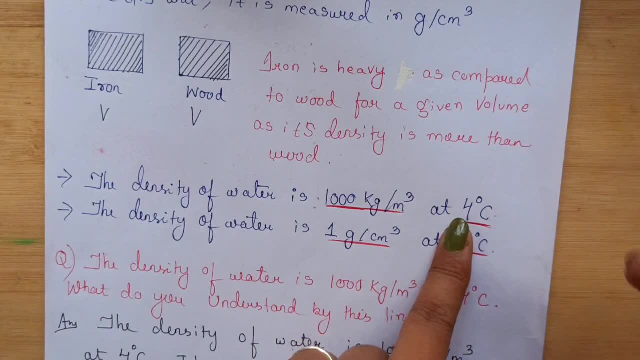 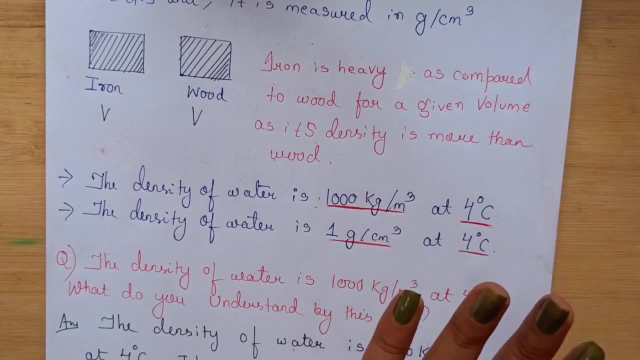 when the temperature of water is 4 degree Celsius means there is cold water. so density of water at 4 degree Celsius is 1000 kg per meter cube. this means, if we have water, what is its temperature? 4 degree Celsius. water temperature is maintained at 4 degree Celsius. 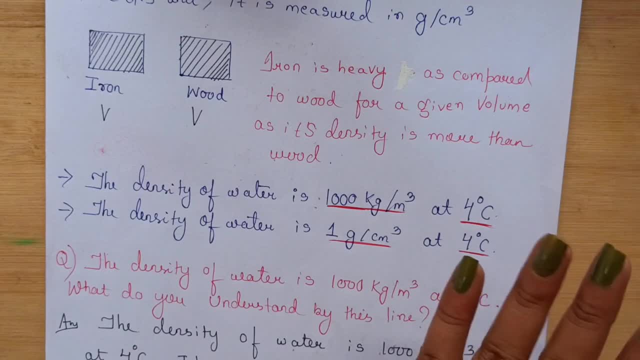 at that time, when we calculate its density, it comes out 1000 kg per meter cube. this is the number of kg per meter cube which I have calculated in the meter cube, the number of kg per meter cube which I have calculated in the form of SI unit. 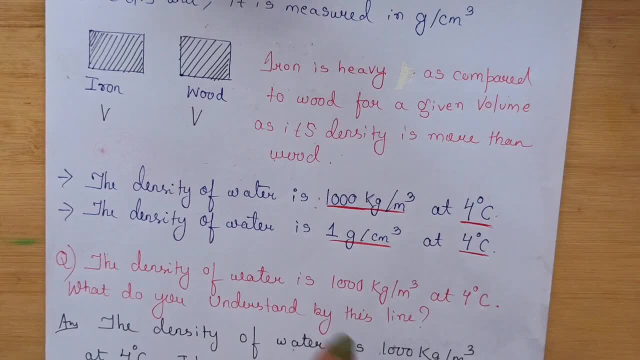 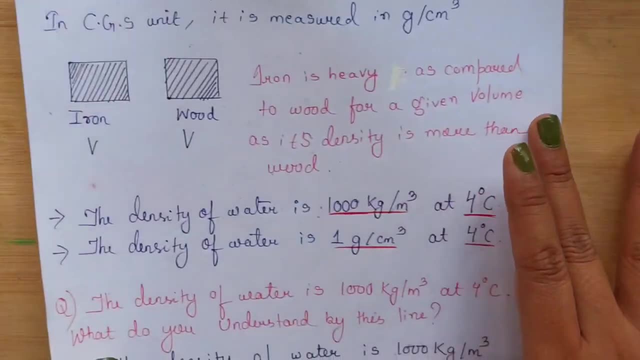 but if I have to calculate it in the form of CGS, then how will we calculate it? that density of water is 1 gram per centimeter cube at 4 degree Celsius means the same water, the same water. temperature is 4 degree Celsius. but if I talk about 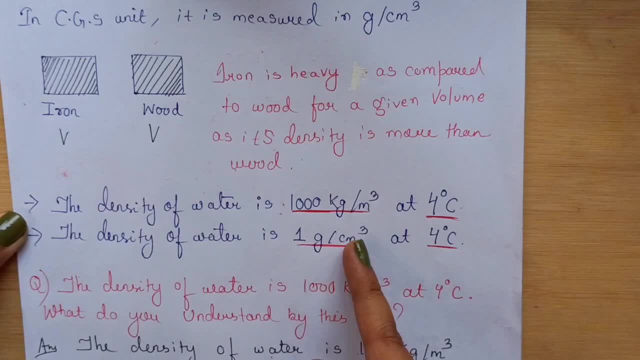 CGS unit, then its density will be 1 gram per centimeter cube. but if I talk about the same water in the same temperature- SI unit, then its density will be 1 gram per centimeter cube. so we will write 1000 kg per meter cube. 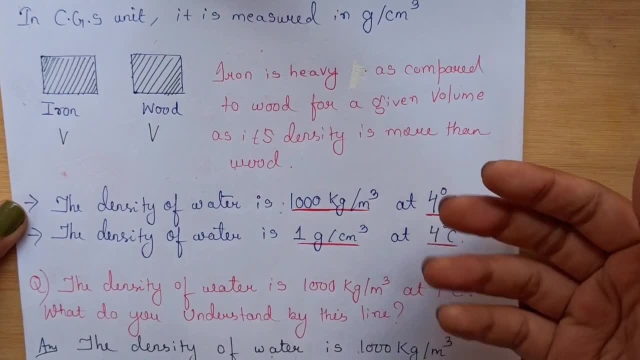 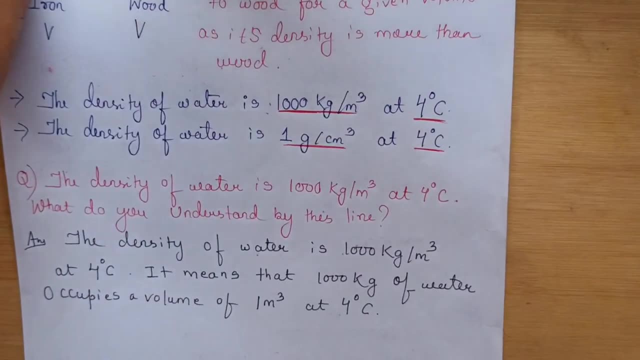 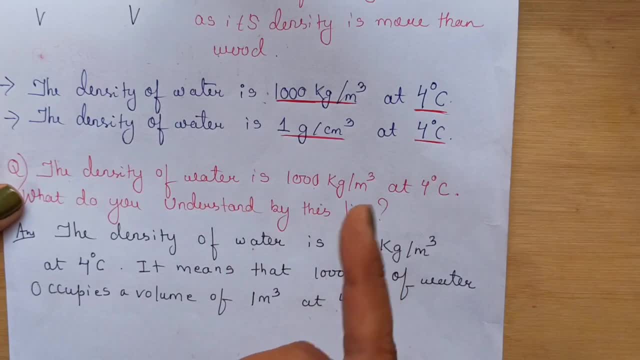 at 4 degree Celsius, which we have written the line above. then it will ask: what do you understand by this line? first look at the line. what is it? density of water is 1000 kg per meter cube at 4 degree Celsius. this means I have told you. 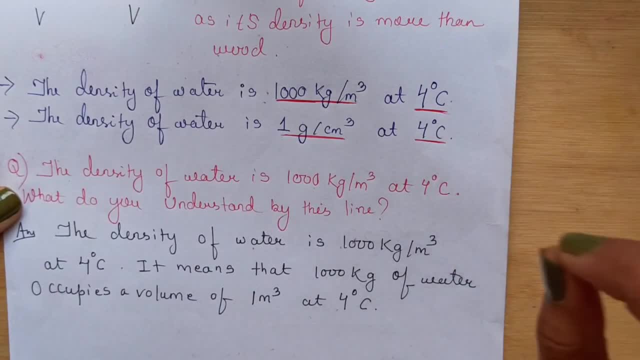 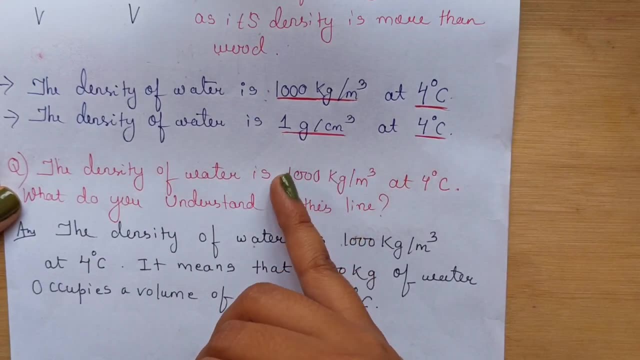 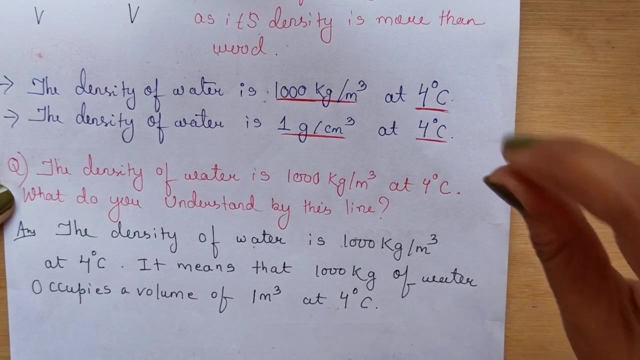 a little while ago, but again in a better way. we can write it like: how can we write? so this means, if we have 1000 kg of water, its temperature is 4 degree Celsius, so a water means 1000 kg of water, 1000 kg of water. 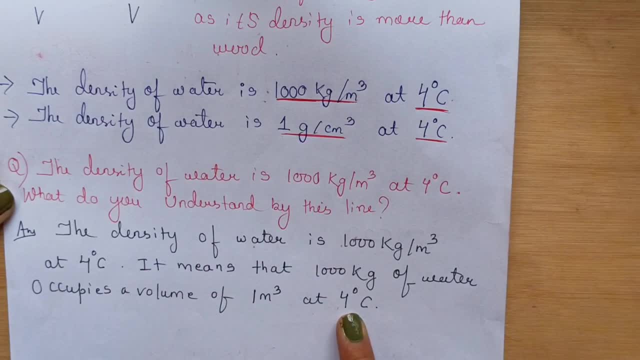 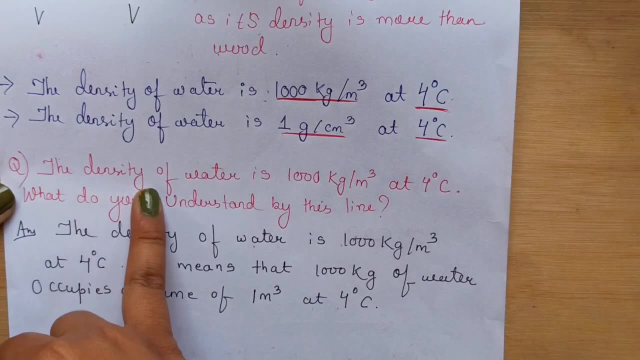 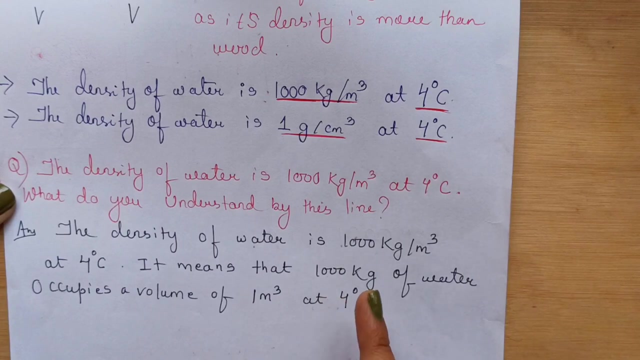 at 4 degree Celsius is: occupies this much volume. 1 meter cube occupies this much volume. this means, if we have said density of water is 1000 kg per meter cube at 4 degree Celsius, so that means 1000 kg of water occupies a volume. 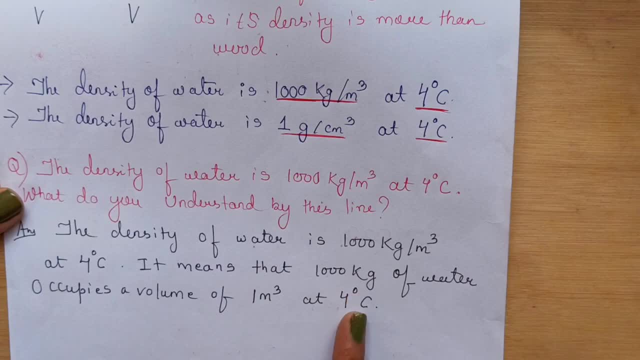 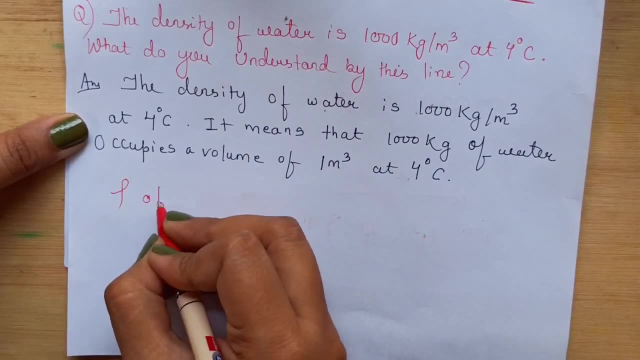 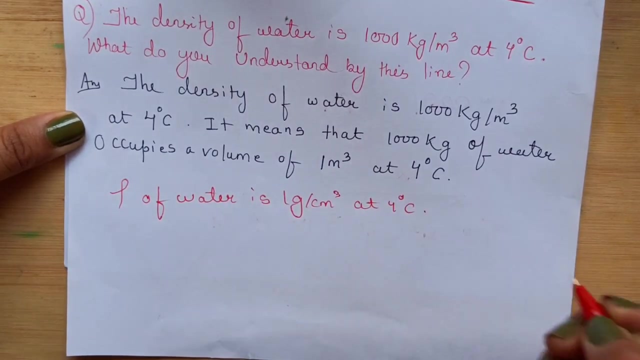 of 1 meter cube at 4 degree Celsius, if, if, if, if, if, if, if density of water is 1 gram per centimeter cube at 4 degree Celsius, in the question he will say: what do you understand by this line? this is also the same. 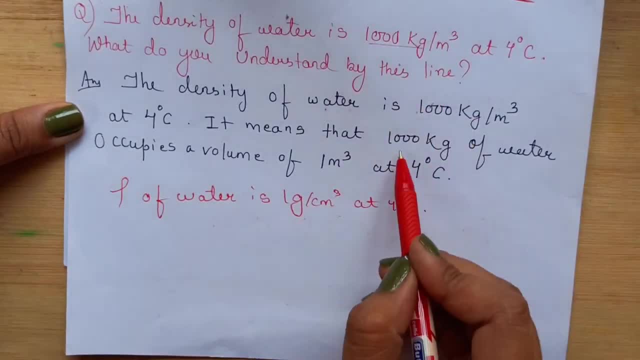 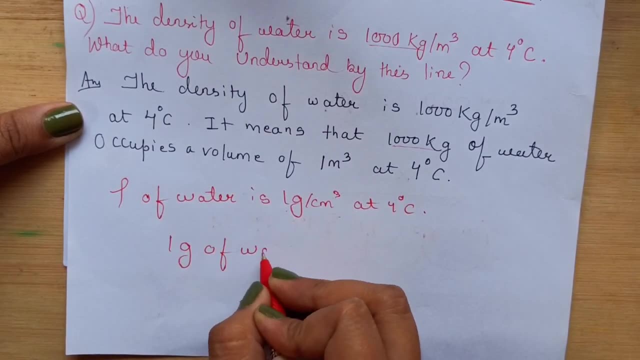 so what? you will understand that there was 1000 kg of water. so we wrote: 1000 kg of water, here is 1 gram. so what we are understanding from this: that 1 gram of water, 1 gram of water, occupies 1 centimeter cube. 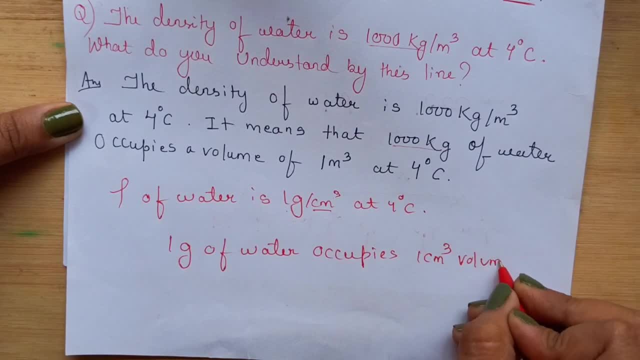 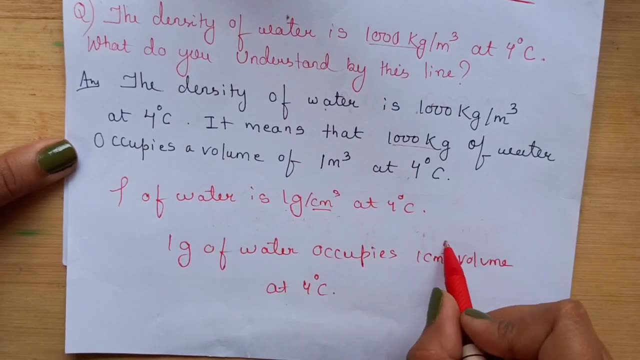 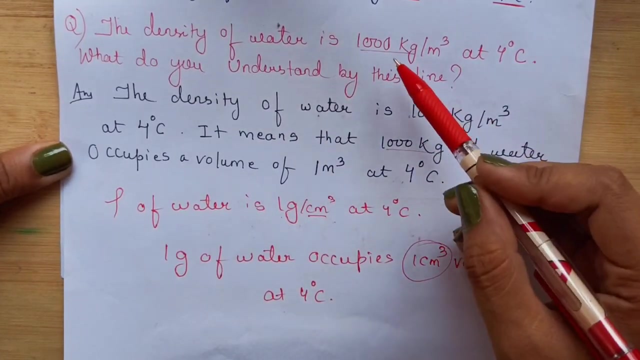 what volume of water at what degree Celsius? 4 degree Celsius. we can write this better: 1 gram of water occupies a volume of 1 centimeter cube at 4 degree Celsius. if 1000 kg per meter cube, then what we were understanding: that 1000 kg of water. 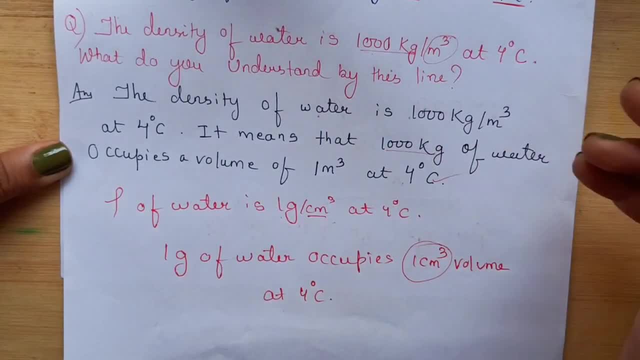 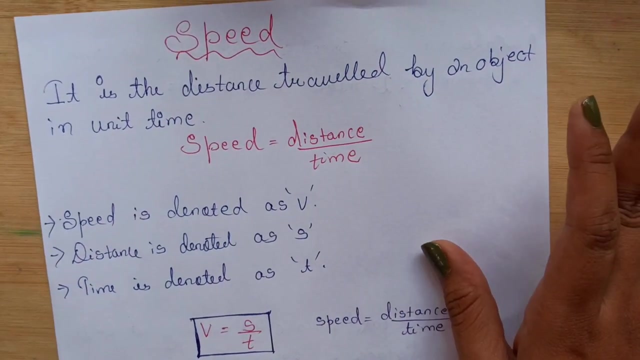 occupies a volume of 1 meter cube at 4 degree Celsius. these two questions are very important. there is no need to guess, if you understand, then the next topic is speed. that is related to density. there are some numericals which we will do later. ok, so speed. 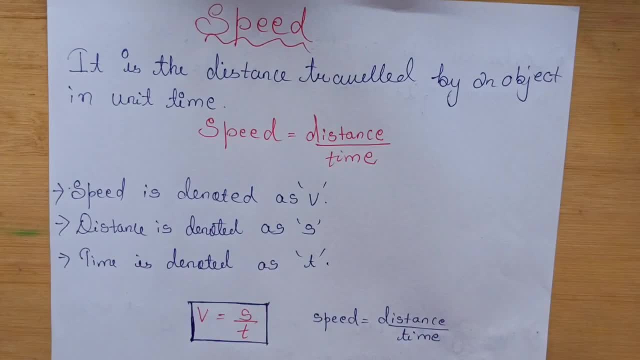 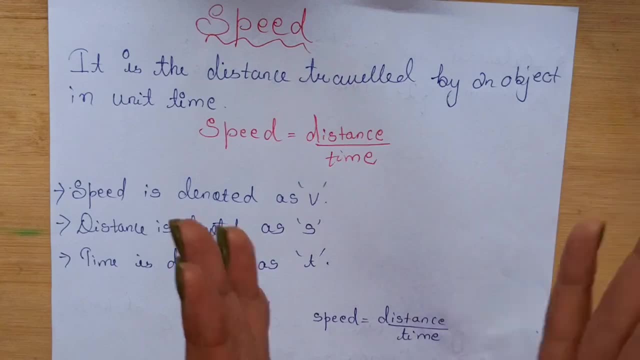 normally in our daily life, whenever we see a running, what a car, moving car. if a car is going fast, then what do we say? its speed is high speed is fast. if we see that any vehicle is going slow, then what do we say? it is going so slow. 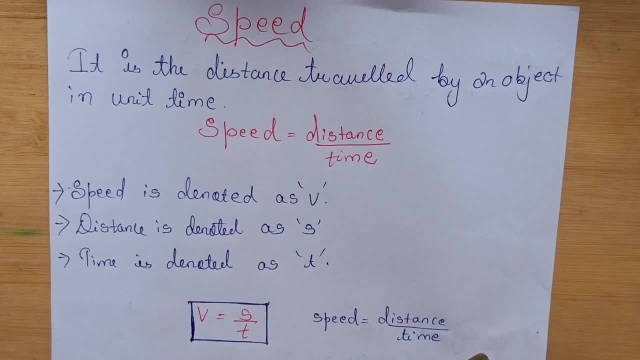 means its speed is low, its speed is less, its speed is slow. in our daily life, in our daily life, in our daily life, we always describe the motion of a body as fast and slow as speed. we see the motion of a body when a body is moving. 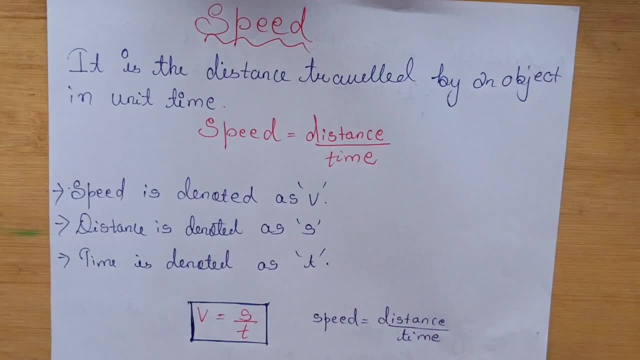 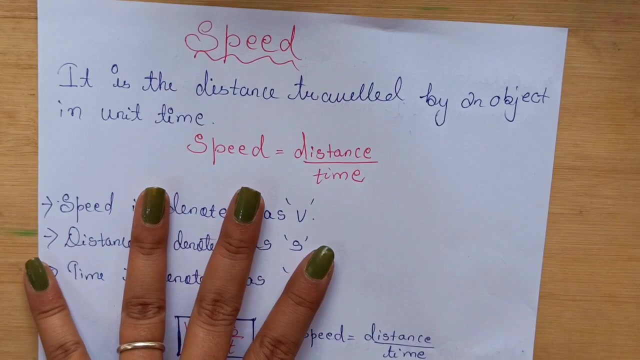 some of them move fast and others using speed we describe in terms of speed. if someone moves fast, we say its too fast. speed is more. if the riding of a body goes slow, speed is less. so now speed. We all understand speed, but how do we define it? 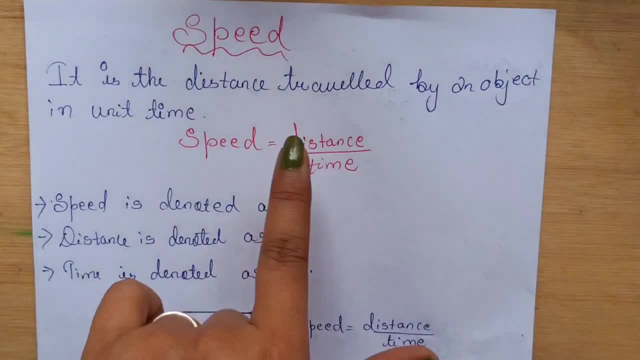 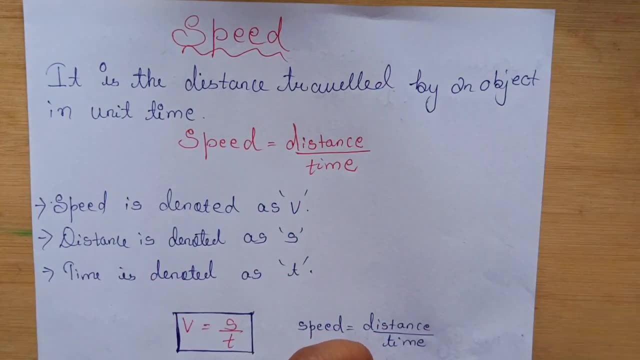 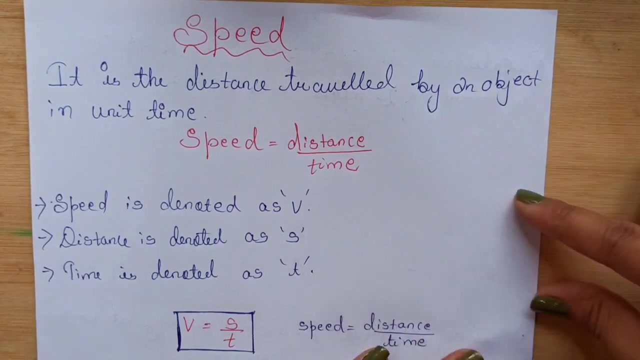 So how do we define speed? It is the distance travelled by an object or a body in unit time or per unit time Means an object travelled per unit time. For example, how much distance it travelled in 1 second, How much distance it travelled in 2 seconds. 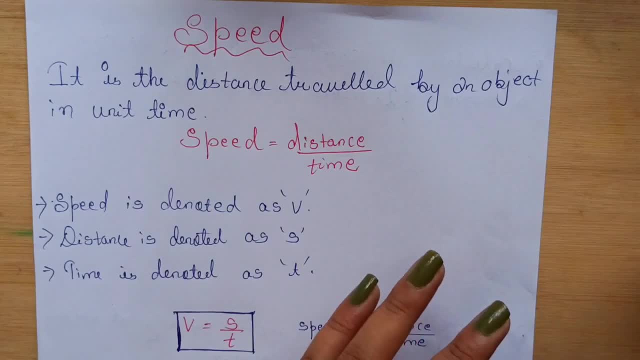 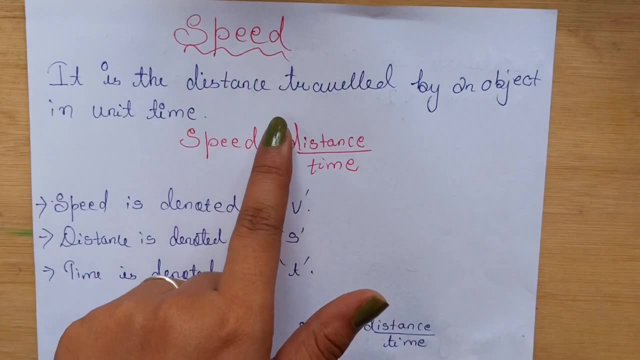 So how do we define it? It is the distance travelled by a body or an object per unit time. Its definition is the same as its formula. What is its mathematical expression? Speed is equal to distance by time. How do we define it? 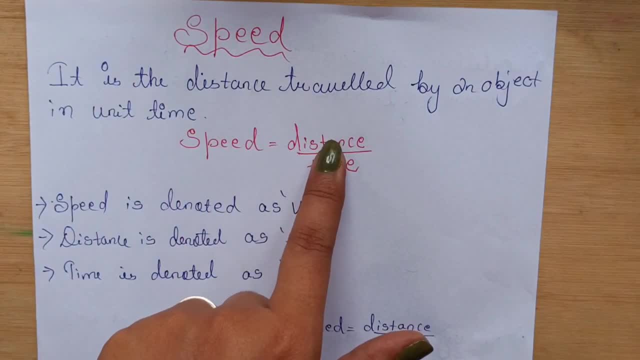 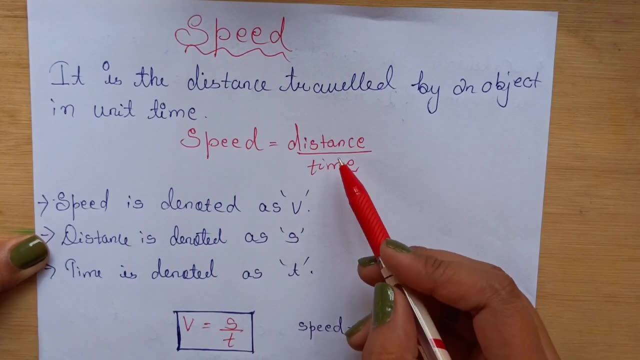 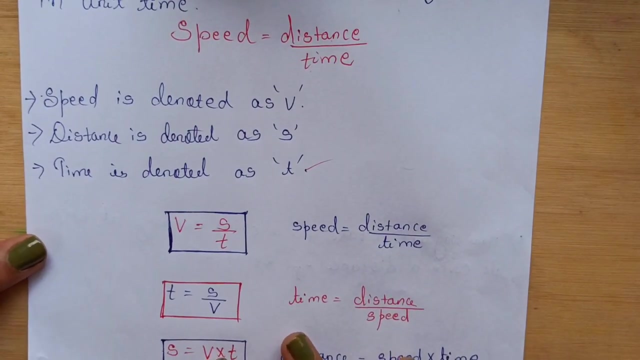 Speed is the distance travelled by a body or an object per unit time. Now we denote speed as v, We write speed as v, We write distance as s, And time is always written as t. So the mathematical expression given here is its formula. 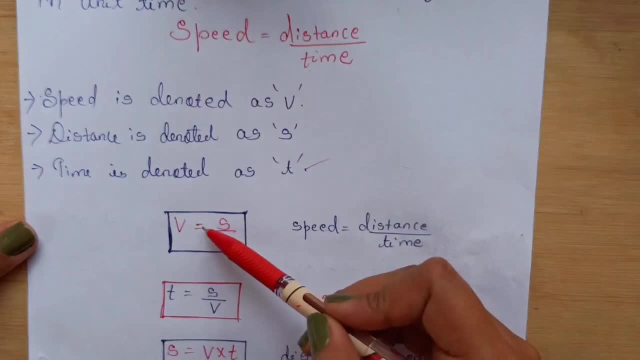 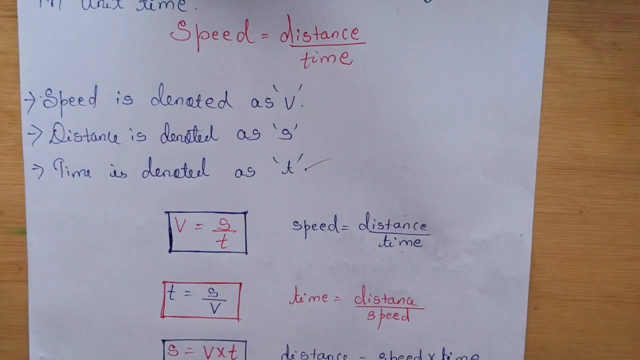 If I put the symbol here, what will it become? For speed, v is equal to s by t, So here speed is equal to distance by time. We can make many more formulas from here, Because when we do word problem numericals. 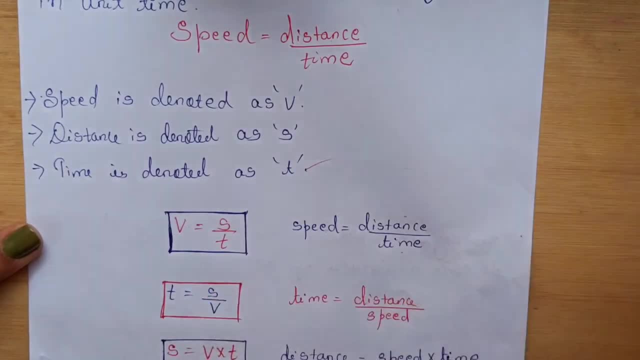 it is not necessary to always say speed. It will say sometimes measure time, sometimes distance. So if I want to take out time from here, So let's put time here And v will come here. So time is equal to distance. by what? 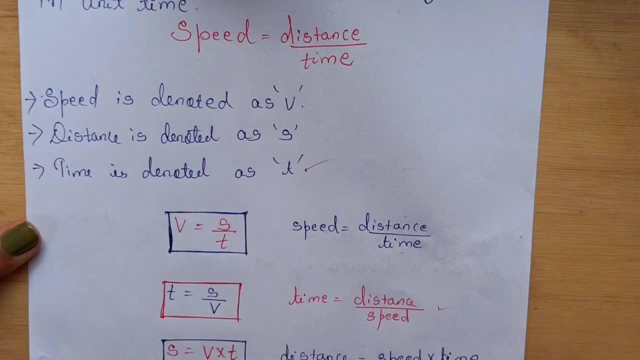 Speed. So this is done. Time is equal to distance by speed. If we want distance, what do we have to do for distance? Distance is different And v and t will be multiplied here, So distance is equal to speed into time. 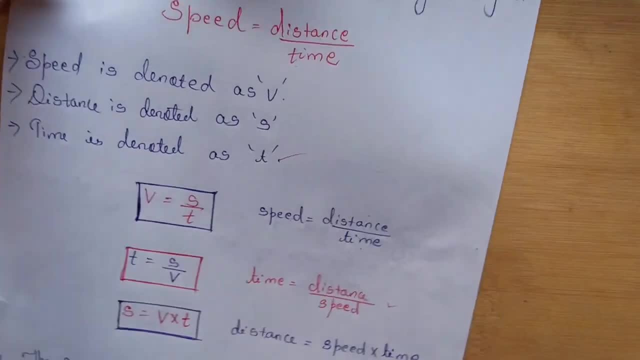 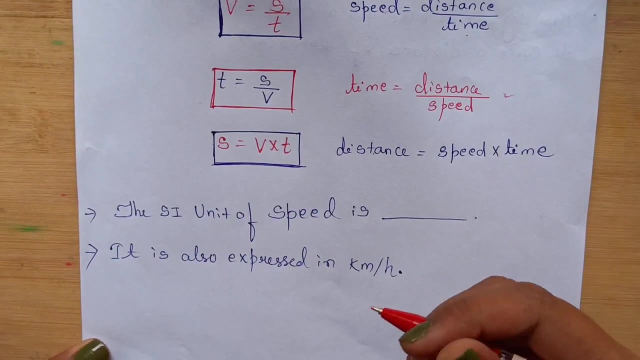 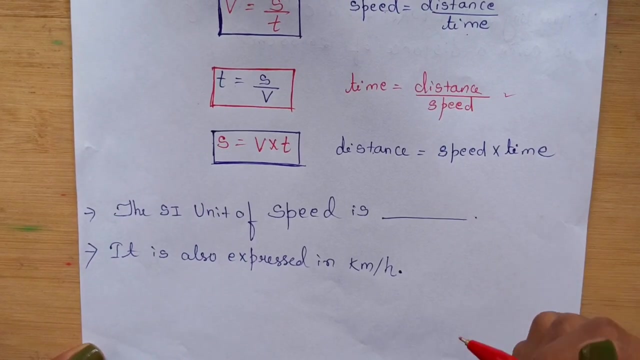 So these are simple formulas which are very useful in numericals. So we have to remember these three formulas. Now there is an important question. One more question: What is the SI unit of speed? What is the SI unit of speed? So we don't have to remember this too. 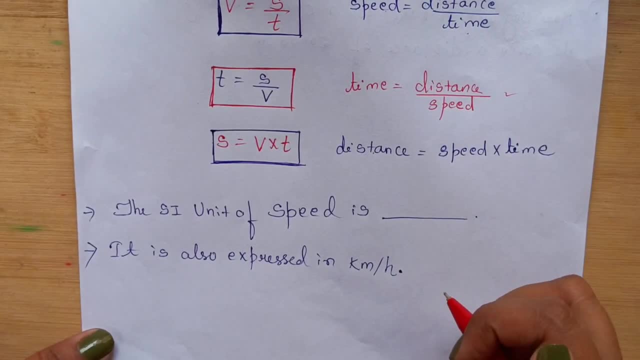 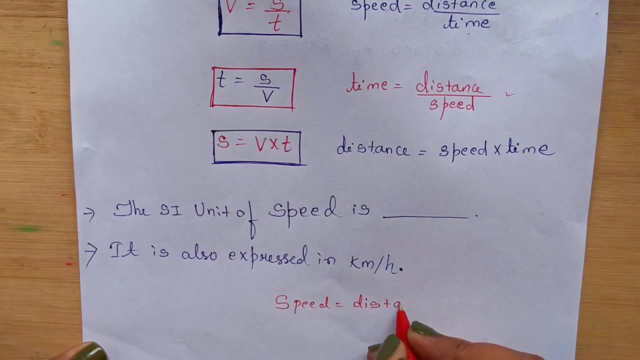 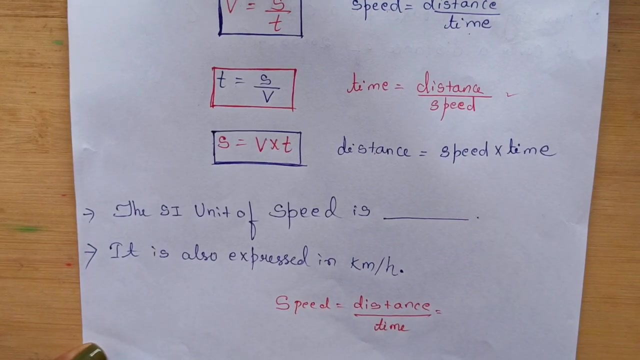 We can take it out easily. For this, what do we need? We need a formula. Just think Speed is equal to. First, let's write the formula Distance by time. Now, if I talk about the SI unit, So we measure distance by meter. 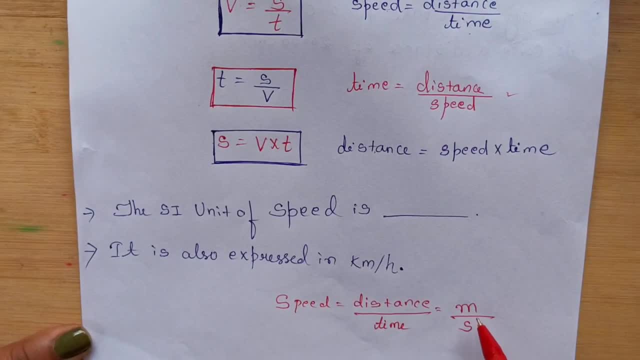 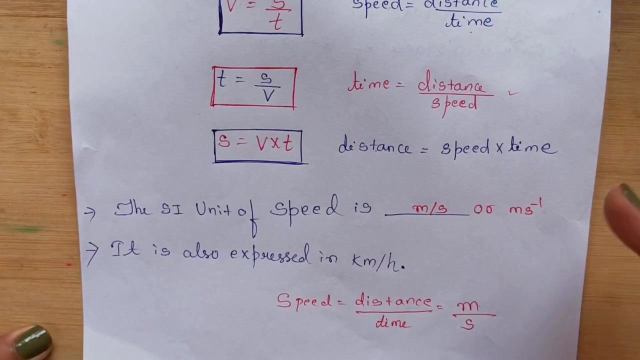 Divided by time. We always measure time in second. So this is done. SI unit of speed, Meter by second. So I can write it meter by second like this, And meter by second. We also write it in this type, But we don't always measure speed in meter per second. 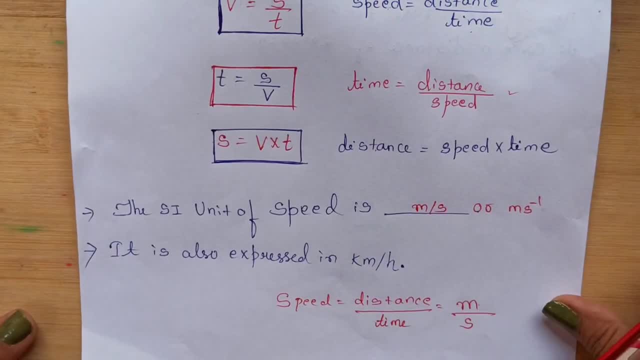 Because sometimes there are many moving objects which move very fast, Like take a train, take a car, take an aeroplane. They move very fast, So when their speed is taken out, So we take it out according to kilometer per hour. 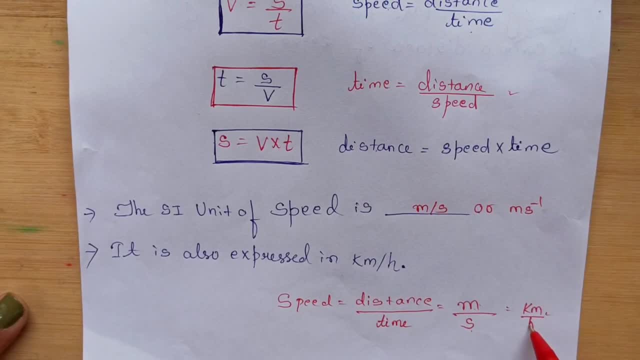 Kilometer is made up of meter And second is made up of hour. S here is for hour, Here S is time unit. second, Here S means don't understand distance. This is its unit. So we can also measure according to kilometer per hour. 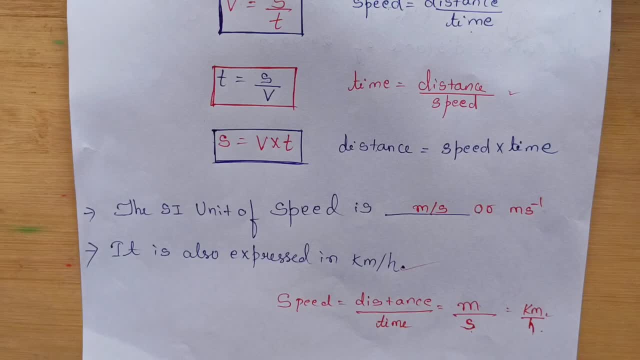 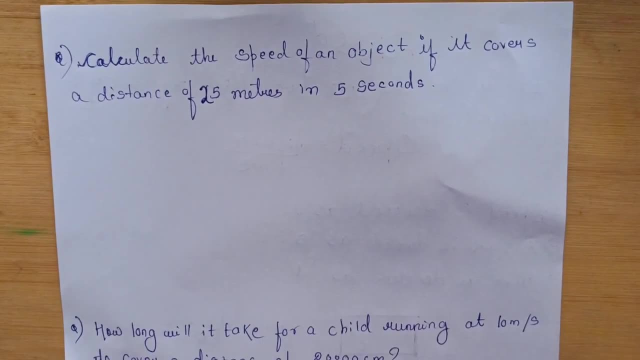 When, If we are talking about very fast moving objects, Otherwise, normally the SI unit of speed is meter per second. Now let's solve some of the numerical related with speed. We have to remember the formula: Speed is equal to distance by time. 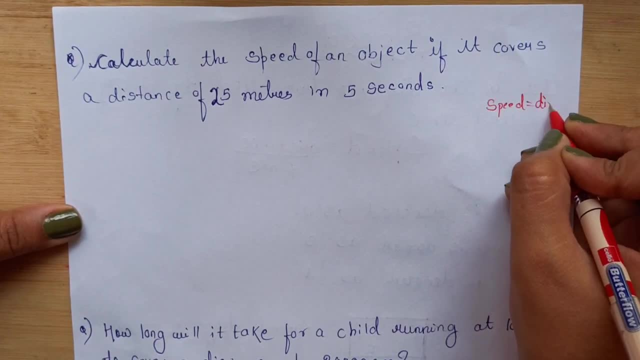 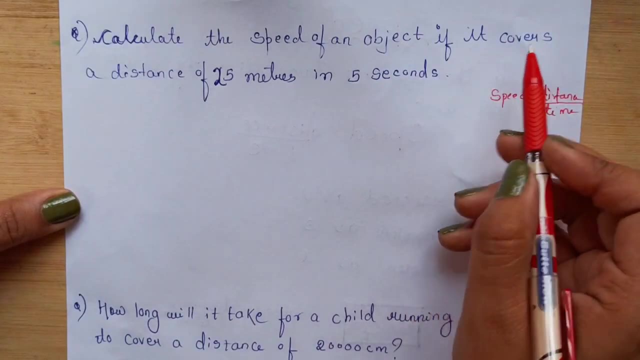 We will remember that So we will be able to do it easily. So let's do Okay. So first question: Let's see what is given: Calculate the speed of an object If it covers a distance of 25 meters in 5 seconds. 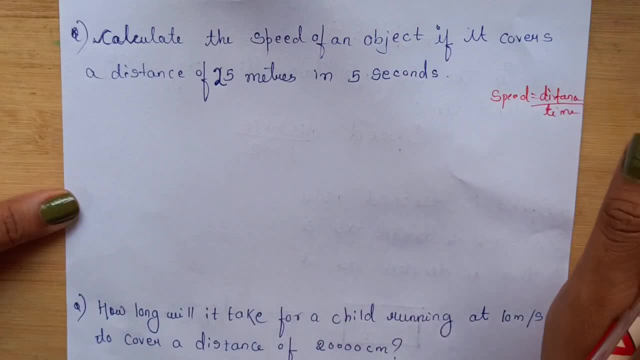 Now we have to remember one thing before starting the numericals: We will understand the question after reading it, But we can also find out by looking at the unit. Is it talking about distance? Is it talking about time? Is it talking about speed? 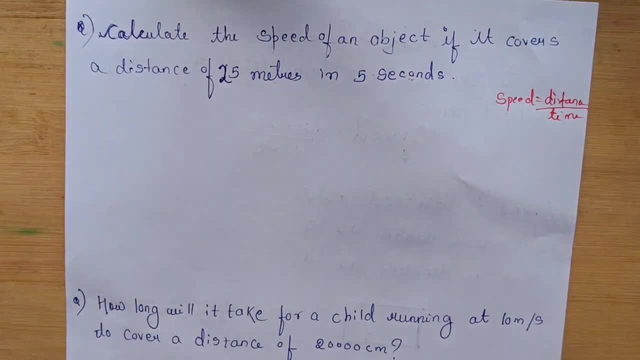 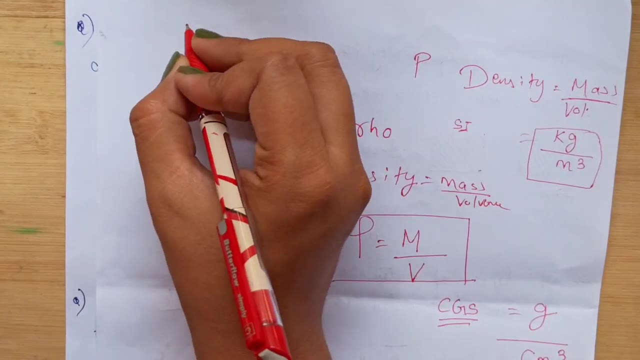 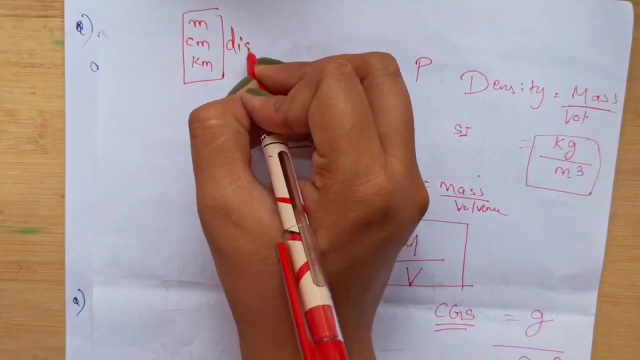 So if the unit is given, all this, Okay, If you think in the question, What is the matter of meter or centimeter or kilometer? So all this is the matter of distance, Means all this unit is for distance. So if you see in the numericals, 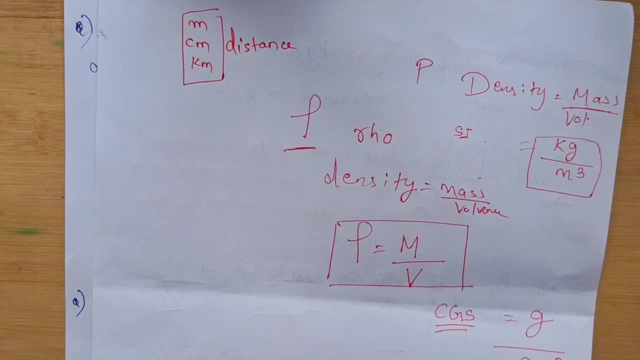 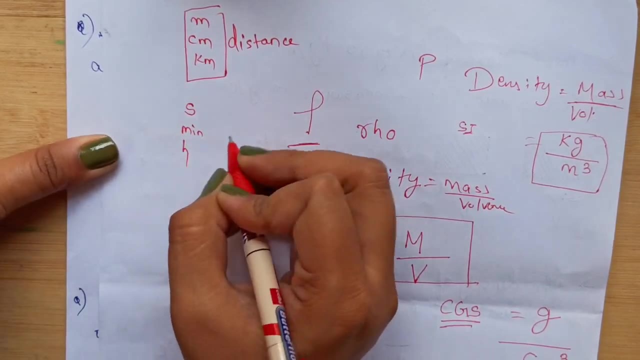 That meter, centimeter, kilometer. If it is written all this, then there is a matter of distance, So that distance is given. Similarly, if I talk about time, then second Minutes are also written there. Sometimes hour is also written here. 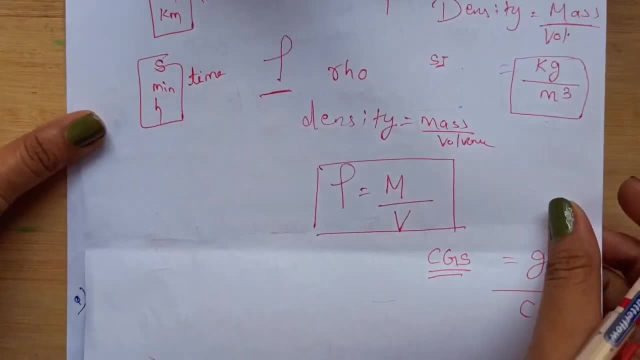 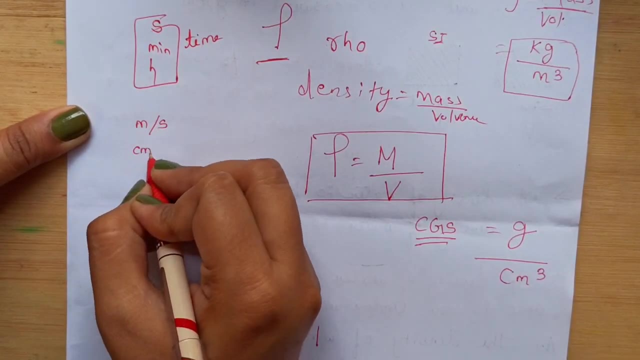 So all this is for time. This is also important. All this is for time. Next, if I talk about speed, So that is meter per second or centimeter per second Or kilometer per hour. What will be given according to this? 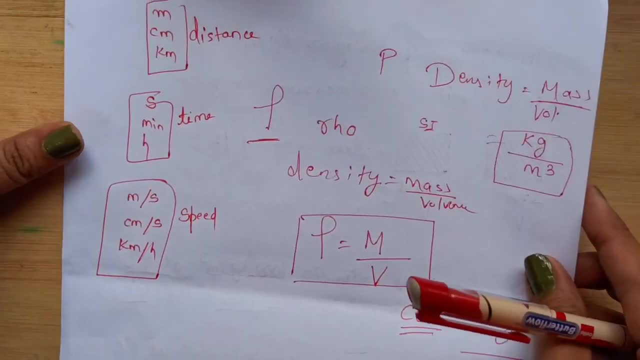 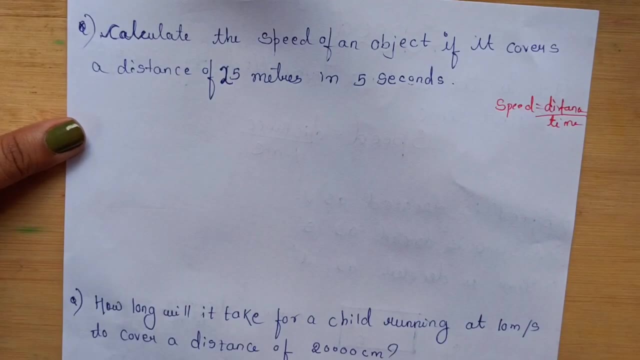 We will be given speed. So you have to remember these three things. If you remember this, then there will be no problem in solving the numericals. Next, Now, we will do by looking at this First question is: calculate the speed of an object. 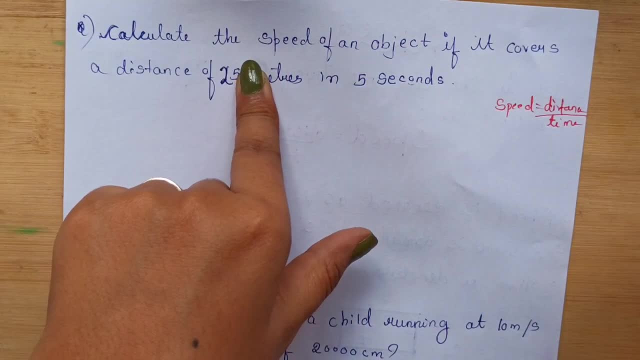 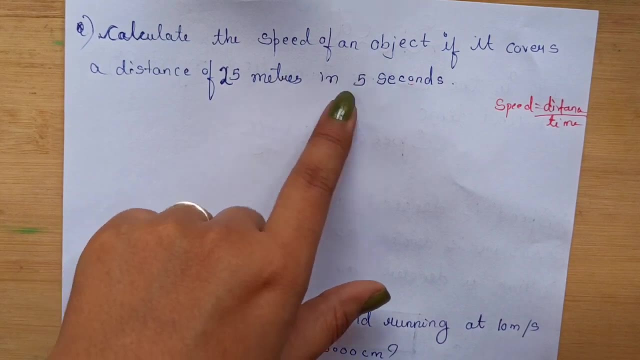 Means to calculate, means to find out What we have to find out. We have to find out the speed of an object If it covers a distance of 25 meters in 5 seconds. If an object is travelling 25 meters in 5 seconds. 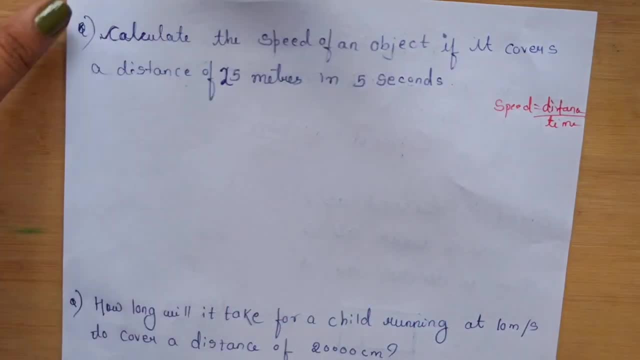 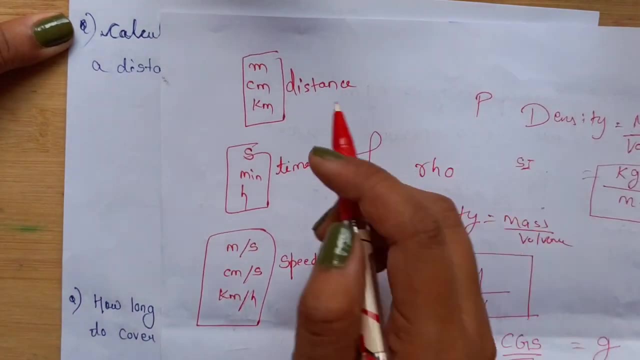 Then calculate its speed. First, see what is given. It is given 25 meters And it is given 5 seconds. So meter means What we see. for meter, See, meter means distance is given And there second means time is given. 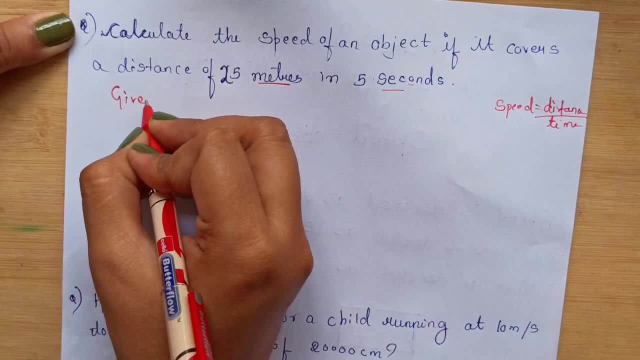 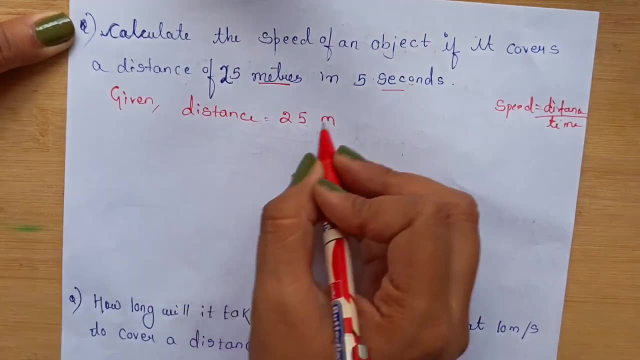 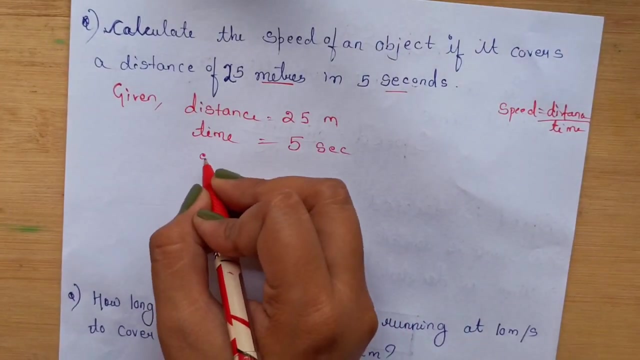 Ok, So here we will write: given distance, How much distance is given? 25 meters. So make it 25 meters. Meter means distance, 5 seconds, Obviously. second means time. I write here 5 seconds, What we have to calculate. 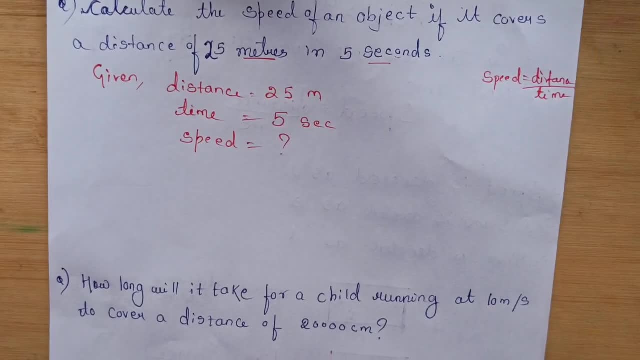 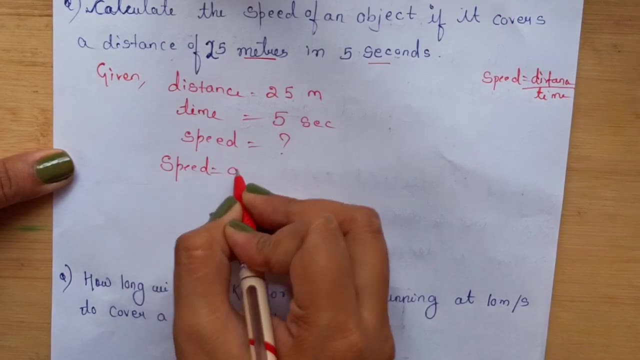 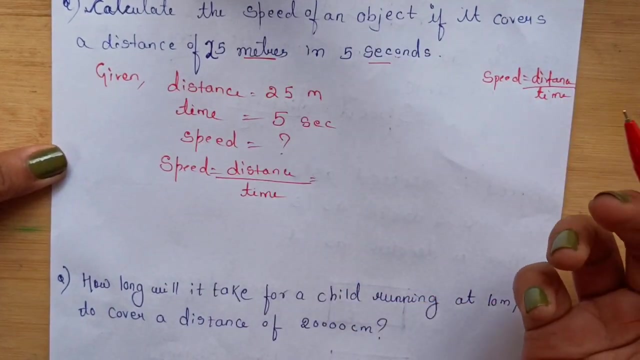 We have to calculate speed. So how to calculate speed? We will use its formula here. So what is the formula of speed? Distance by time. Speed is equal to distance by time. Now, wherever the object is asked, We will put it and get the answer easily. 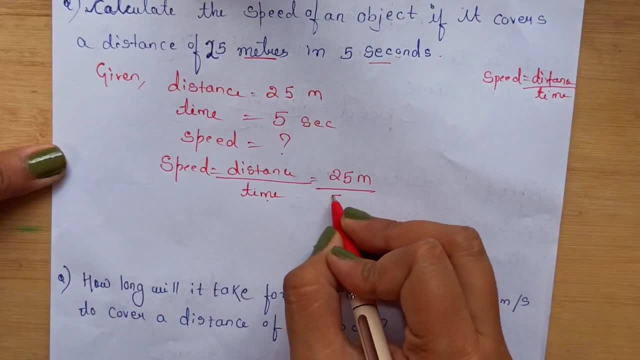 How much distance is given 25 meters? How much time is given 5 seconds? Let's write like this: Now cut this, It will become 5.. 5,, 5,, 5.. So this is 5.. 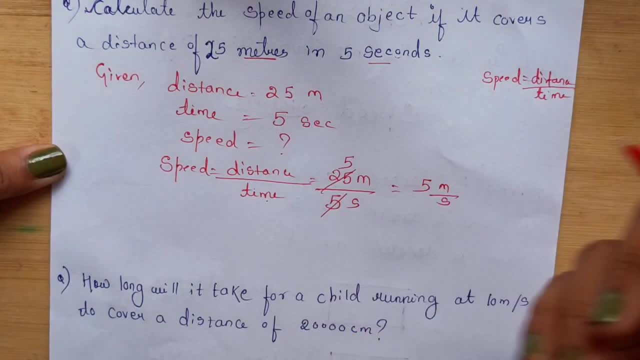 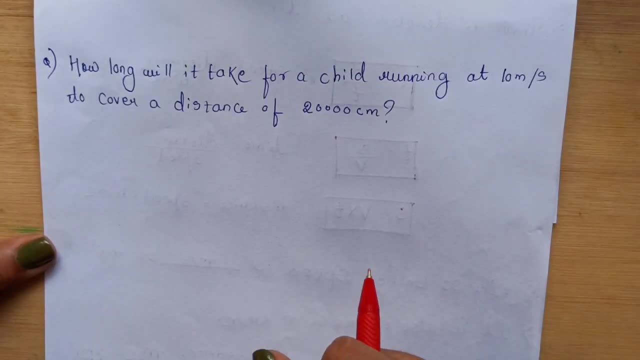 The above is meter, Below is second. Answer is here. How simple is this? By the way, there is one more question. See this: How long will it take for a child Running at 10 meters per second To cover a distance of 20,000 centimeters? 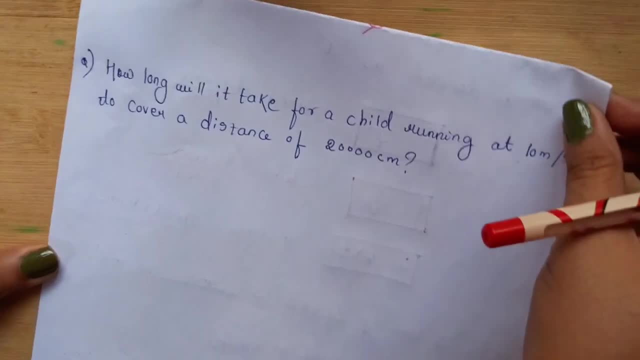 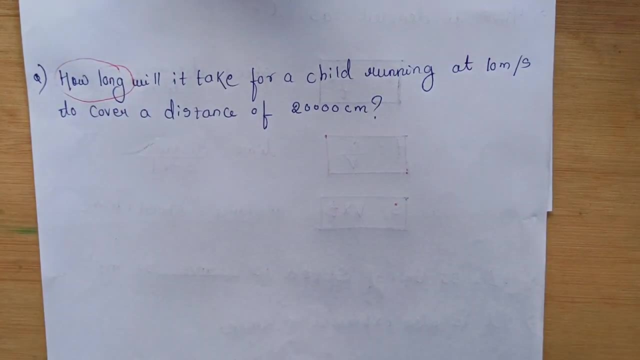 Now, what is this given? No, No problem, It is very simple. See what is in this. First of all, it is saying how long. So where you saw how long? Now you are seeing the math of classic. It was speed, distance and time. 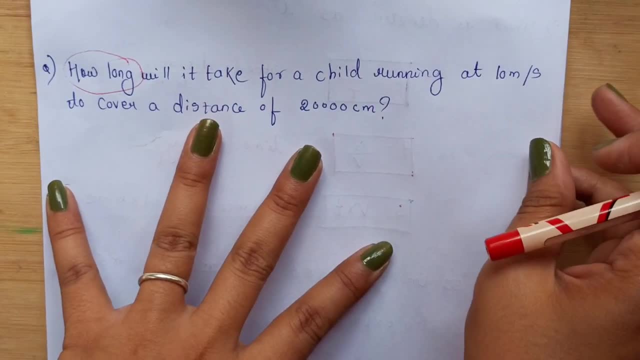 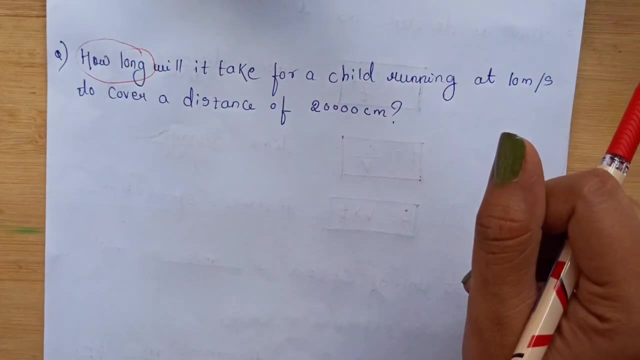 There was a question of this type: How long? Long means it is talking about time. How long means it is talking about time. So, in the question, if you see how long It means to take out time, How long will it take for a child? 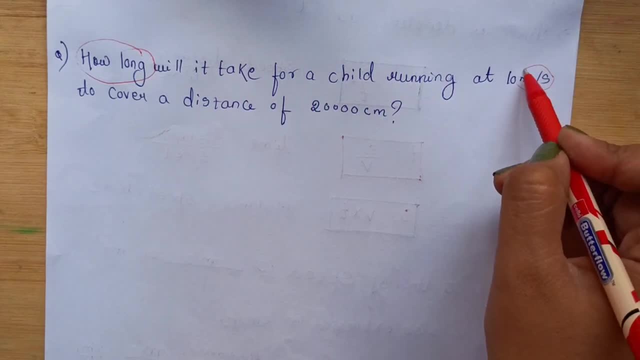 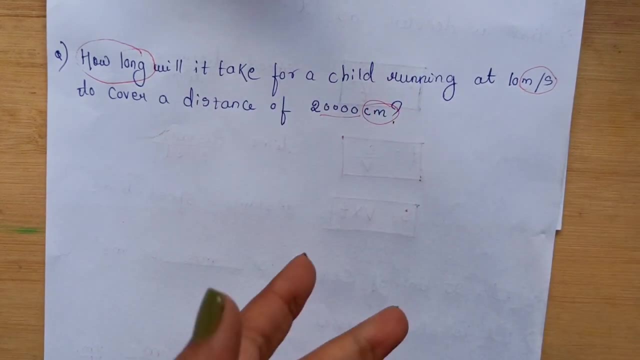 Running at 10 meters per second. This meter per second unit is given To cover a distance of 20,000 centimeters. Now let's see what is given. You must have known by looking, But one way, which I have already told you. 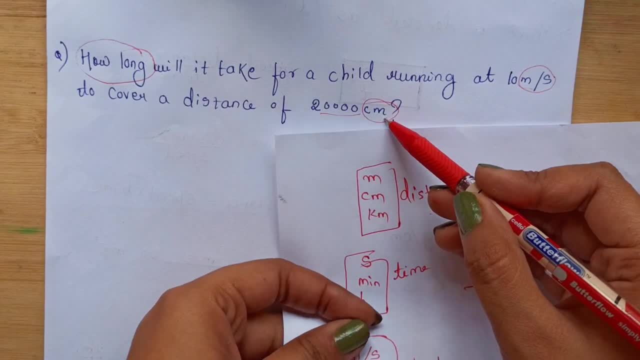 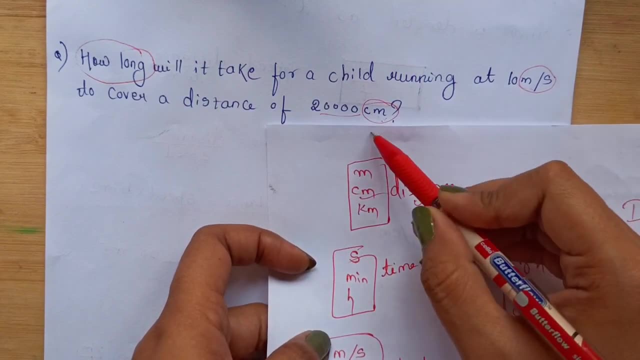 As in, we have given centimeter First. we will see if this is centimeter. I hope this will be visible. Yes, So it is centimeter. So what is the meaning of centimeter Distance? now you know that it is distance. 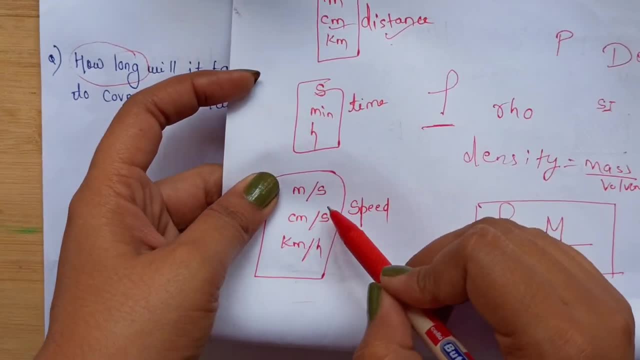 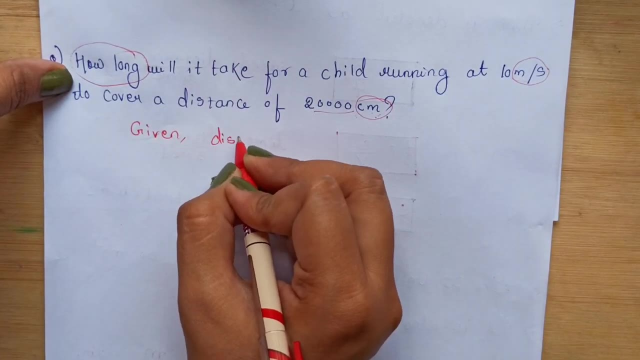 It is given meter by second. So meter by second, This is meter by second, Means speed is given. So you have understood that. Then we write it as given. Distance is given to us first, 20,000 centimeters Speed is given to us. 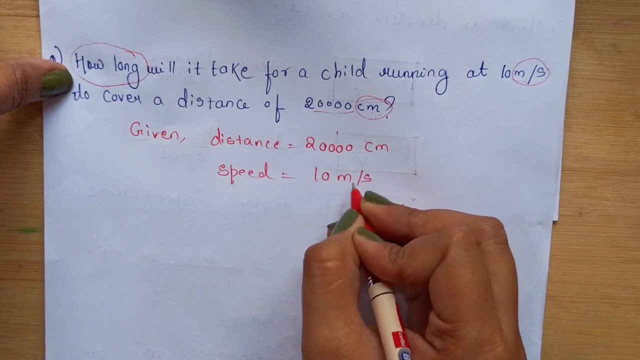 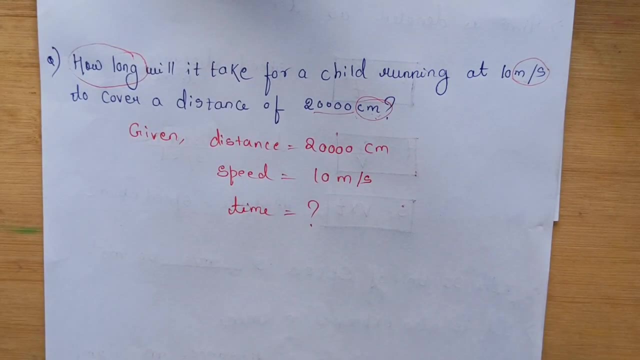 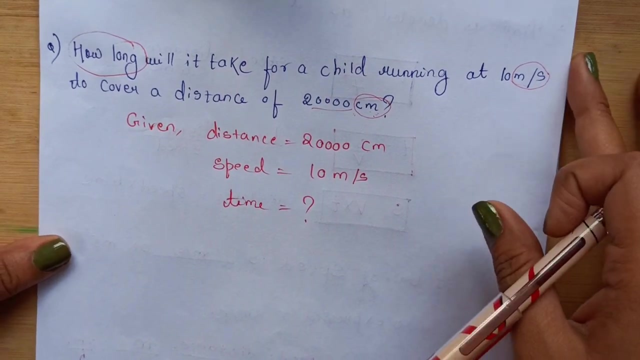 speed we have given is 10 meter per second. what time we have asked. how long means time we have asked. now you will say that here. ok, you may not know, I will tell you, and if you know, then very good. see, I will tell you one thing. 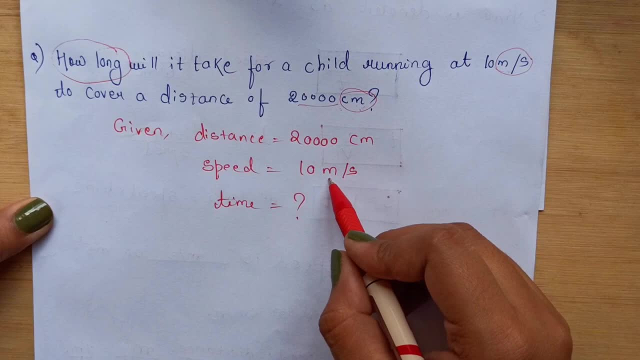 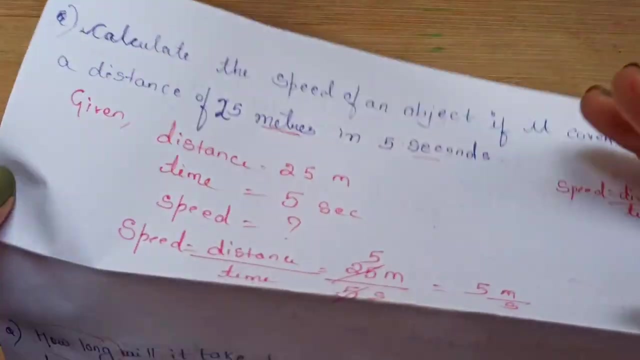 like see here speed. we have read: speed is given in meter per second. if speed is given here, 10 meter per second and here distance is given in centimeter. so here meter is not matching with centimeter. before this what we have asked here distance is 25 meter. 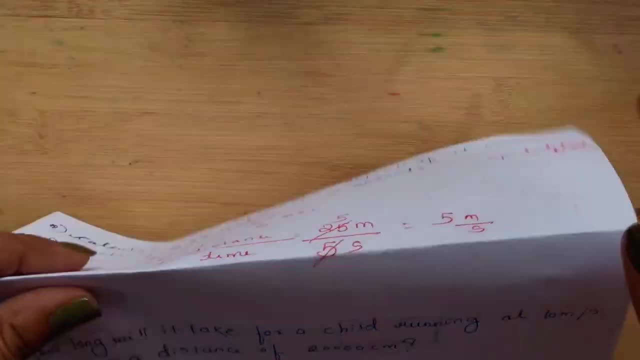 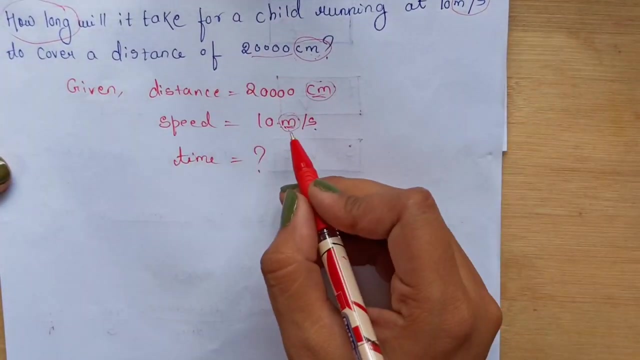 so here speed is given in meter per second. so it should match like this. it should be one unit, ok. so here distance is given in meter, sorry in centimeter, and here speed is given in meter. so it will be better for us if we convert it in one unit. 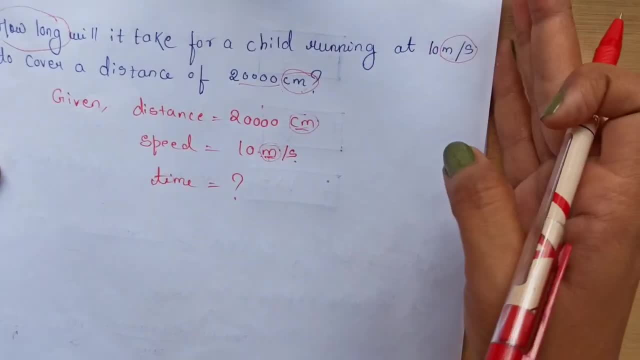 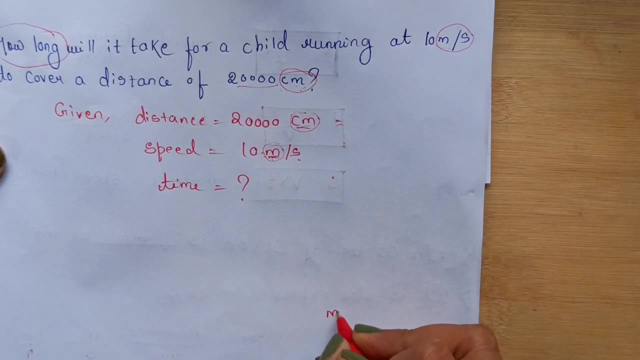 ok, if meter is given here, then convert it in meter form, or else we will get wrong result. ok, so now we will work. we will convert centimeter into meter. so we have read- I have already told you in this video: meter, then decimeter, then centimeter. 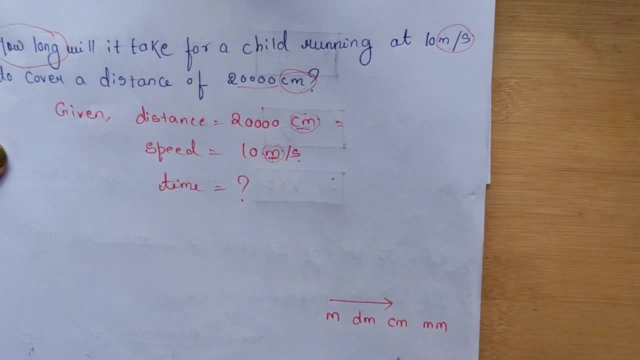 then millimeter. we will convert like this: this is small and this is bigger. when we go in descending order, then we multiply, and when its reverse comes in ascending order, then we divide it. so in which I have to convert from centimeter in meter, in meter from centimeter. 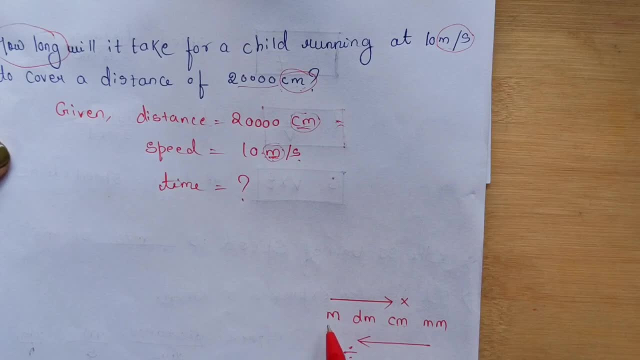 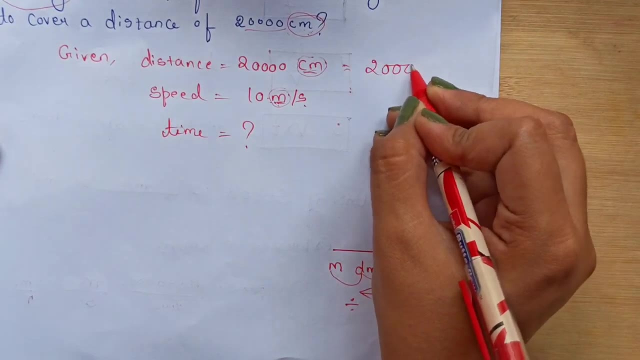 to convert into meters. we have to go like this, from small to big. so I have to go here from small to big, so I have to jump 2 times. whatever number is written, I have to jump. 2 times means how much will I divide? I will divide it by 100. 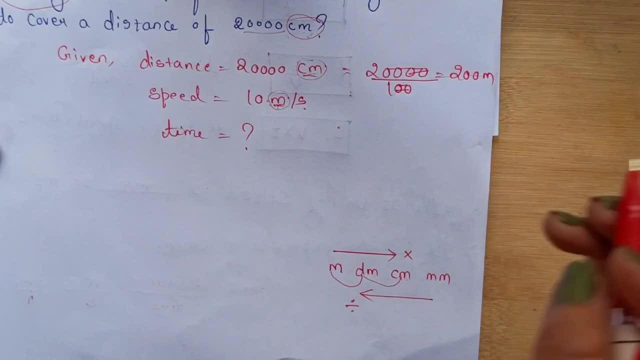 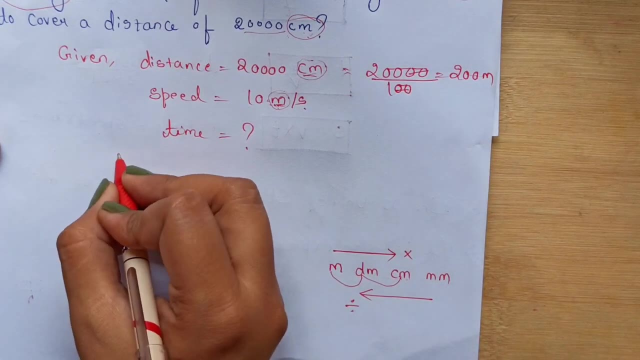 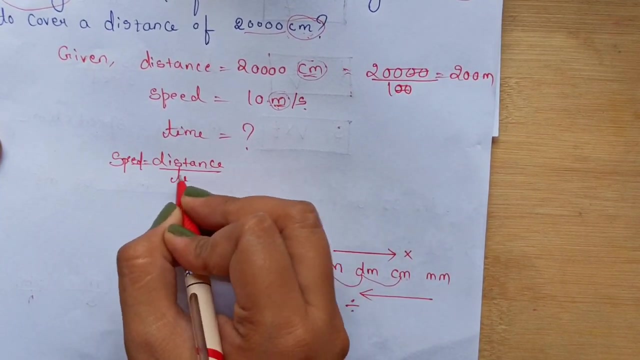 I cut 0 and 0 and the answer is 200 meters. now this also comes in meter. now, what is the formula of time? time is equal to what we know, that speed is equal to distance. this is speed by time. to find time, the formula of time is: 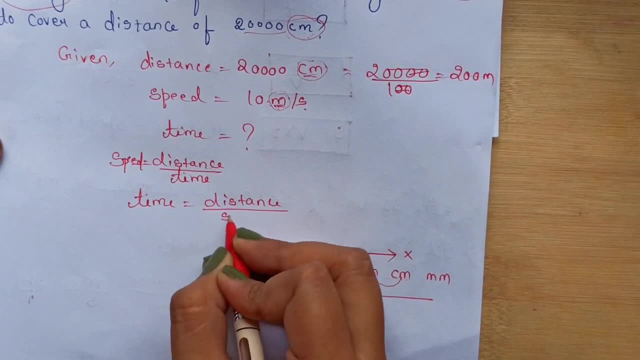 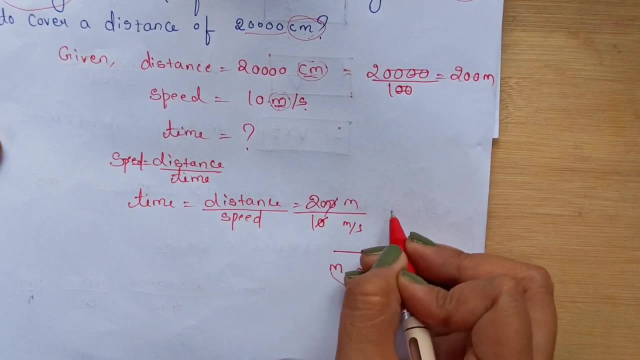 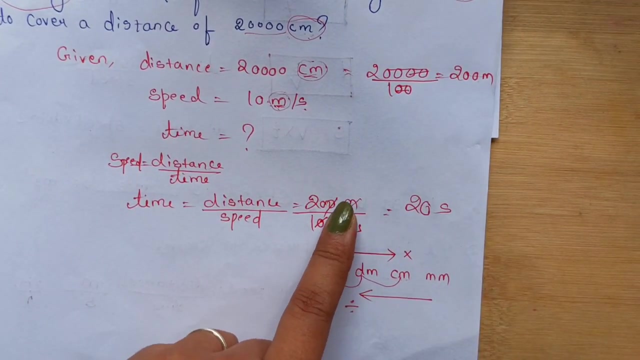 distance by speed. distance by speed. distance is given in meter. 200 meters speed is 10 meters per second. I cut this. the answer is 20 seconds. do one thing: if you get confused here, don't write this unit and time if there is a second in meter. 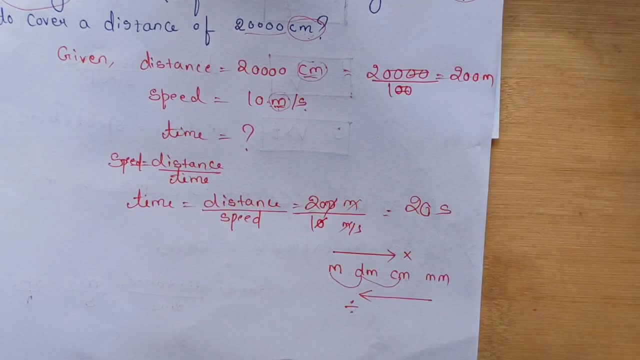 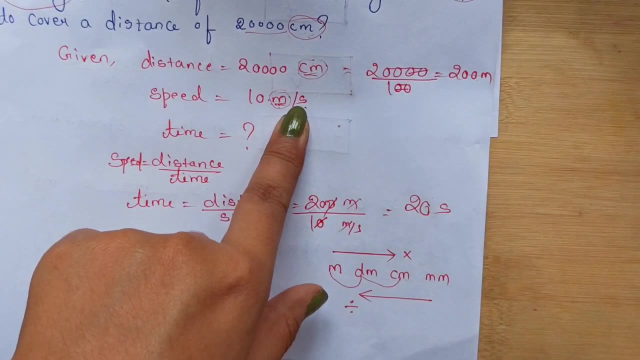 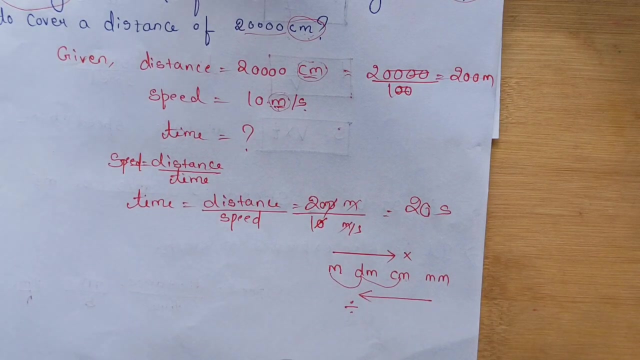 then you can write in time, because in time you don't write meter. in time we write second and hour, but here in question time you can write second. so this was some numericals and many topics of first chapter. first chapter is completed. we have done 1-2 numericals. 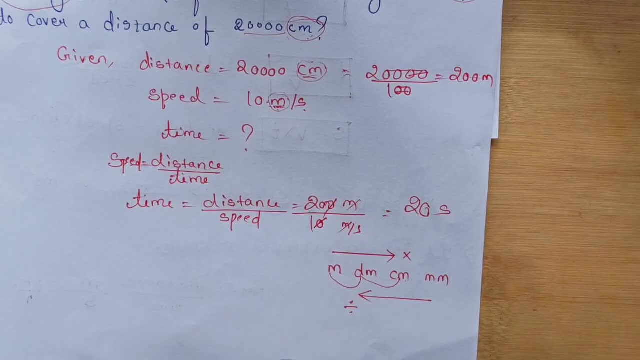 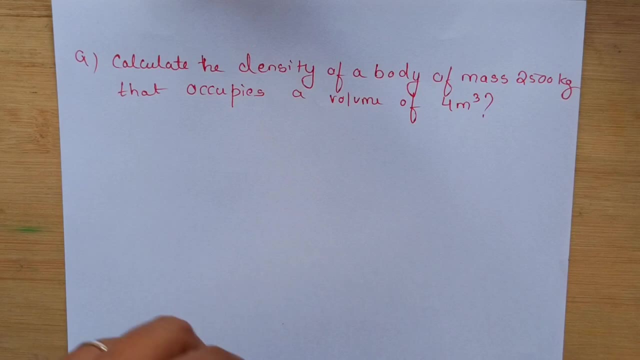 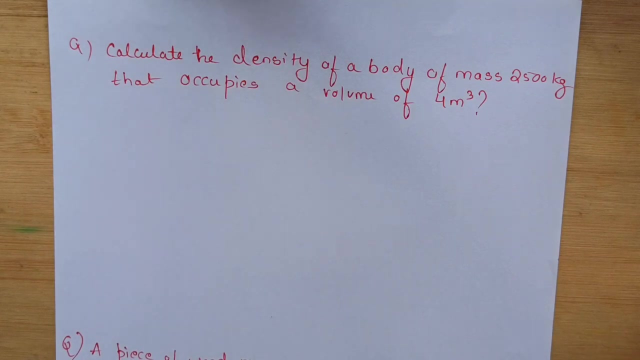 let's see this chapter. after that, this chapter will end. so so this is some numericals on density. see, we have read about density and let's see some numericals. so, as we I told you about speed, by looking at units we can know easily. similarly, let's see this: 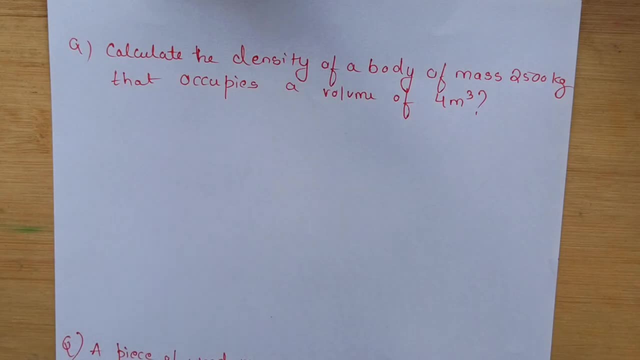 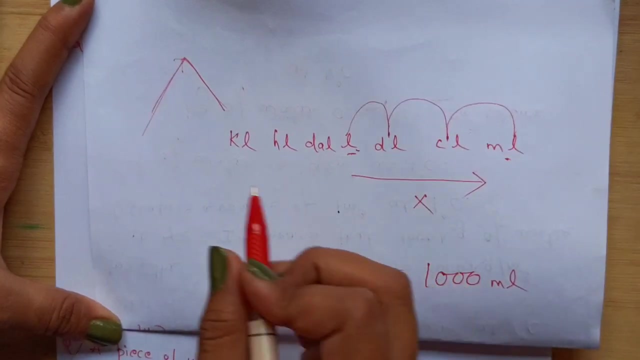 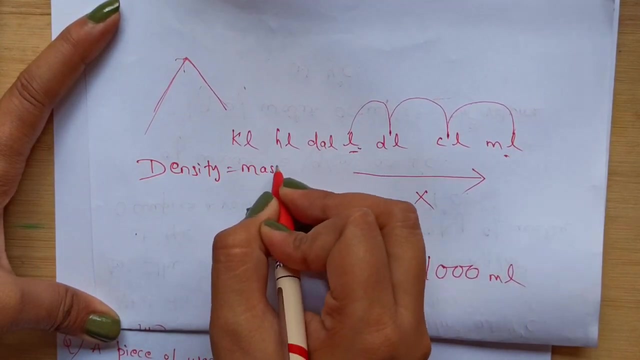 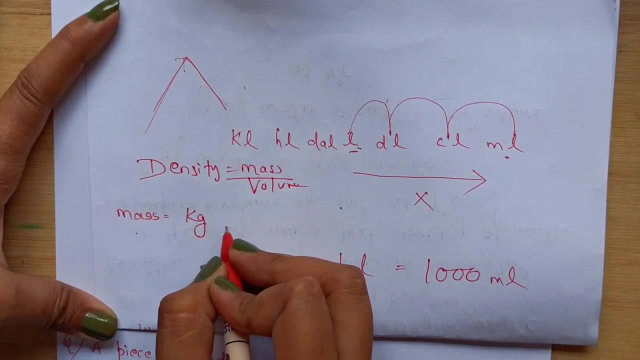 so remember here, as I write here, it will look better, as you can see here, if you first of all I write formula: density is equal to mass by volume. if we talk about mass, if either it will be in kg or it will be in gram, it will be like this: gram, kg, centigram. 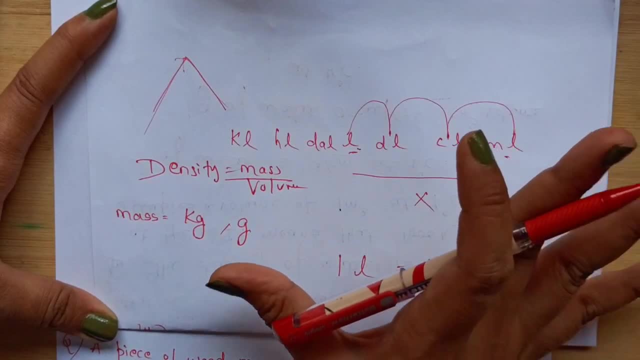 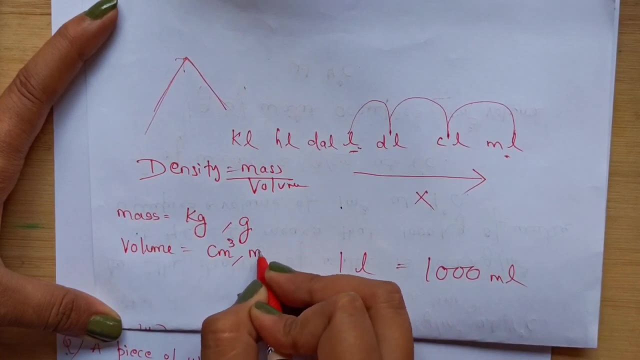 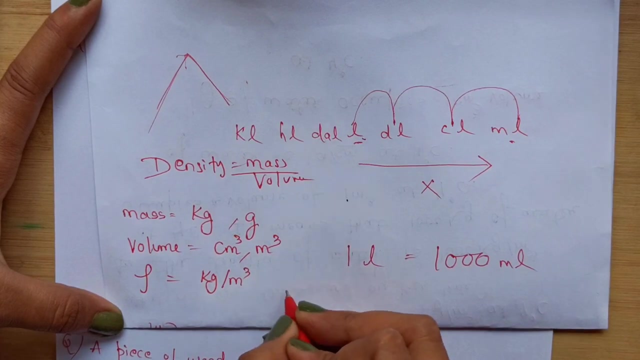 but it will not go that much in centigram and antigram. gram and kg is given like this: if we talk about volume, then volume will be in centigram or in meter cube, and if we talk about density then it will be either in kg per meter cube. 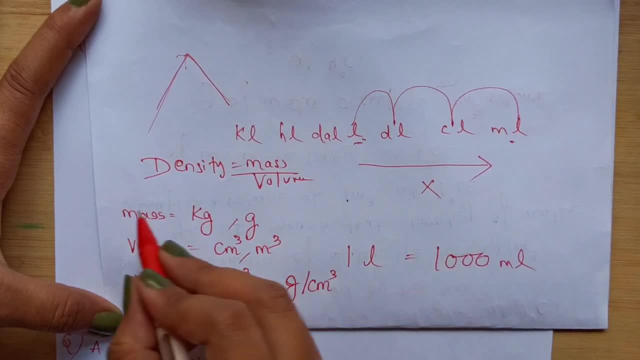 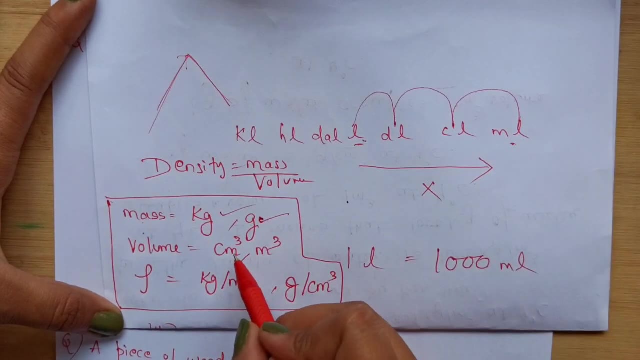 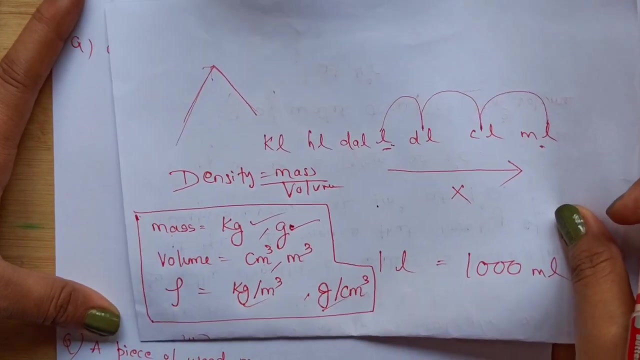 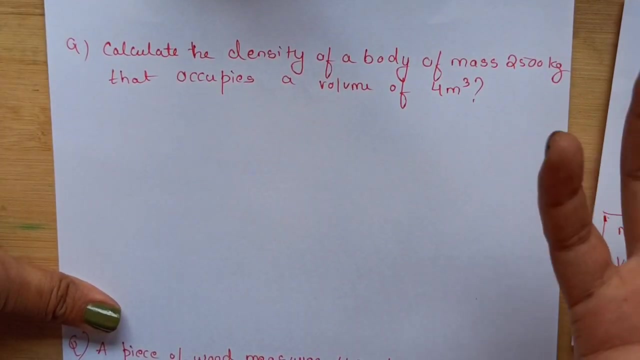 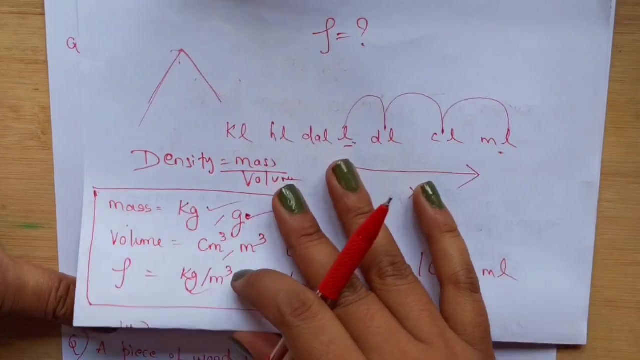 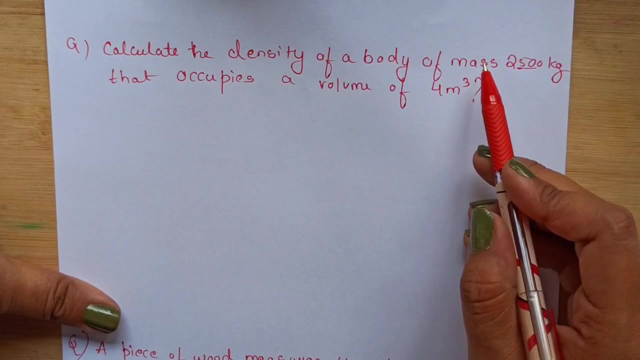 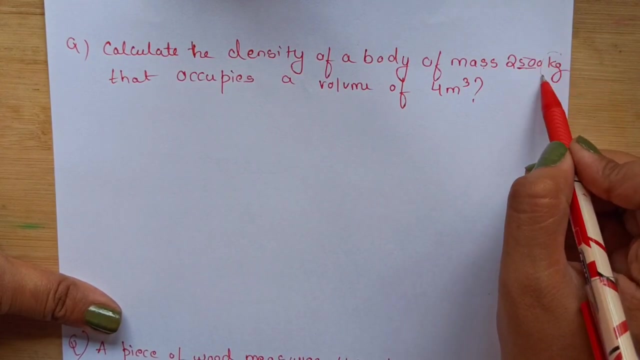 or it will be gram per centigram. remember these 3 things. if you are showing something in gram or kg means have given mass. if you are showing something in centigram or meter, cube means volume. and in all these things, First of all let's do the question. what is said in the question? look, calculate the density of a body. calculate means find out what. to find out, density means we have to take out the density once in the rough. then one of the body whose mass is given is 2500 kg. here it is clear from the direct question that it is talking about mass. but if still no one will understand, look you should come. you have reached 7, so here you have to see this unit. it is given in kg. now you see. 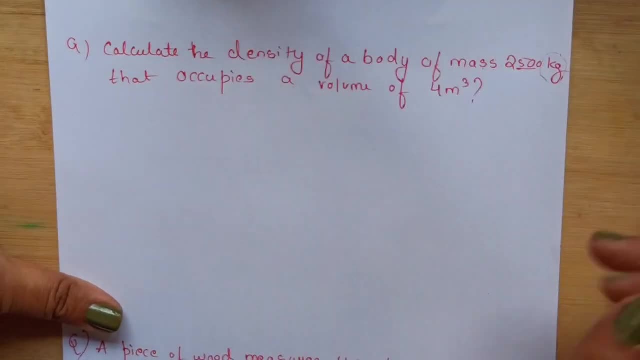 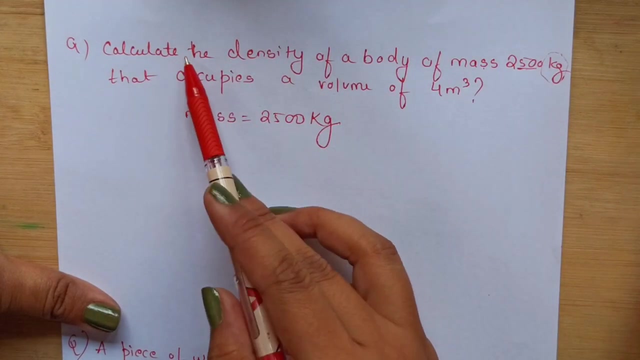 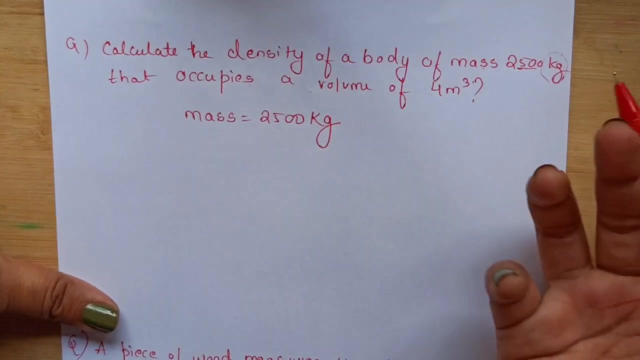 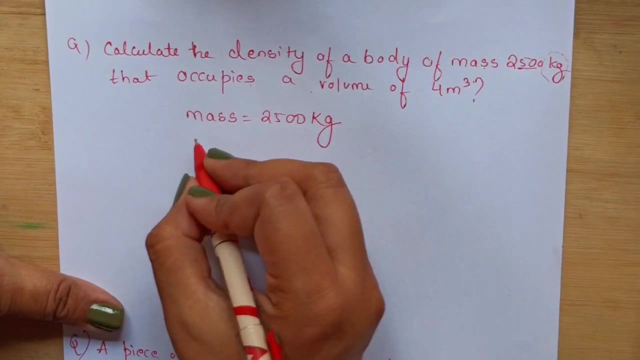 it is given in kg means who is talking about mass. so here, write, write quickly. given mass is equal to 2500 kg, so calculate the density of a body whose mass is this: that occupies a volume of 4 meter per cube. sorry, not per cube, sorry, 4 meter cube. now 1 meter cube is given, so meter cube means who is talking about volume, and here directly we are getting to know. so volume is equal to, so volume. also we have written 4 meter cube. 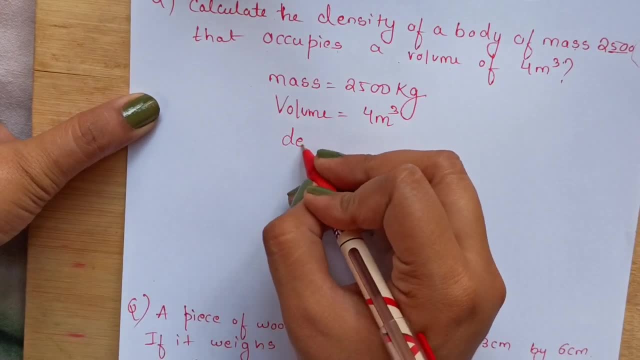 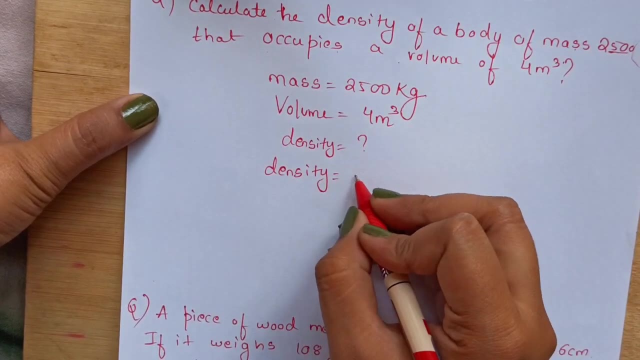 now, what to find out? density. so density is equal to question mark. look, we are doing it the same way like I am doing it. I used to do it the same way now. after that, write the formula: what to find out? so density to find out? so its formula is mass by volume. 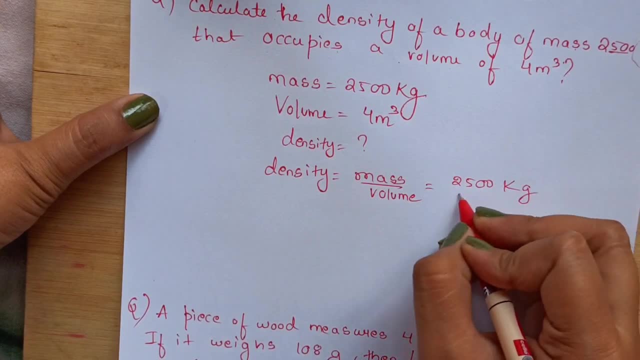 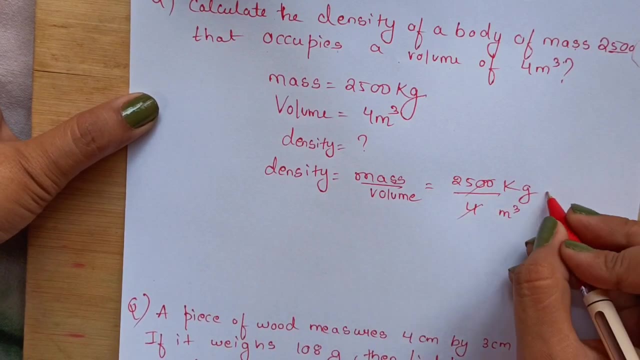 for mass: write 2500 kg. on the side for volume: write 4 meter cube. now divide it. is it going to go from 4 or not? so it will go from 4, it will be our 625,. now just write. 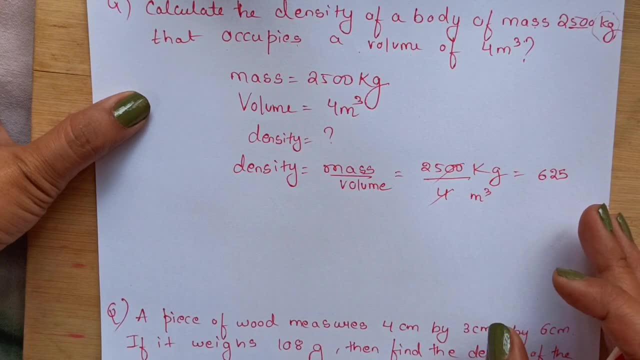 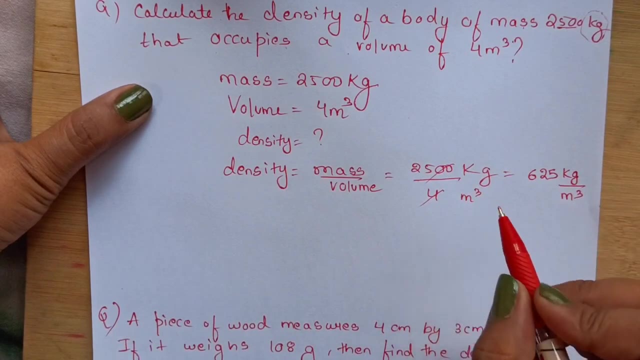 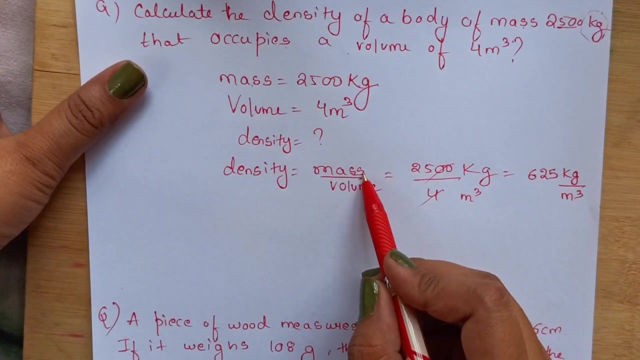 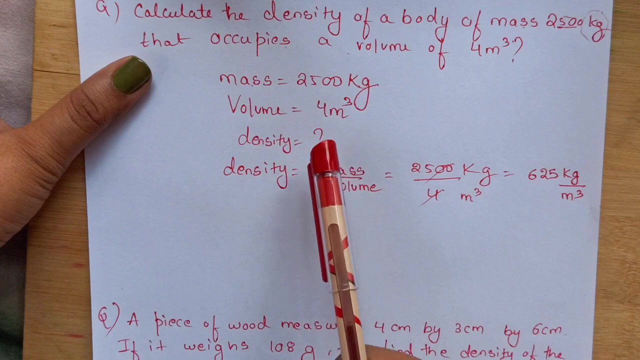 if you write 625, then you will not get marks. we have to write unit also whose density, because we are finding density here above is left kg. so write kg by meter cube. but if you will not understand what to write, then no problem. you see, mass is in kg, write mass above or you will get cube, because I have told you the method, how to find out unit. so if mass is given in kg, then kg is given above. volume is given in meter cube, so below meter per cube, below meter per cube, not below meter per cube, below meter per cube. 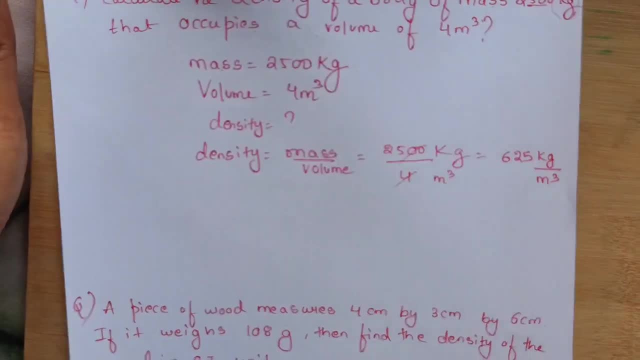 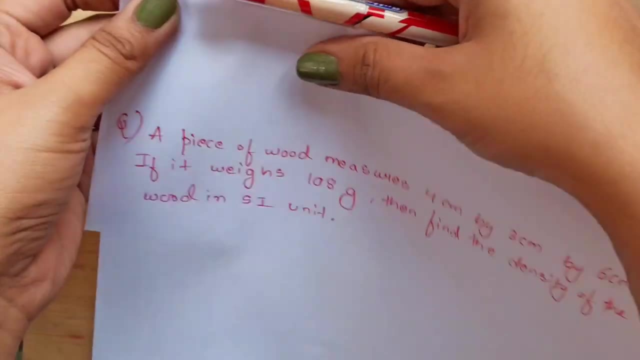 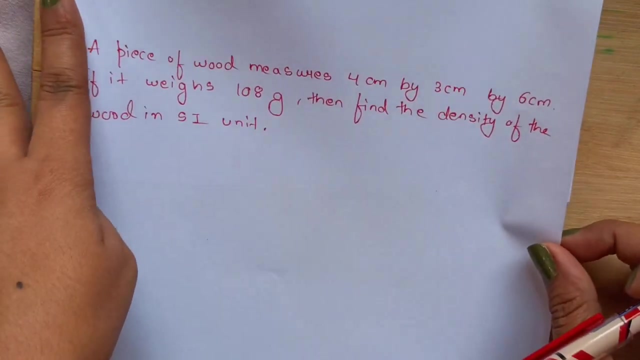 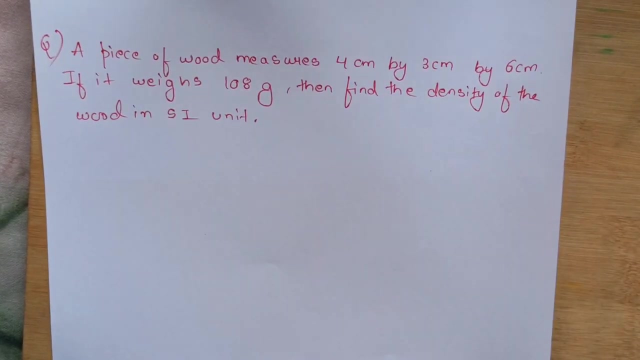 below meter cube, below meter per cube, then this is our density. it's easy, not too much tough, faster. next is, next is, next is: what is it? now we have a question. Let me take another questions. this one is very different because I know many people will start getting distracted by it. 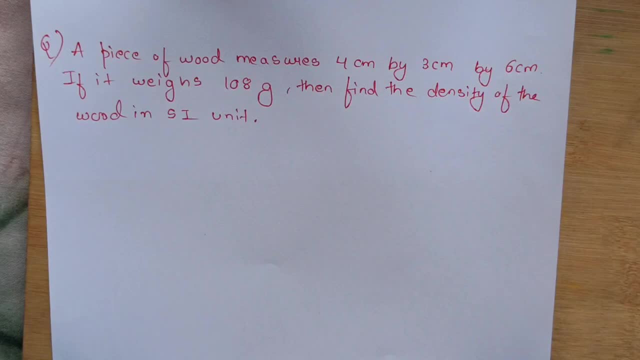 So what is it? the question is about a piece of wood. it is a piece of wood. it measures 4 cm × 3 cm centimeter by six centimeter. Now, what is this? Now, what is this? It is given by by: If it weighs 108 gram. 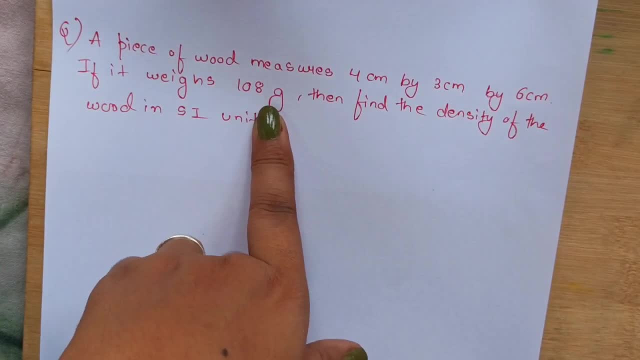 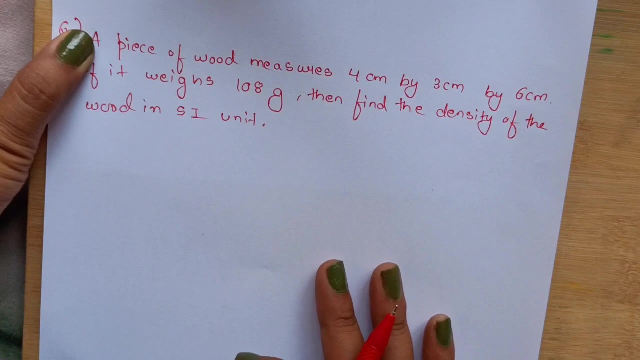 and if its weight- it weighs 108- means 108 gram. If its weight is, then get the density of the wood in SI unit. We will see what SI unit is. we will see. Now see what is said to be taken out: Density and I. 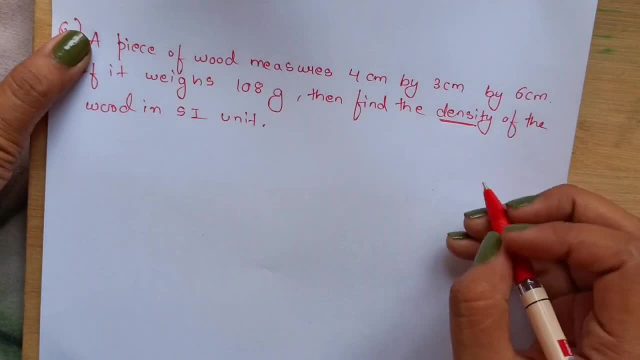 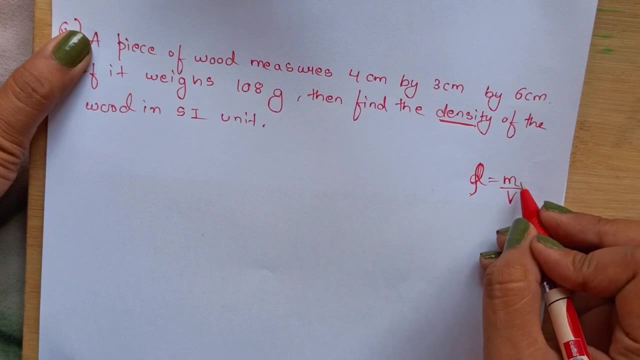 have told you. if density is said to be taken out, then think: what is the formula of density? Mass by volumeinto theinkles I put this row: mass by volume. Now we have read about the mass. what is the mass? 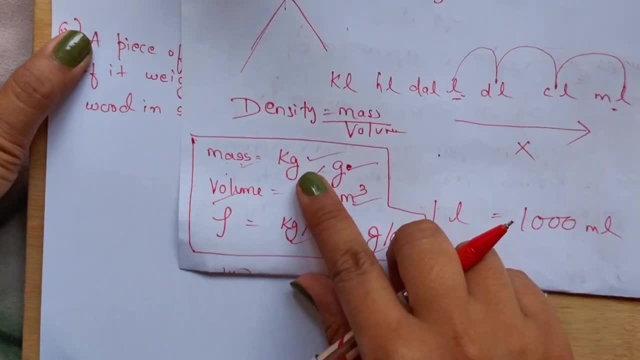 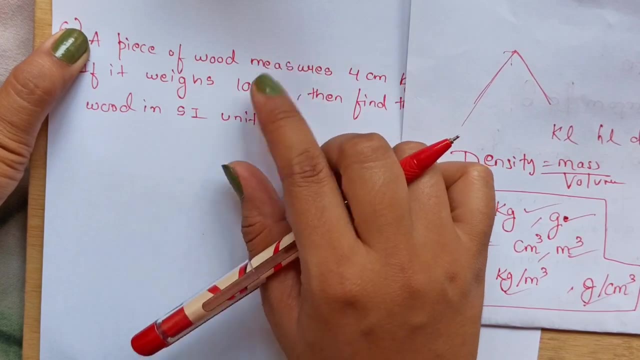 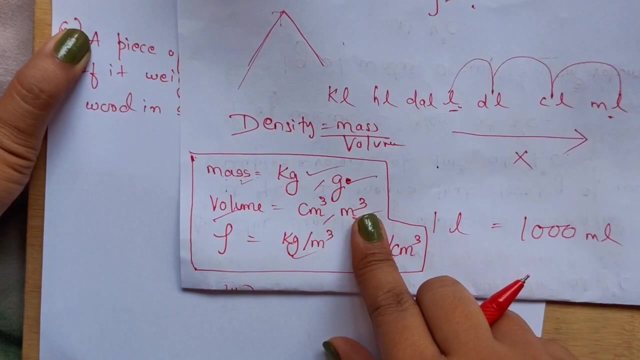 For mass we see in KG and gram, but here it is no given anywhere, but here it is given deliberately. this thing has been given. so this mass, as long as the weight, then our mass in the formula comes in the Chinese also. but what is the value of volume? Theว, Nurse Q, But there is no cube проб system given to the 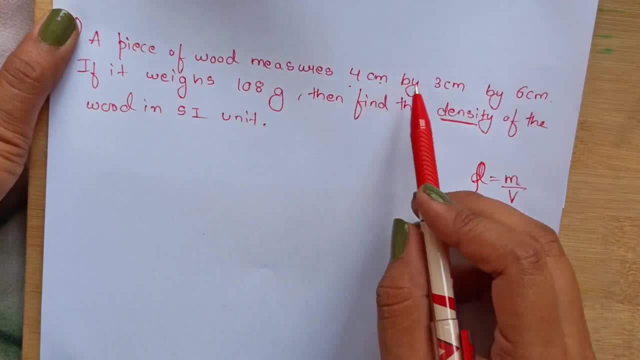 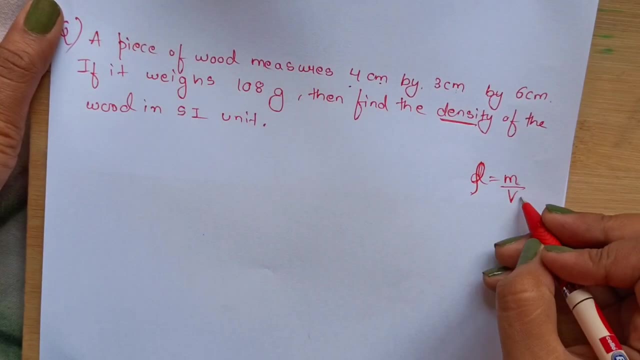 question I But something like this: is given, A piece of wood measures 4 cm by 3 cm by 6 cm. Centimeter is given, but cube is not given. So what will we do? We don't know anything about volume. 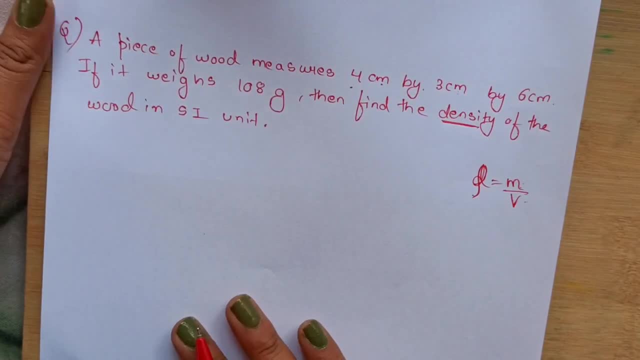 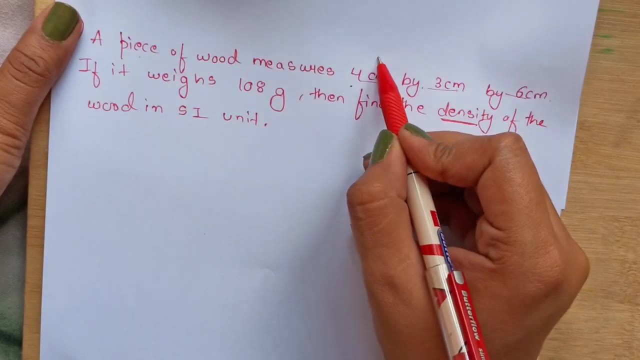 Yes, mass is known, but it is in grams. But for this it is very easy If you have a question from this type. What is written here? A piece of wood which measures this? by this, by this, You must be studying in maths. 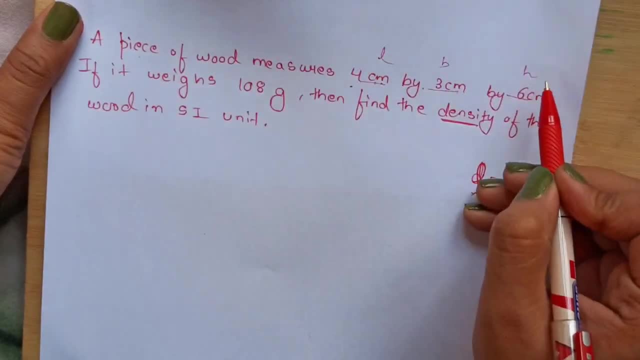 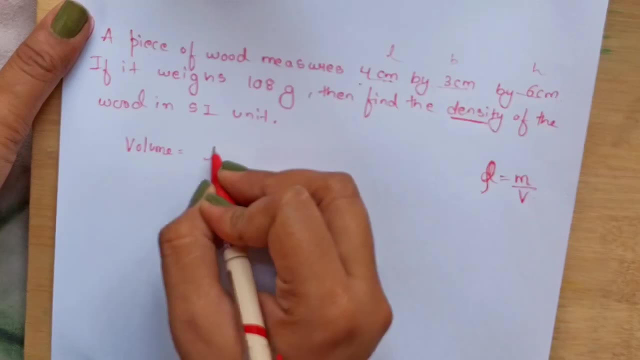 If it is given from this type, then first is length, this is breadth, this is height, Height and volume. of cuboid we had done earlier, So here we can easily calculate volume, Length into breadth, into height. So we will multiply these three. 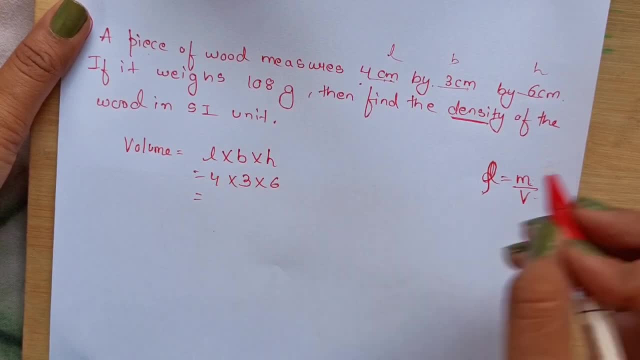 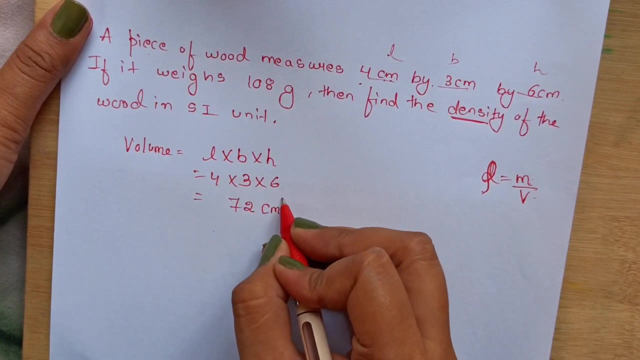 4 cm into 3 cm, into 6.. So how much will this be? 4 x 3 is 12 and 12 x 6 is 72.. What Centimeter cube? Why did I write centimeter cube? Because all three are in centimeter. 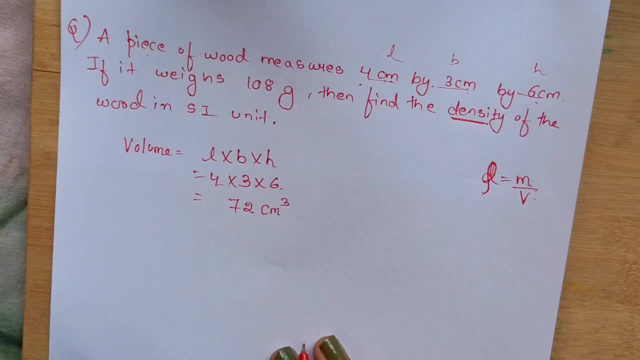 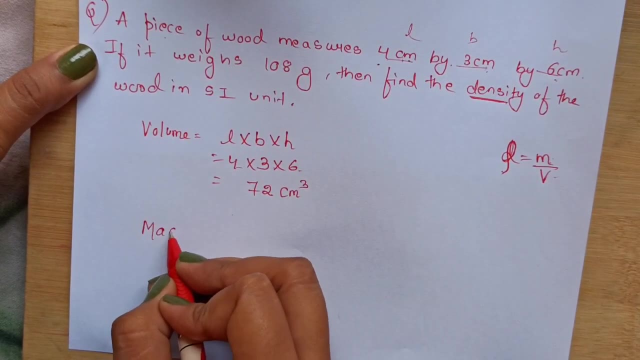 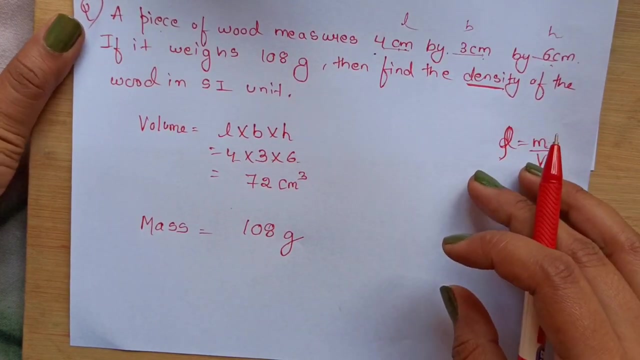 Centimeter, centimeter, centimeter, And we can easily calculate this in centimeter cube. Now, Now, Now what else is given? Second, Weight is given Means. write here mass. once Mass is given 108 grams, But we are being told that whatever density you will get. 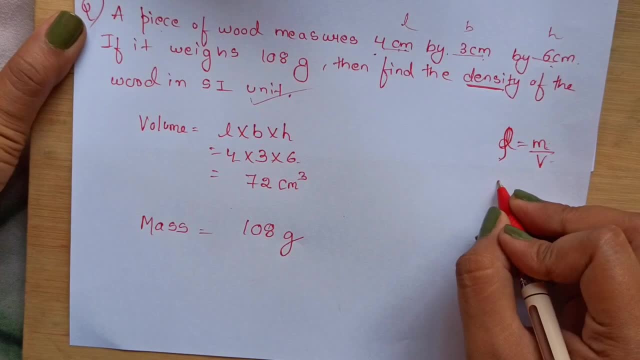 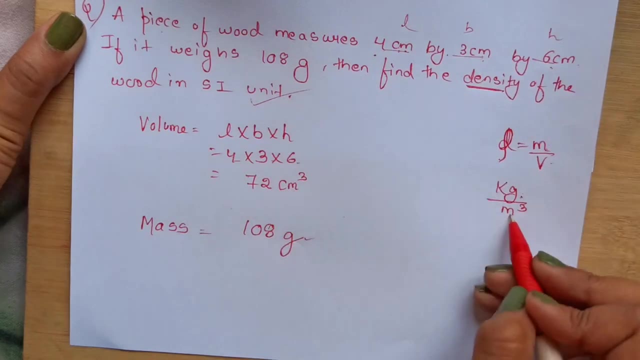 You have to get that in SI unit. In which SI unit? And what is SI unit? Kg by meter cube. So mass should be in kg, but I have it in grams, And volume should be in meter cube, But in which? 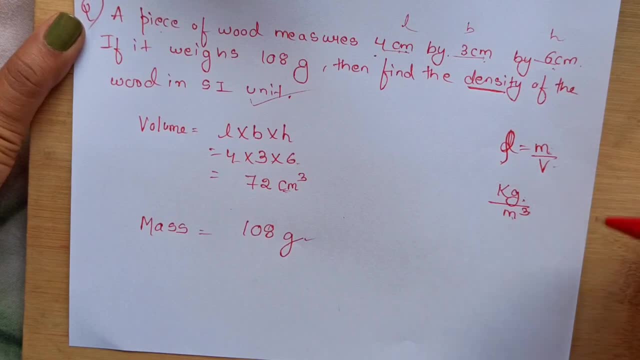 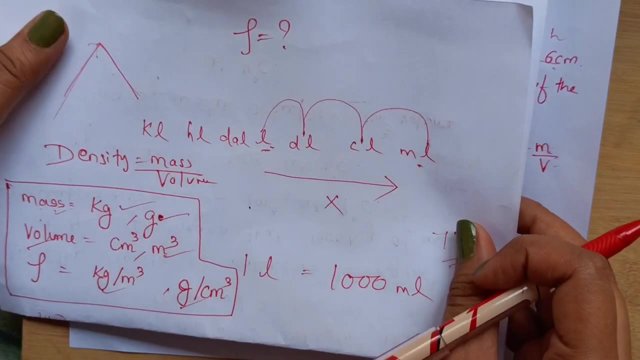 Centimeter cube. So it is okay, So we will convert it Centimeter cube. we have to convert it in meter cube, No problem. Now you remember. I have told you what we have to do: Meter, decimeter, centimeter, millimeter. 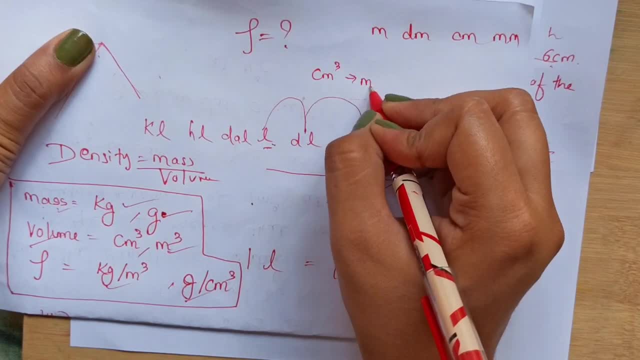 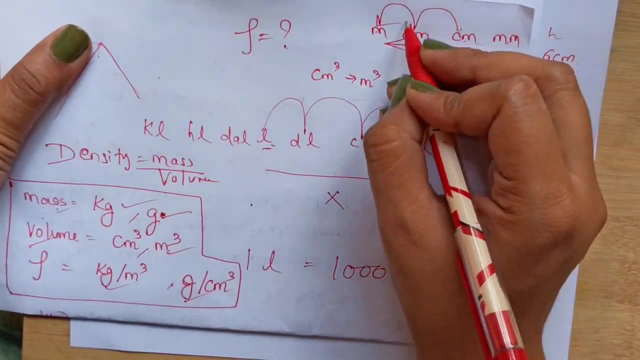 We have to convert the centimeter cube into meter cube Means. it has to go like this: So small to big, We will divide. How much will we divide? How many times will we jump? Jump twice Means divided by 100.. 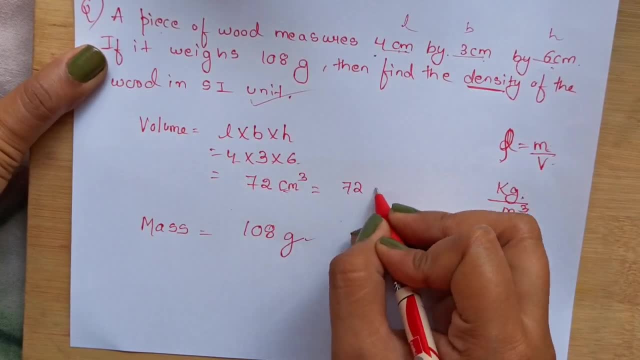 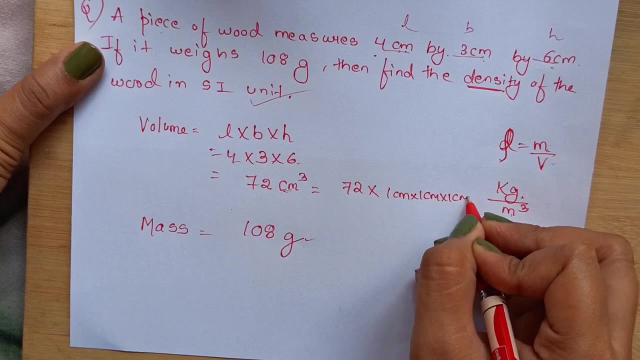 Okay, So here is 72. And with that, how many times is a centimeter? 3 times. So can I write it like this: 1 centimeter into 1 centimeter, into 1 centimeter. Is there any problem in this? 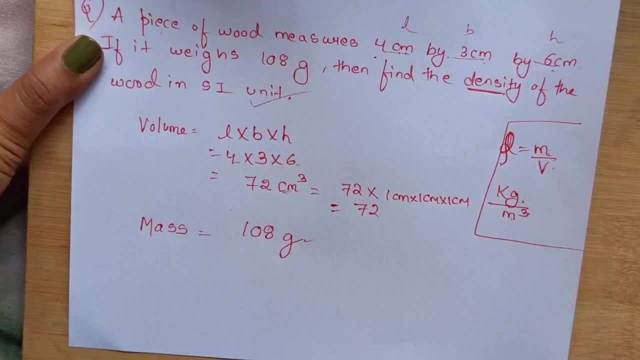 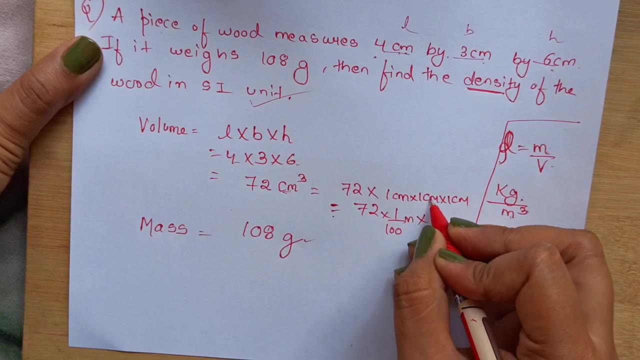 This is a rough work. No, because it is 3 times Now. let 72 be above. Centimeter is 1 time. If I will do 1 time centimeter into meter cube, Then it will be 100 meter. For this, also same 100 meter. 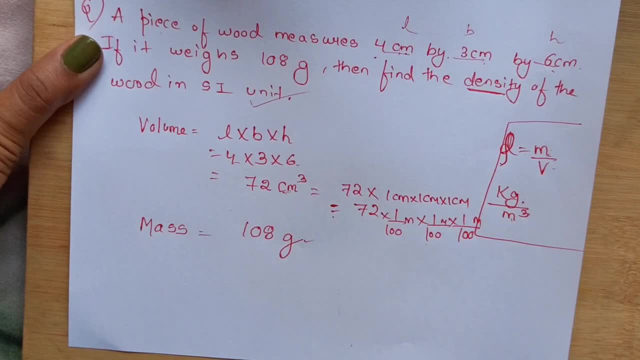 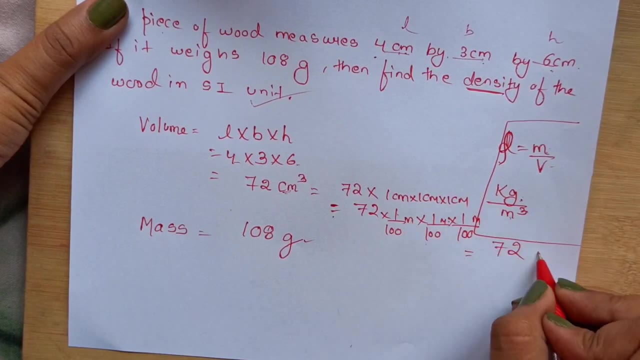 For this also same 100 meter. Now we will solve it, See above: 72 into 1, into 1 into 1.. So this is 72.. 1 meter into 1 meter, into 1 meter, 1 meter cube. 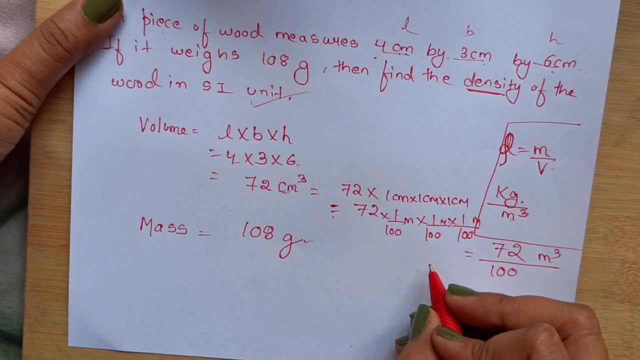 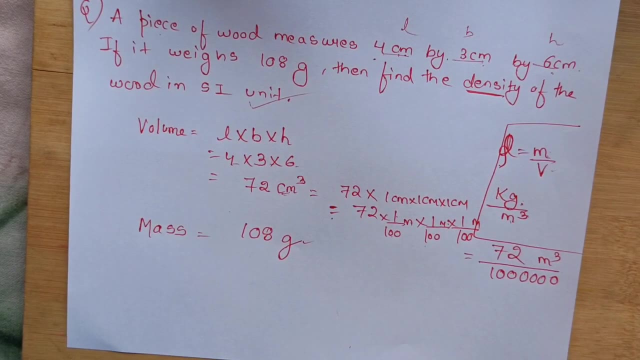 What is below 100 into 100, into 100. So can I write it like this or not? It has converted. It has come to meter cube. It has got a big value, But there is no problem, It comes like this also: 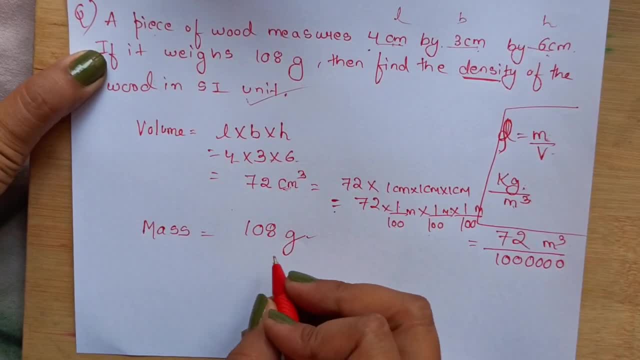 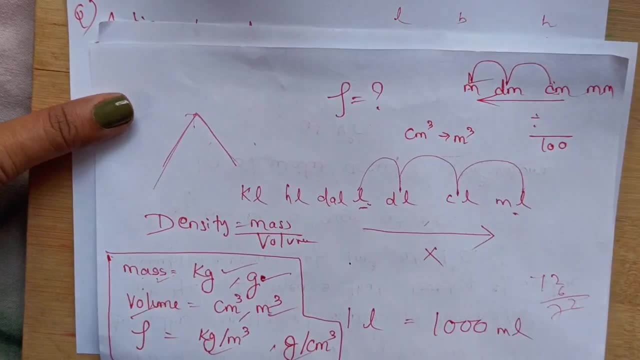 Now next. Now it is the turn of mass. So the mass is given in grams. I have to change this: in what? In kg? Okay, So here again we will see If gram is given here. Here is decagram, Hectogram. 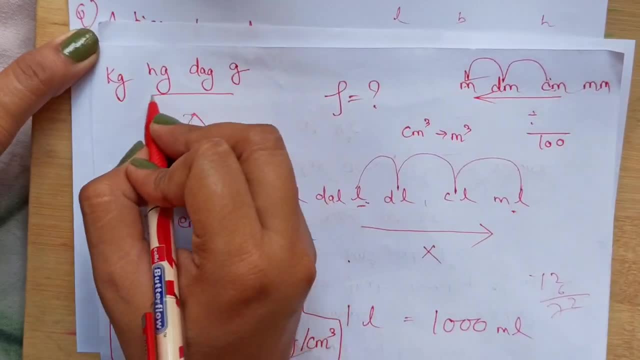 And here it is given as kilogram. Here also I have to go from gram to kg. If it is big or small, then divide. How many times am I jumping? 1, 2, 3 means I have to divide 1000.. 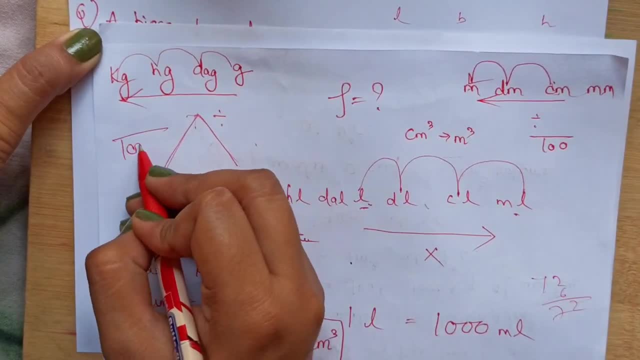 And you must know that To convert from gram to kg, Whatever number it gives, We just divide it by 1000. So this is done. Now we have volume also come in meter. cube Mass also come in kg Means. in such a unit the density can come. 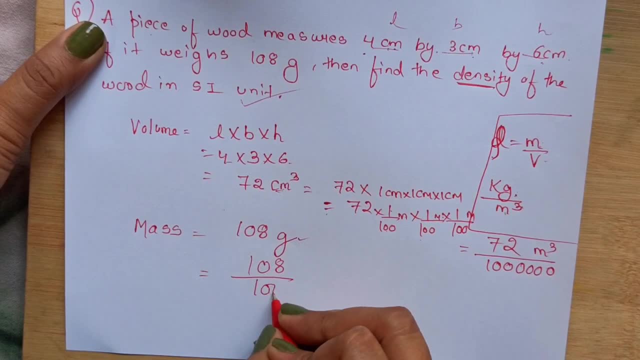 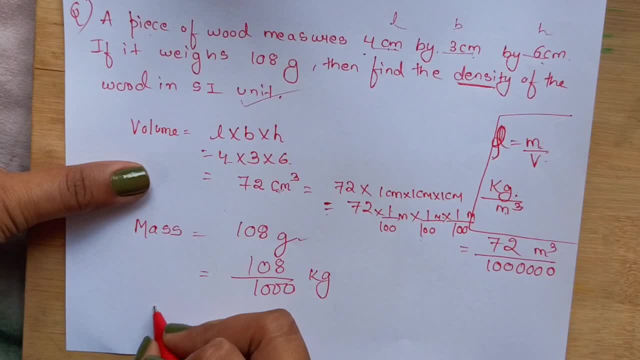 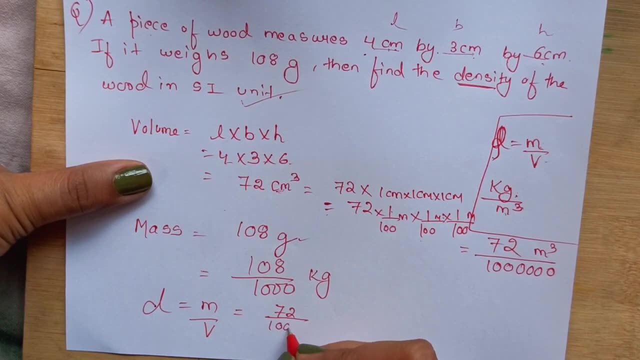 1 meter cube. 1 meter cube, 1 meter cube. So density is equal to mass by volume. instead of mass, write 72 by 1,, 2,, 3,, 4,, 5,, 6,. write this: 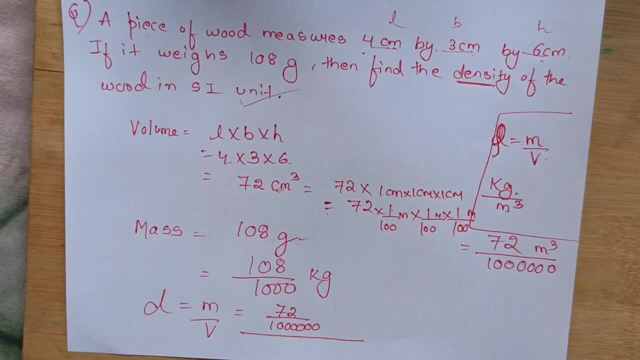 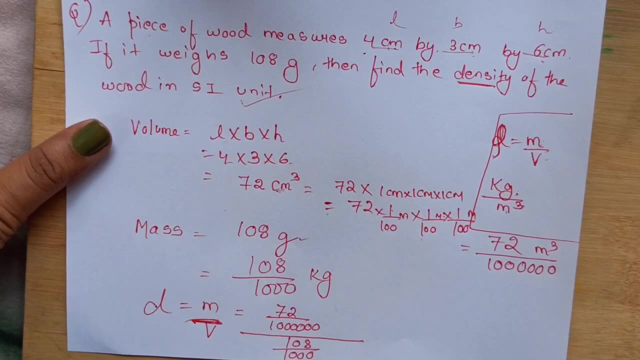 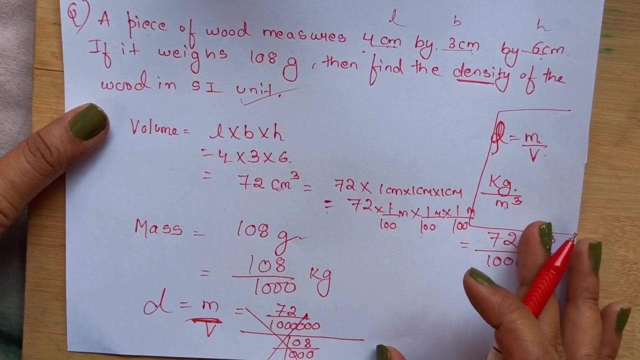 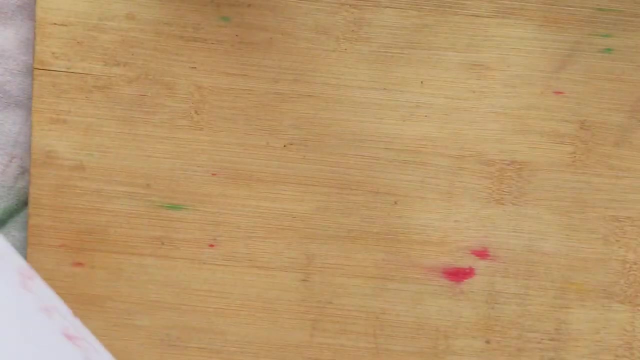 Now make the divided by a little longer. This is the divided by: make it a little longer. What is the volume? 108 by 1000.. Now I will write it upside down. Now I will write it on a new page. 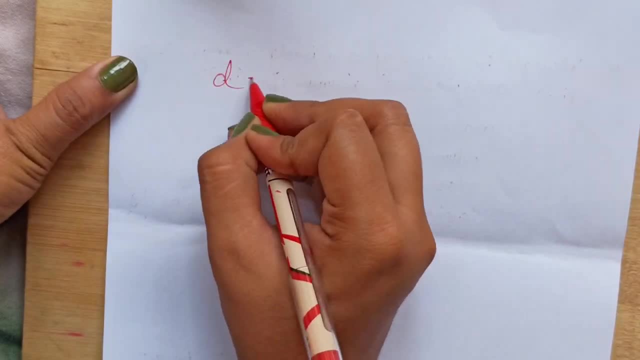 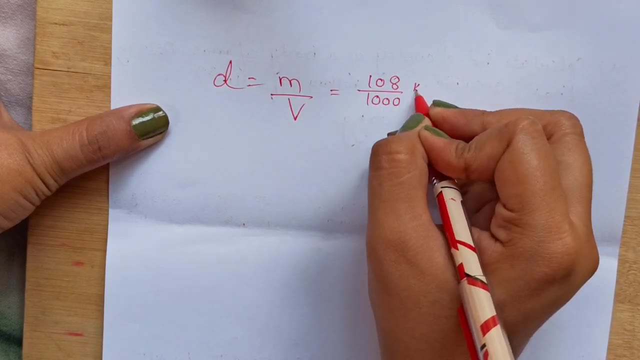 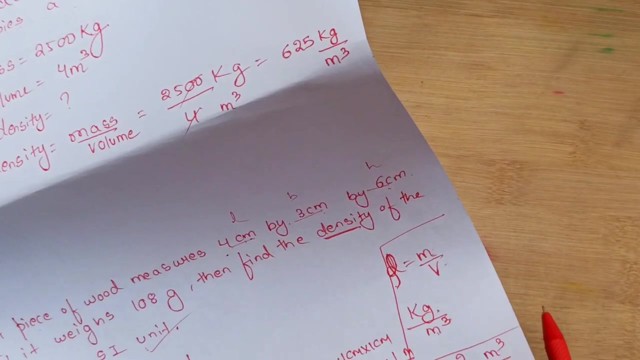 Now I have to find the density. So what is the formula to find the density? Mass by volume. What did we find? the mass: 108 by 1000 kg Whole divided by what is the volume? What is the volume? 72.. 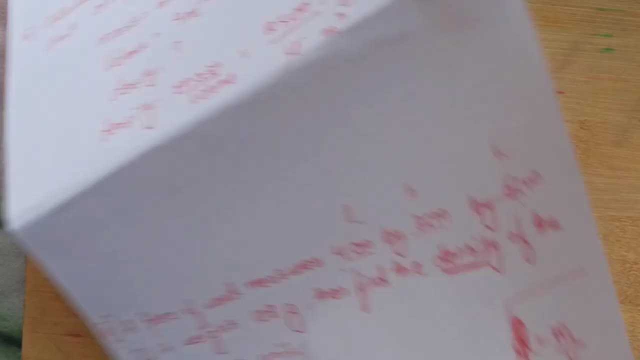 How much did we find? 72 by 1,, 0,, 1,, 2,, 3,, 4,, 5, 6.. I will write it: 72 by 1,, 2,, 3,, 4,, 5,, 6, meter cube. 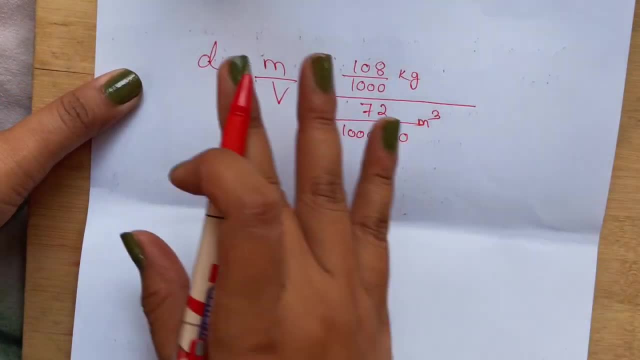 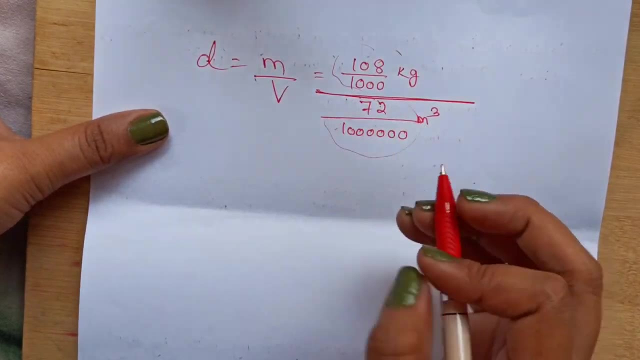 This is done. Now we will solve this very easily. Now, see, I will make the divided by a little longer, Because there is a fraction at the top and there is a fraction at the bottom. Now, forget these two. 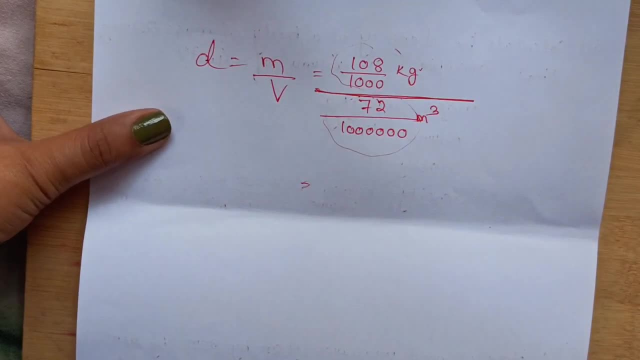 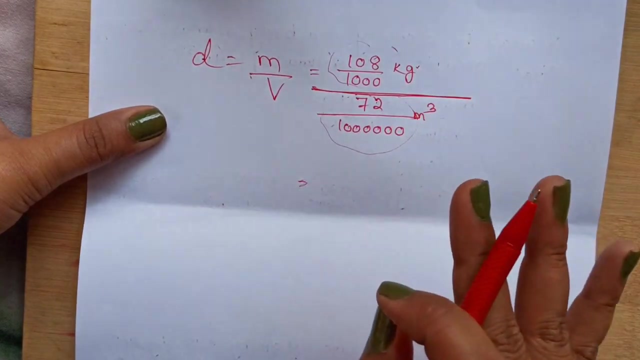 So remember that, whatever the answer is, we have to put the meter cube in kg. Now see the number at the top. We can solve the problem with this kind of a number. Whatever the number at the top, there is no problem. 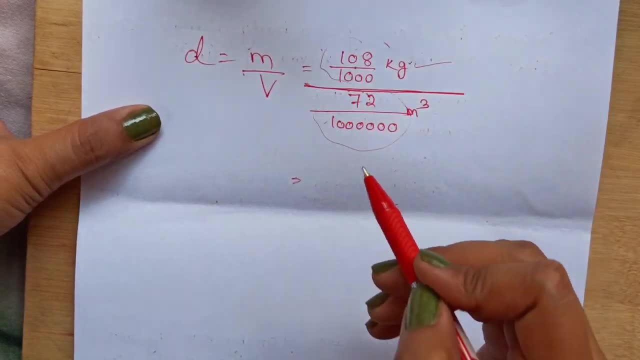 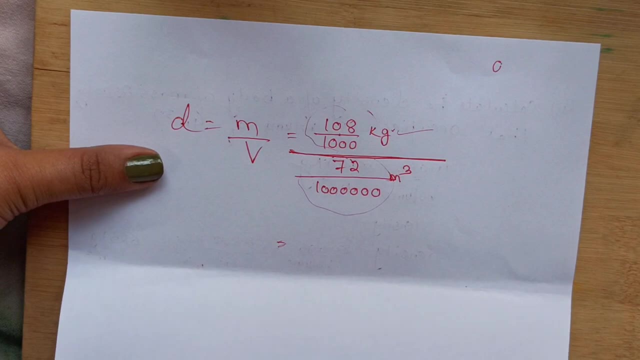 We can do it easily: Fraction at the top and fraction at the bottom. If no one knows fraction, then fraction means that if the number is of this kind, Let me show it here: If the number is of this kind, a by b, 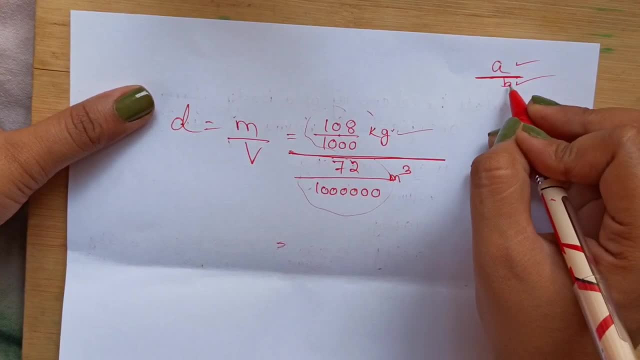 There is a number at the top and at the bottom. There is a number at the middle divided by. But the number at the bottom should not be equal to zero. Zero should not be at the bottom. Now let's do it here. 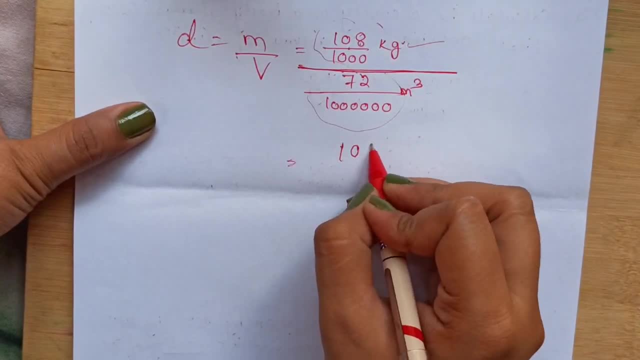 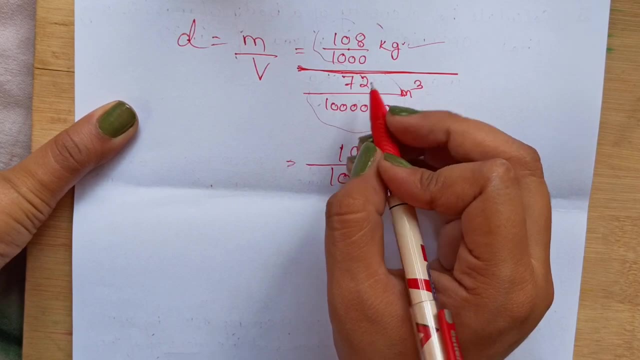 There is a fraction at the top and a fraction at the bottom. No problem, Write down the one at the top, Whatever it is. Now, if there is a fraction at the bottom after y, then what will we do? This is in the divided form at the bottom. 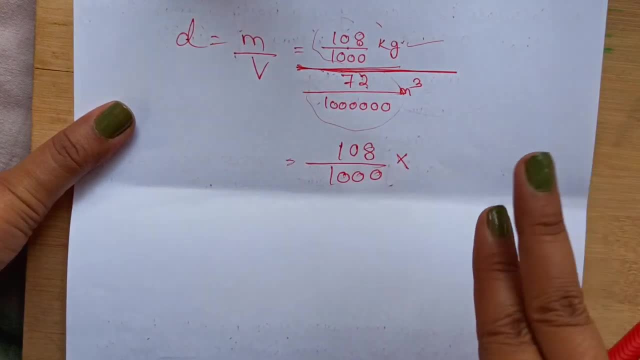 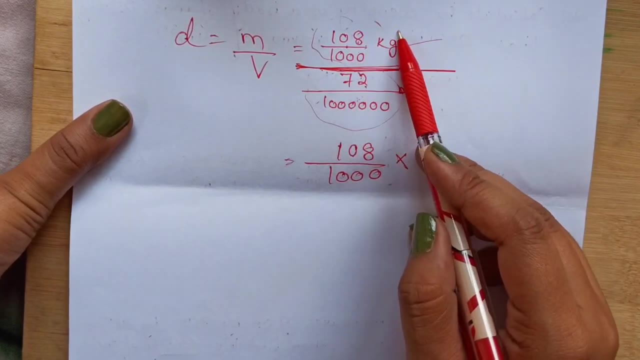 Here we will do into and this one at the bottom will come up. But this will be reciprocal, it will be upside down. What I am saying is, if we get to solve this type of problem, there is a fraction at the top and a fraction at the bottom. 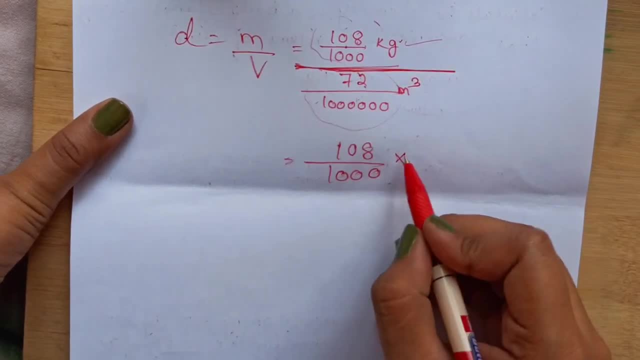 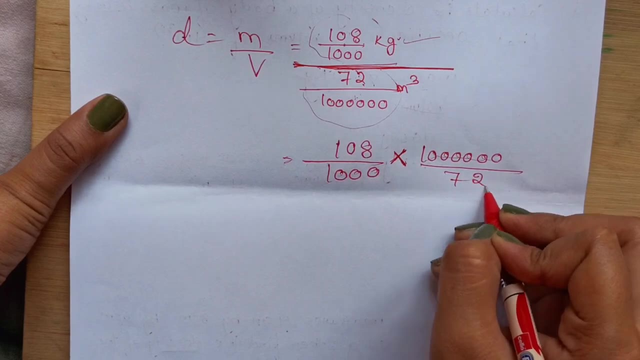 Write down the one at the top. How will we solve the one at the bottom? Write down the one at the bottom and this one at the bottom will be reciprocal. Reciprocal means it will be upside down, So we will get this type of problem. 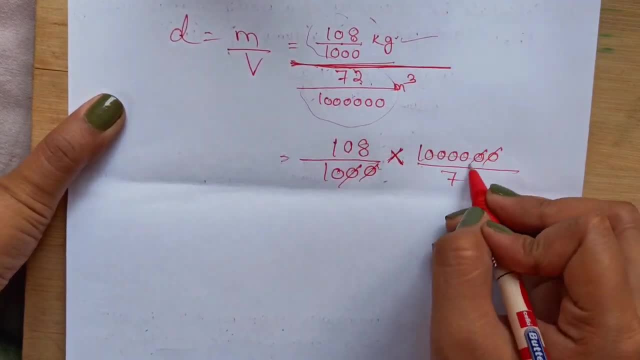 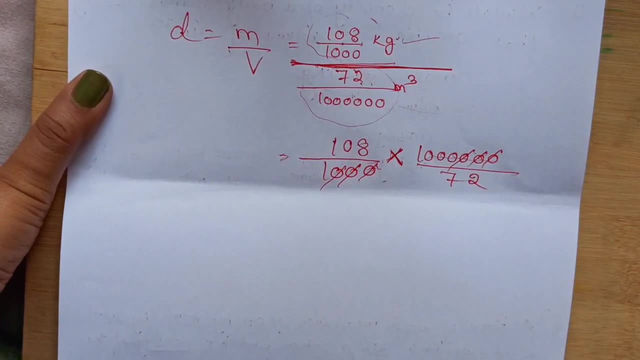 Ok, Now here we have 1010, 1010, 1010, 1010.. Now 72 is left here and 108 is left here. Now we can easily cut 72 and 108.. How can we cut it?